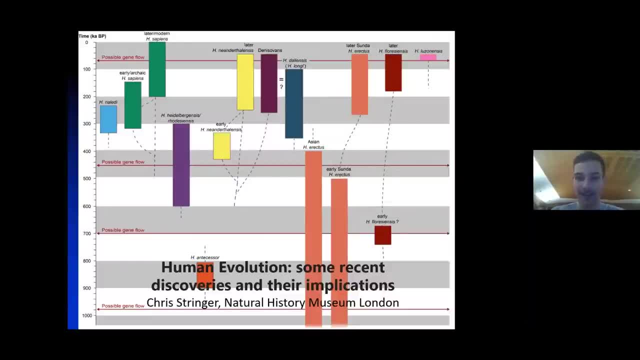 And he has excavated at sites in Britain and abroad, directed the Ancient Human Occupation of Britain project from 2001 to 2013.. And he has published over 250 scientific papers, And his recent books include Complete World of Human Evolution, The Origin of Our Species and Britain: One Million Years of Human Story. 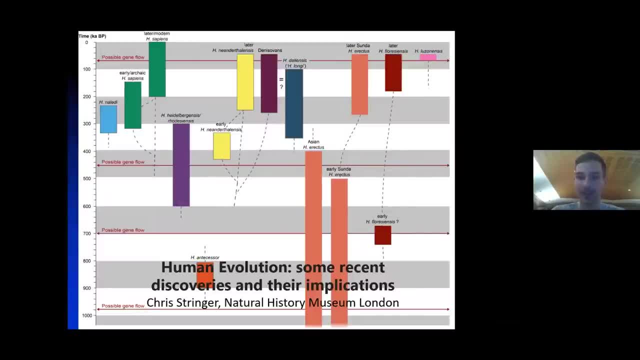 So there are plenty of publications and scientific papers on human evolutions, And Chris will be giving us updates on human evolution from his perspective and from the newest research he has done today. So I'm leaving this virtual stage to you now, Chris. Okay, thank you very much. 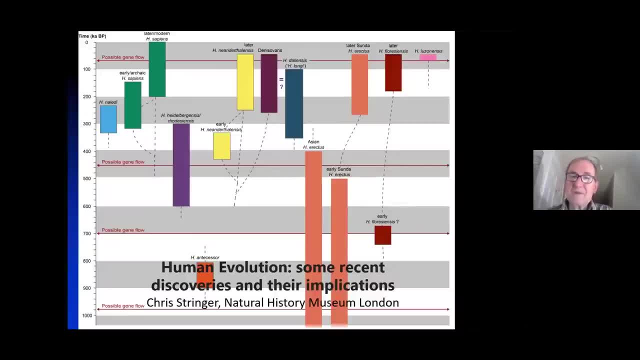 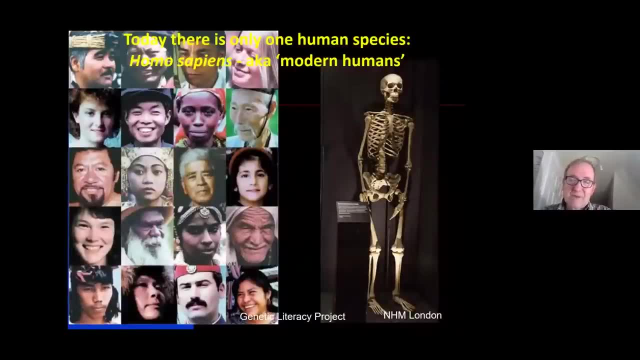 Yeah, so human evolution, some recent discoveries and their implications And, of course, you know some basic groundwork, that everyone around today, of course, is a member of this species. We call ourselves Homo sapiens. wise humans May not be such a good name, but that's the name we've got. 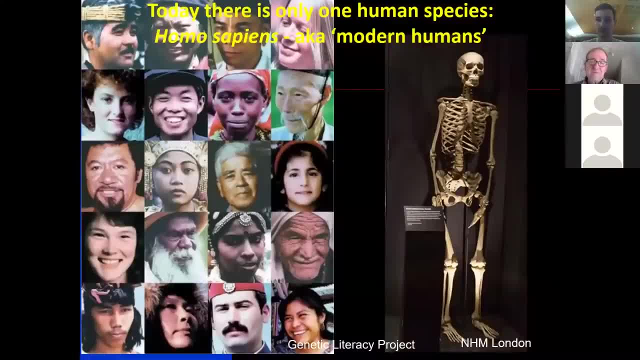 And of course, if we look around the world, there's a lot of diversity. People come in many different sizes, shapes and colors, But genetically we are all closely related and we belong to this one species. And when we take away the superficial features and get down to the skeleton, we also have shared features in our skeletons. 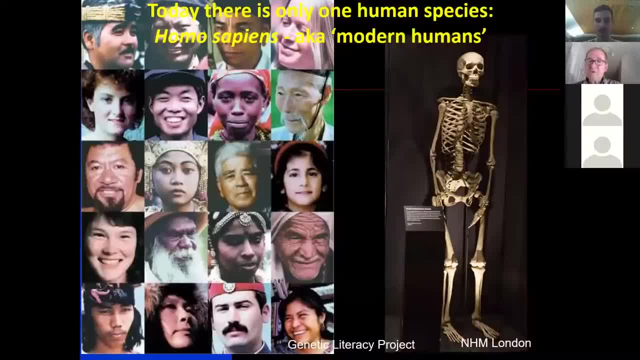 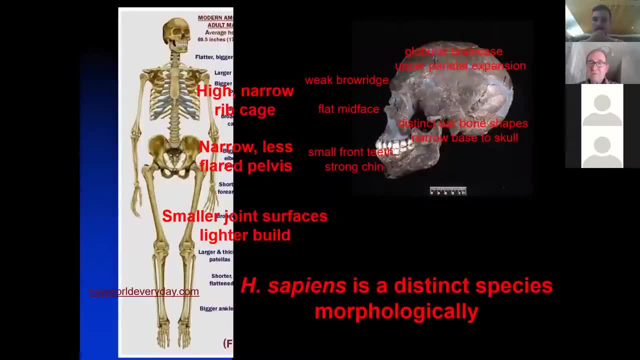 And on the right hand side there you can see a modern human skeleton from the exhibition at the Natural History Museum in London, And when we look at that skeleton we can see a number of derived features that are special to our species. So in the skeleton as a whole we've got a high, narrow rib cage. 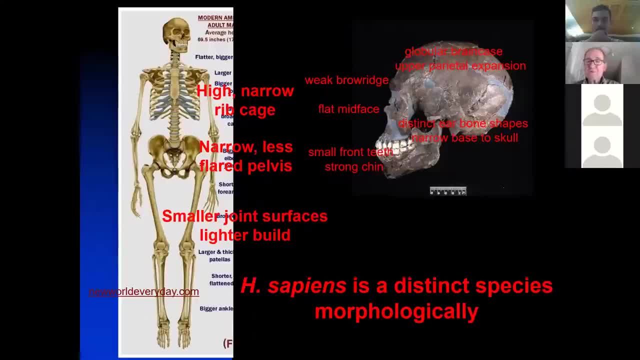 We've got a narrow, less flared pelvis compared with earlier humans. We've got smaller joint surfaces, a lighter build to the skeleton. Generally the muscle markings are not so strong as we find in earlier human species, And that goes for the skull as well. 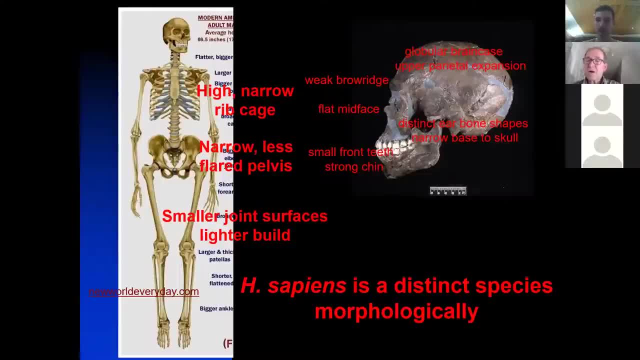 We have a number of differences there. So we've got this high and rounded globular brain case. The upper parietal region is expanded out. The base of the skull is narrow. We have distinct ear bone shapes compared with other humans. We have a weak or non-existent brow ridge at the front of the brain case. 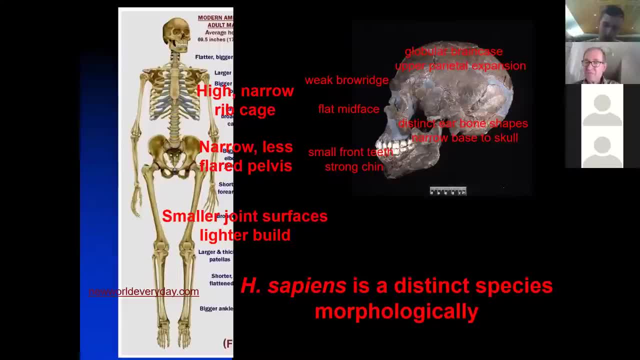 The face is flat, transversely flat, and retracted under the brain case. We have relatively small front teeth and we have a chin on the lower jaw. So these are all features we can look for in fossils to track back when Homo sapiens originated. 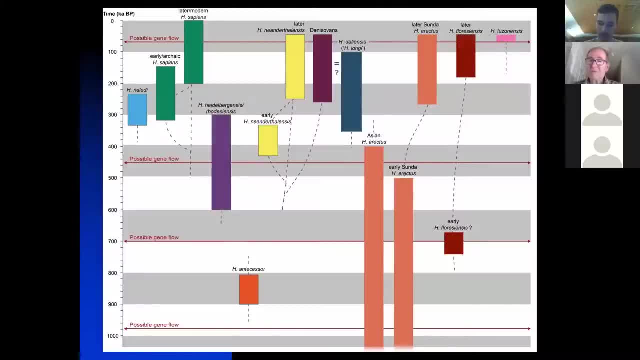 But there was a lot of diversity in the past And this is my attempt to map that diversity. So these bars in this diagram represent different lineages. I would call most of them different species of human during the last one million years. And we're over there on the top left, the green bar, Homo sapiens. 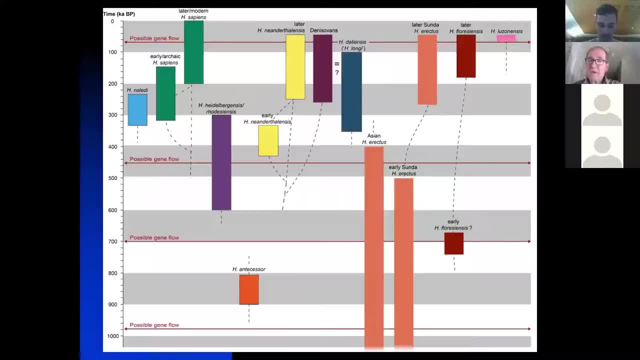 We've got the yellow bar, the Neanderthals and another lot, But I'll be talking about the Denisovans in the center there. So there's all this diversity, And even recently there were a number of different humans around. 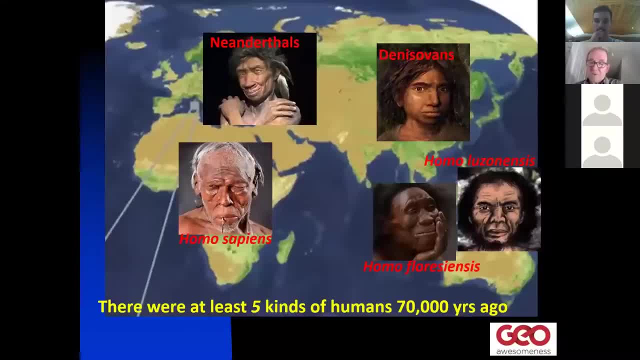 So even 70,000 years ago, of course, geologically like yesterday, there were at least five kinds of humans around. We had been evolving in Africa. Homo sapiens, The Neanderthals, had been evolving in Europe and Asia. 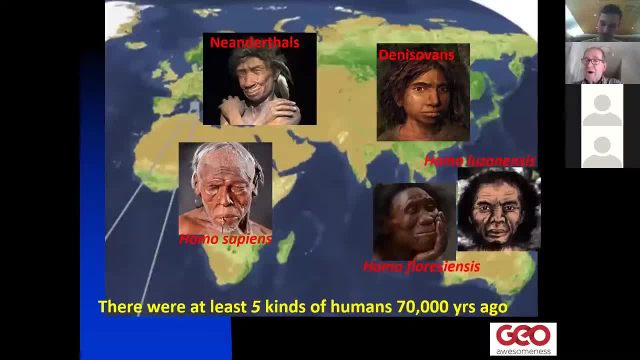 The Denisovans over in East Asia And down in Ireland, Southeast Asia, we had these strange small bodied species of human and small brain species of human on Flores, Homo floresiensis, nicknamed the Hobbit, And in the Philippines, Homo luzonensis, a species only named in the last couple of years. 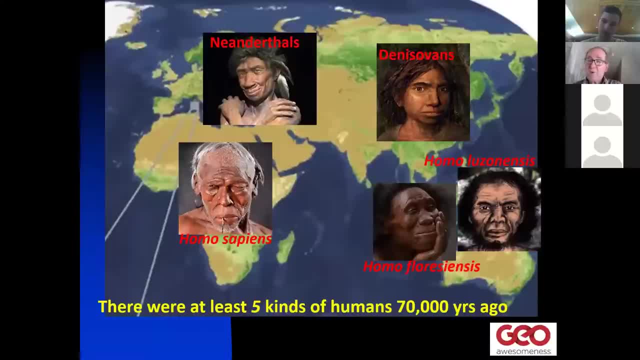 So even 70,000 years ago there was still all this diversity, And Homo erectus, the more ancient species, might even still have been around as well. That's not so well mapped, So I'm going to talk about four things, if there's time in the talk. 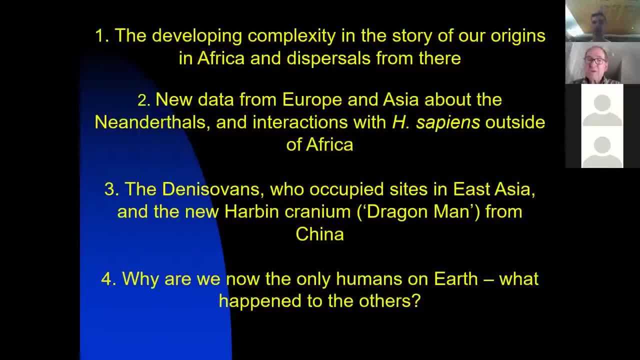 Talk about the situation in Africa and our origins there, Talk about Neanderthals in Europe and Asia and our interactions with them, Talk about the Denisovans in East Asia, And then, finally, that big question, which, of course, is very interesting for archaeologists too. 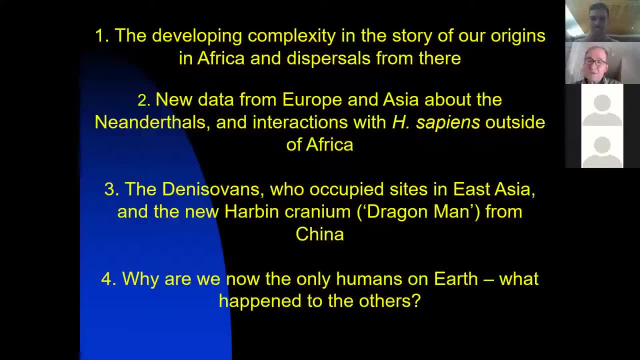 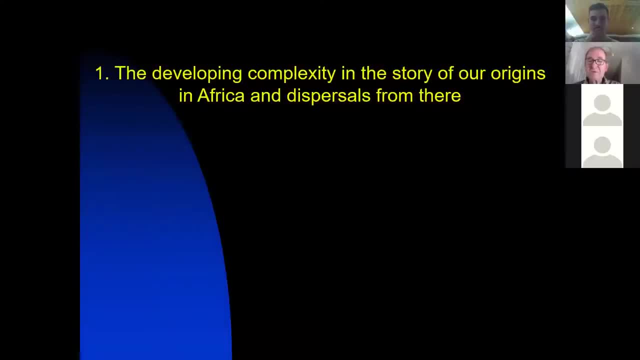 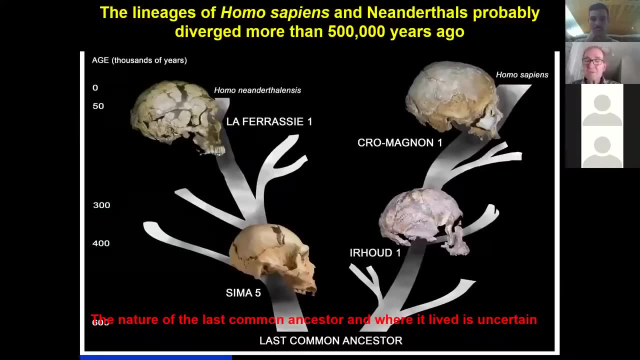 Why are we the only humans on Earth? What happened to those other species that were around until recently? So let's look at the African story briefly, And here's a simple representation of the evolution of the Neanderthal and Homo sapiensis. So on the left, there we've got the Neanderthal lineage stretching for several hundred thousand years in Europe and Asia. 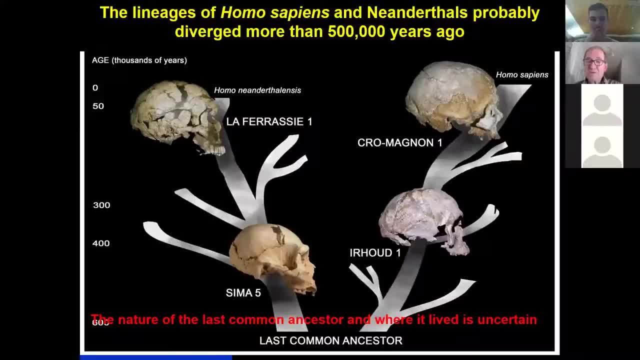 And we've got this fossil from the Cima del Huesos in Spain, about 430,000 years old and showing what seemed to be clear early Neanderthal features. So the Neanderthal lineage goes deep in time And in Africa we can trace our own lineage back over a similar length of time. 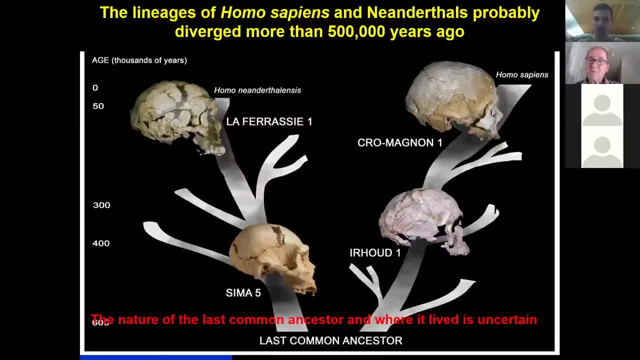 We've got a Homo sapiens fossil on the top right there from Cro-Manual In France, But lower down there, the Jibbel Ehud 1 fossil from Morocco seems to be an early Homo sapiens at around 300,000 years ago. 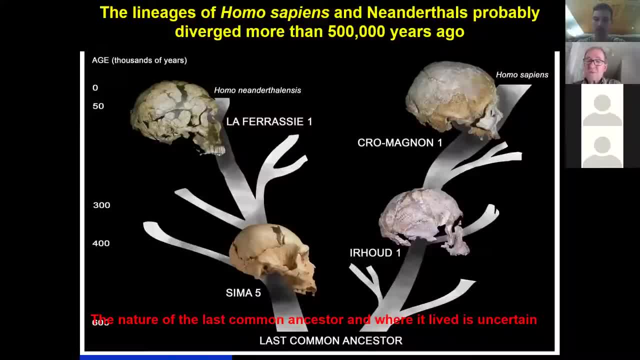 Geneticists estimate that we had a common ancestor with the Neanderthal lineage, probably more than 500,000 years ago. But who that ancestor was and where that ancestor lived, I think now is much less certain than I used to think. I used to think the common ancestor was a species called Homo heidelbergensis. 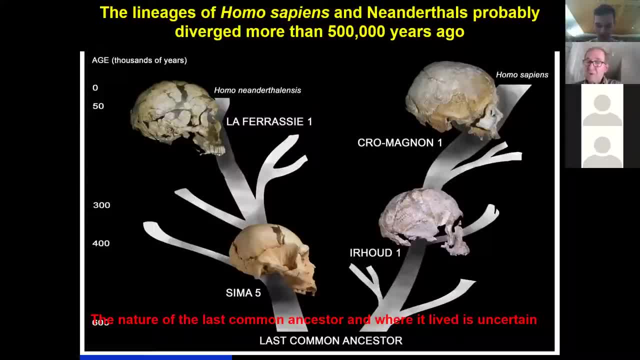 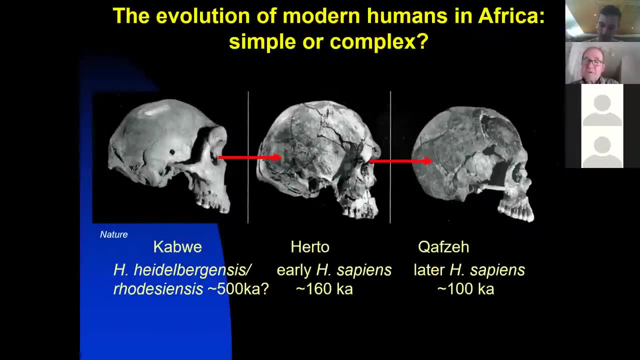 And now I'm not sure about that, And I'm not sure what continent that common ancestor lived on. It may have been in Europe, It may have been in Asia, It may have been in Africa, And because the African story seemed to be relatively simple until recently, 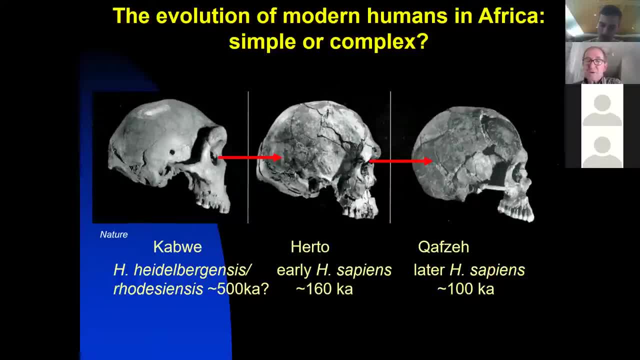 So here's a common representation of the evolution of Homo sapiens in Africa, with this earlier species, Homo heidelbergensis or Rhodesiensis sometimes called, Represented here. Represented here from the Broken Hill fossil, also known as Cabway. 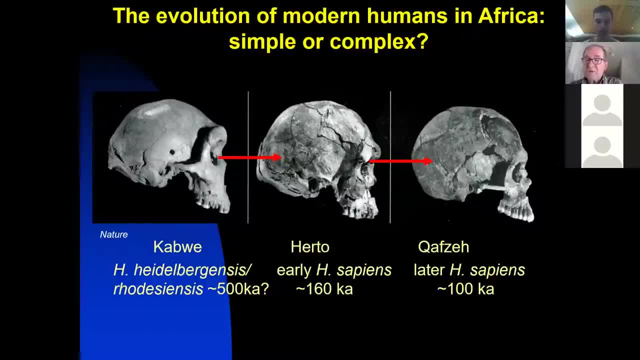 Estimated often at 500,000 years old, giving rise to early forms of Homo sapiens and giving rise then to later forms of Homo sapiens. So this was seen as a relatively gradual transition and possibly- in fact probably for some people- occurring in only one area of Africa. 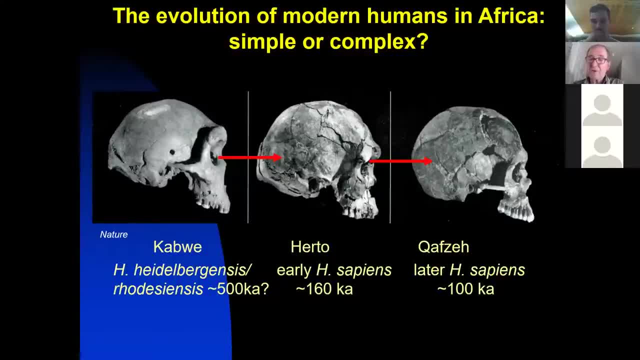 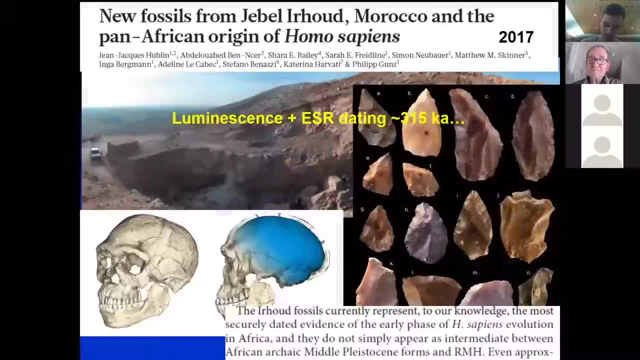 East Africa was often the favoured area for this transition from heidelbergensis Through to Homo sapiens, And we know that that representation of Homo sapiens, as we've suggested, goes back quite deep. So the Jebel Ehud fossils, which some of them were found back in the 1960s, 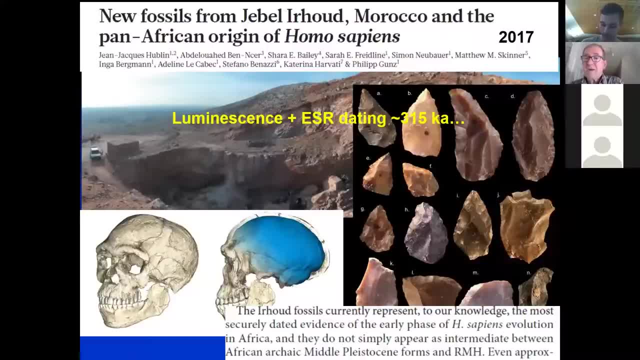 They've only recently been dated properly and more material has been recovered from the site. So we have these beautiful stone tools from the site, We have luminescence dates and ESR dates for the material of around 300,000 years, And we've got more complete reconstructions of the Jebel Ehud material. now 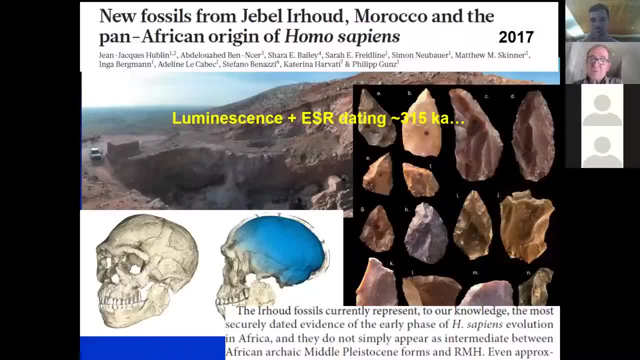 So a composite reconstruction there of the Jebel Ehud 1 fossil with a jawbone added to it from relatively new discoveries. And the Jebel Ehud fossil has got some modern human features: in the teeth, in the jaws, in the middle of the face, the shape, 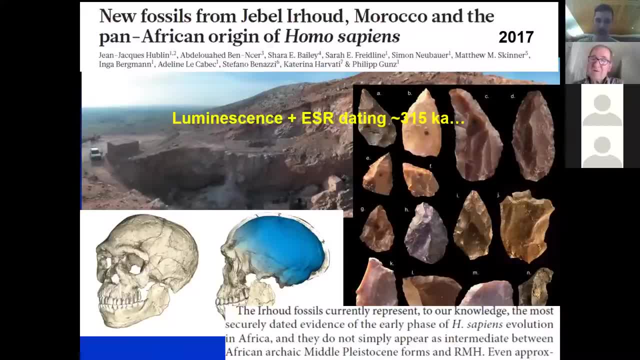 But the brain case is still quite primitive. It looks like Ehud- if it is a Homo sapiens- hasn't yet evolved That high rounded brain case that we find in later Homo sapiens, But that high and rounded brain case is there. 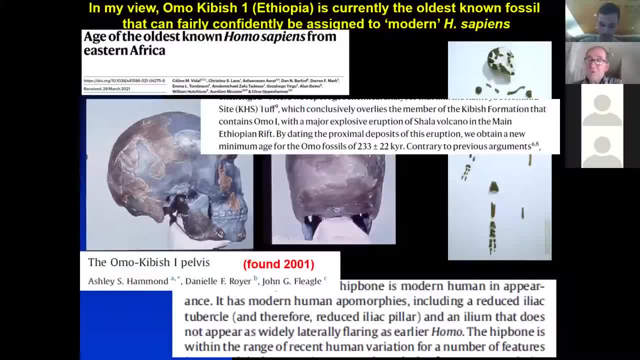 And we now know it was there in Ethiopia more than 200,000 years ago. So this fossil Onokibish 1, found by Richard Leakey's team back in 1967 in southern Ethiopia. The cranial vault is high and rounded. 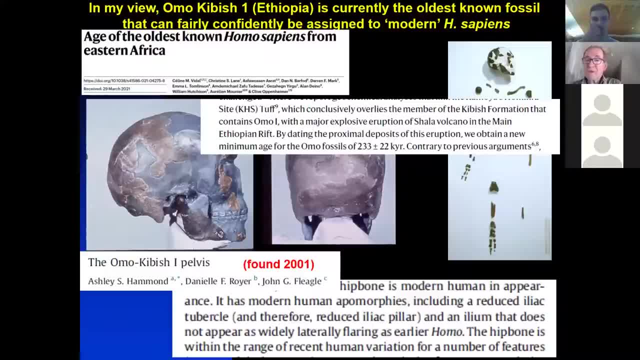 There's a small brow ridge, There's a chin on the lower jaw, It has upper parietal expansion And there's also a skeleton associated with it which does have modern human features, including in the pelvis. So this fossil, as it says, has recently been dated by a major explosive eruption of the Shala volcano in the main Ethiopian rift. 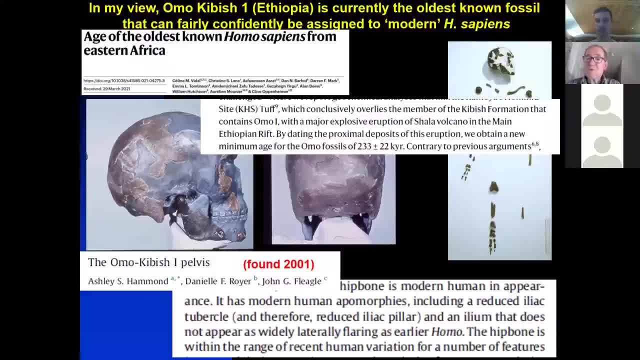 By dating the proximal deposits of this eruption, we obtain a new minimum age for the Homo fossils of about 233,000.. So this is a fossil Which for me, is a modern Homo sapiens, at least in the parts preserved, And yet it's over 200,000 years old. 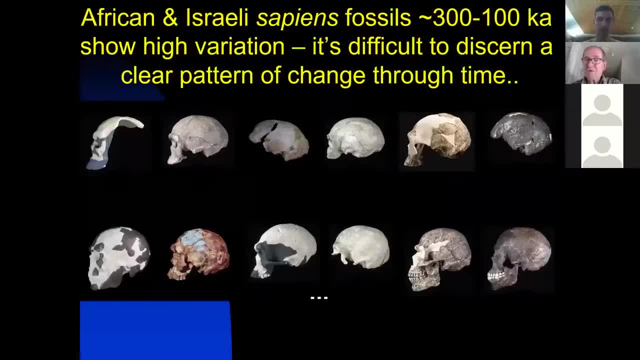 But when we look at the African fossil record as a whole for Homo sapiens it's really quite diverse And there isn't a clear pattern of change through time. If you line these fossils up, in the best we can, in a chronological sequence, they don't form an ordered, gradual sequence through from more primitive to more derived. 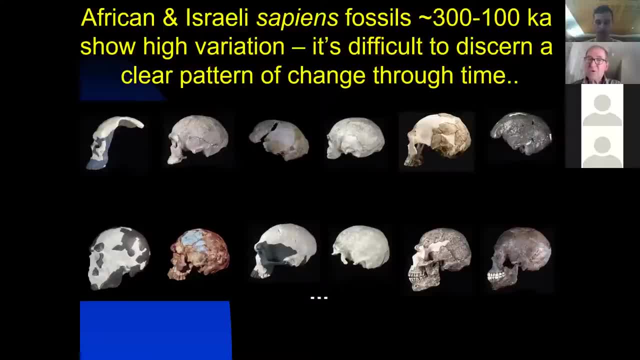 More modern looking. Some of the fossils show mixed features And even at one site, such as Homo kibish, we have two very different looking fossils which appear to be about the same age, So there's no clear pattern of change through time. 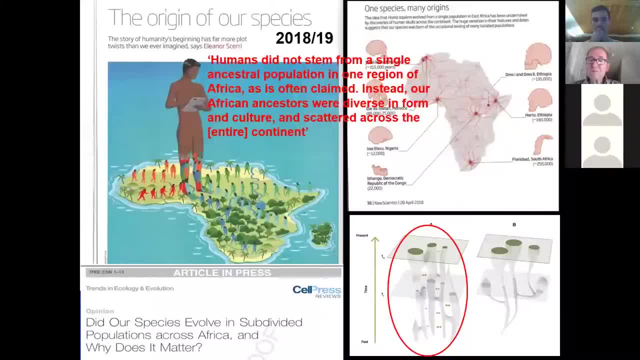 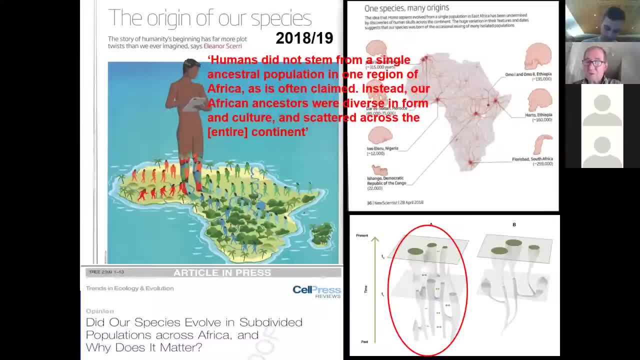 It wasn't Africa And this is a pan-African origin, And I've worked with other people such as Eleanor Sherry on this, and Eleanor's quote there says that humans did not stem from a single ancestral population in one region of Africa, as is often claimed. 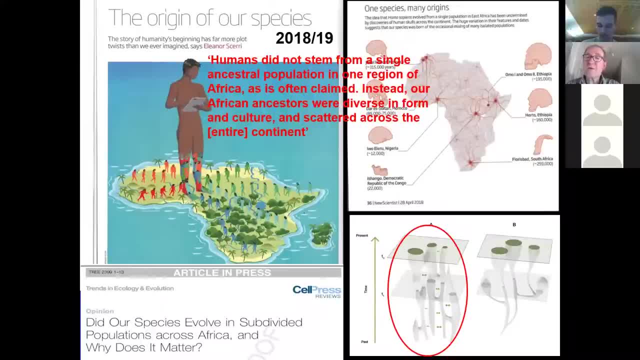 Instead, our African ancestors were diverse in form and culture and scattered across the continent- I wouldn't necessarily say the entire continent contributed to the evolution of what we call Homo sapiens and what we call modern Homo sapiens. So the evolutionary pattern is as shown there on the bottom right. there We've got lineages in. 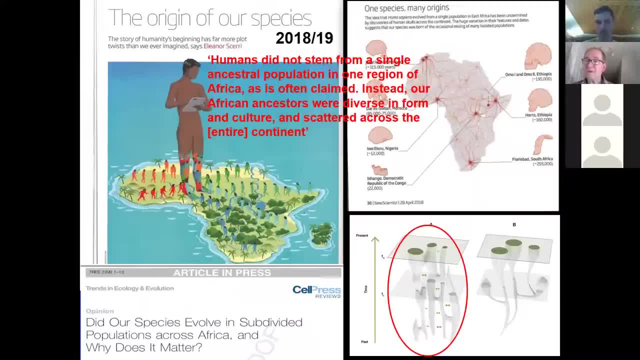 different parts of Africa, at times going their own separate ways, at other times, when climate allowed it, mixing with other populations, and so we get a kind of mosaic evolution of Homo sapiens and a coalescence of the modern Homo sapiens pattern in the last 100,000 years. So no single. 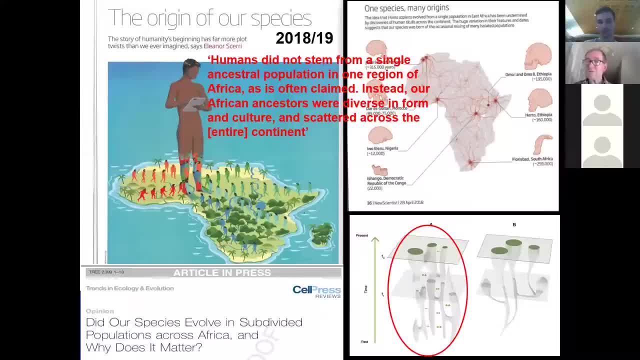 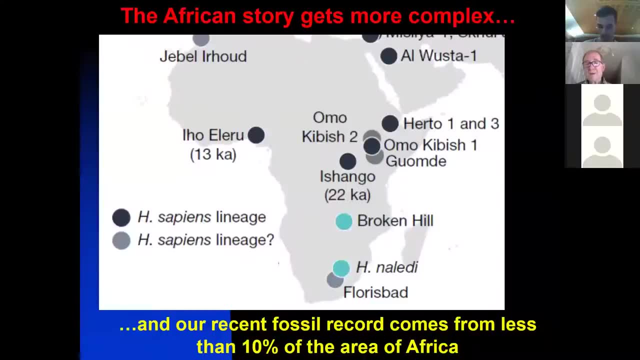 centre of origin and not certainly a gradual change in one place, a much more complex pattern than we used to think. And it's even more complicated than that because this map here shows some of the early Homo sapiens fossils in black and grey, but there are archaic humans around at. 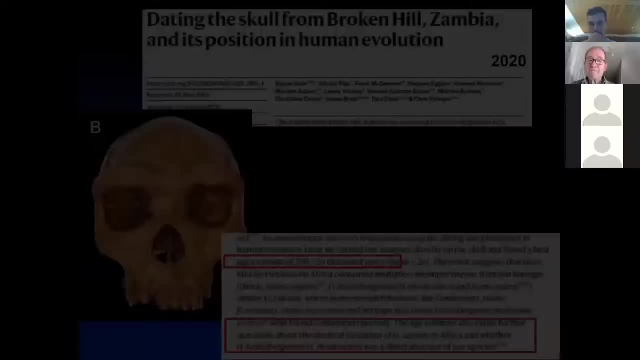 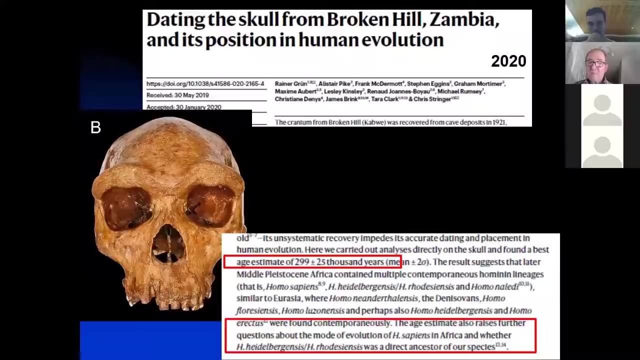 the same time As we now know. So this fossil from Broken Hill Cabway- this is a paper from 2020, where we dated this fossil directly And, as it says here, the best age estimate is about 299,000 years. The age: 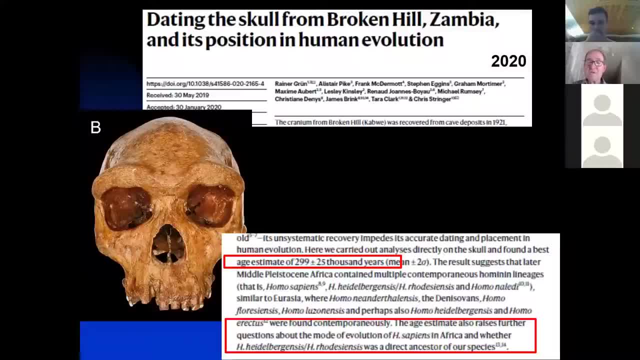 estimate raises further questions about the mode of evolution of Homo sapiens in Africa and whether Homo heidelbergensis or Odysseensis was a direct ancestor of our species. So that's both chronological, because of course you know, we've now seen that the Homo kibish 1 fossil, which looks 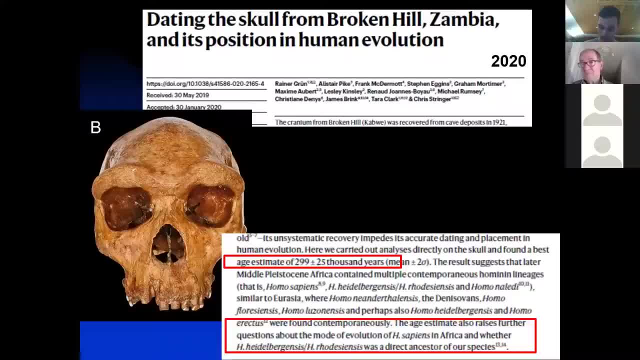 much more modern, is only about 70,000 years, maybe younger than this fossil, And we also look at the morphology of these fossils. So the Broken Hill fossil for me has a face which is very unlike that of Homo sapiens, much less like Homo sapiens than say. 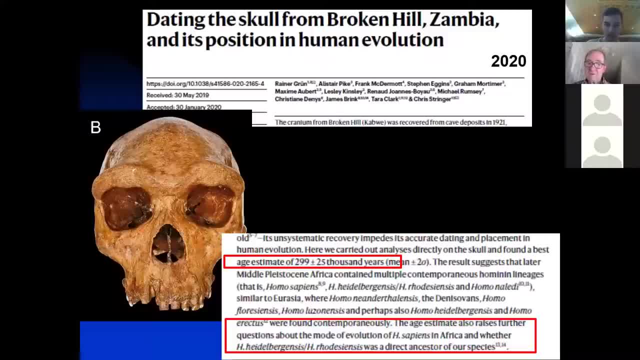 the Ghibli Hood face. So I think that this group that I've called heidelbergensis or Odysseensis, I think it shows derived features away from the modern human pattern in the face And for me that makes it much less likely that this group is the common ancestor for us and the Neanderthals. 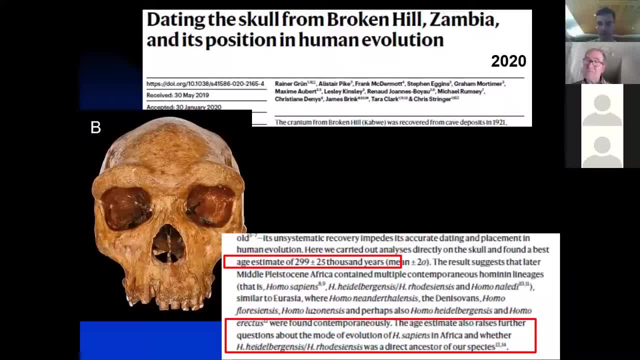 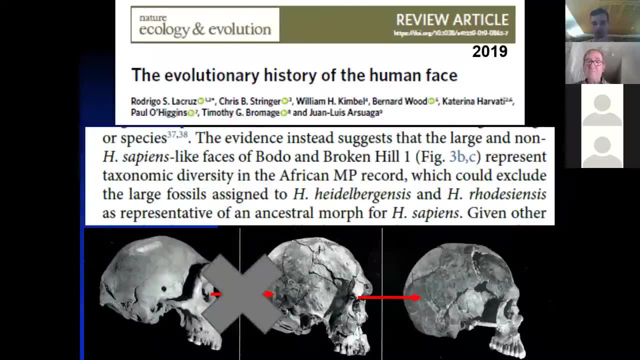 And that's also unlikely when several examples certainly are actually contemporary, with Homo sapiens rather than earlier. So this model seems not to be accurate now, As it says here, the evidence suggests that the large and non-sapiens, like faces of Bodo and Broken Hill 1,. 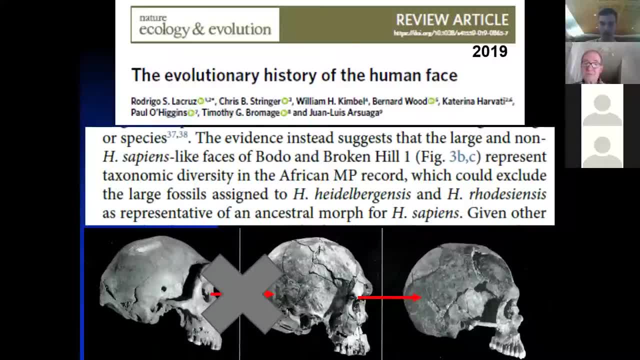 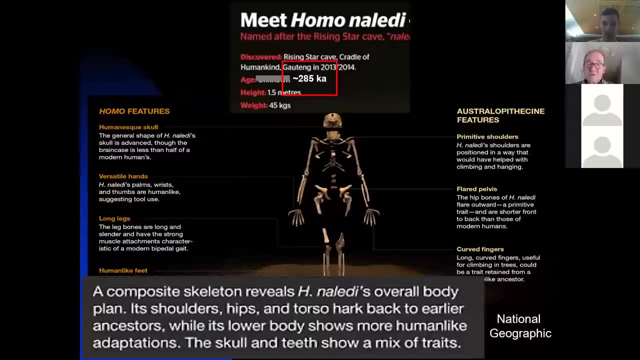 represent taxonomic diversity in the African middle Pleistocene record, which could exclude the large fossils as representative of an ancestral morph for Homo sapiens. And it's even more complicated than that because down in southern Africa we have a much more primitive species surviving until around 300,000 years ago. This is Homo naledi only found. 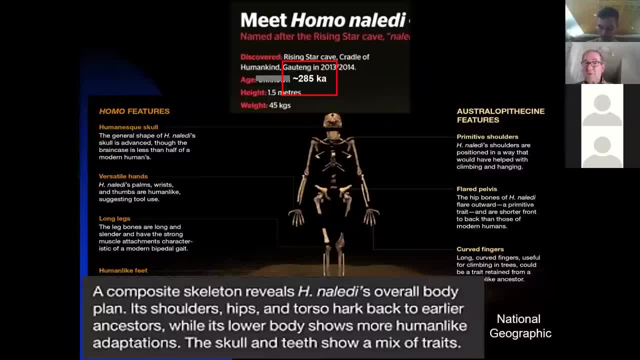 in the last 10 years or so, And as it says here, a composite skeleton reveals Homo naledi's overall body plan. Its shoulders, hips and torso hark back to earlier ancestors, while its lower body shows more human-like adaptations. The skull and teeth show a mix of traits, and that includes a. 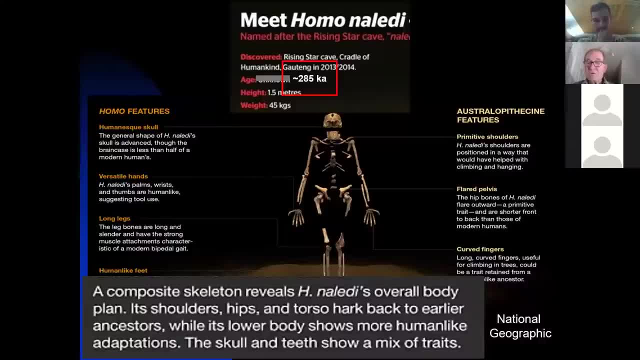 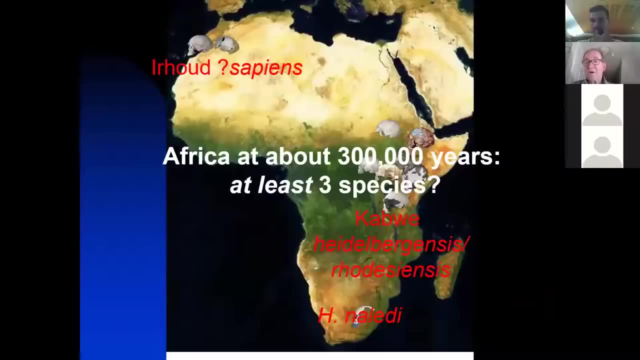 brain capacity which is really only comparable with some of the great apes of today: chimpanzees and gorillas. So this small-brained species still surviving around 300,000 years ago. So yes, the sapiens lineage seems to be evolving in northern and. 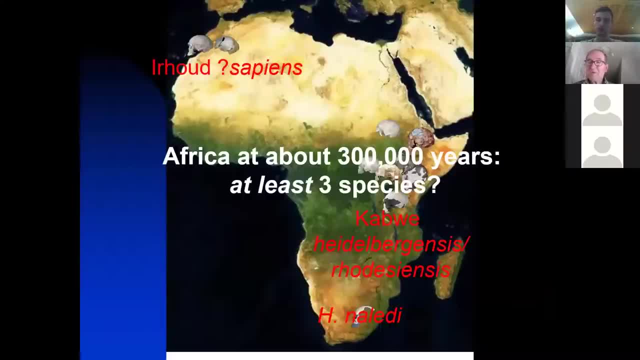 northeastern Africa We've got Heinebergensis or Rhodesiensis still around about 300,000 years ago in Zambia and down in southern Africa something much more primitive still, Homo naledi. And of course we have no idea when the Heinebergensis, Rhodesiensis and Naledi lineage has actually 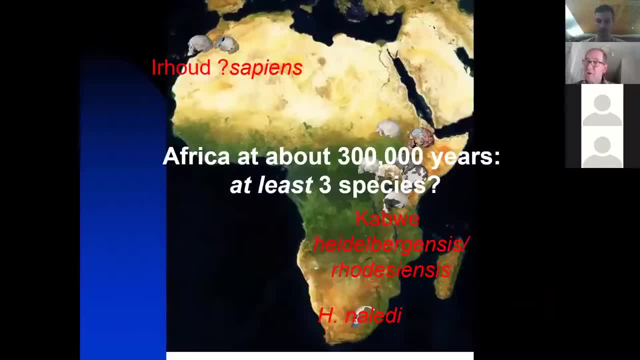 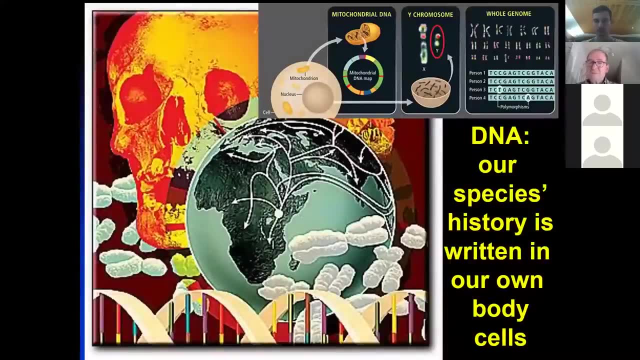 disappeared. We can date them around 300,000.. They may well have survived later than that And, of course, DNA contributes to the story And one of the regrettable things is that, because of the climate of Africa, we have only very poor DNA preservation. 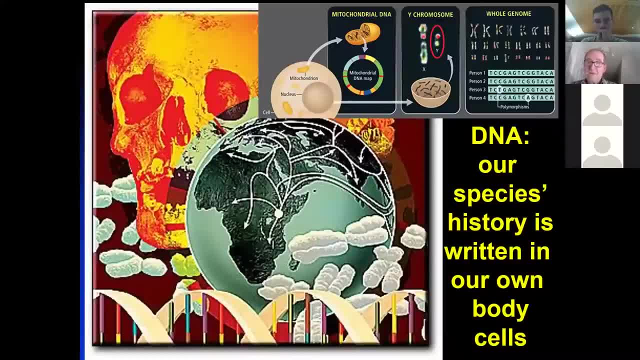 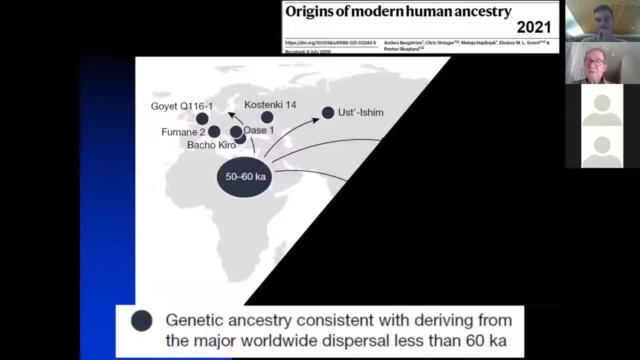 And the known DNA from African fossils only at the moment goes back to about 15,000 years. So whether we'll ever have fossils from those earlier forms, those earlier species, is looking. it looks unlikely at the moment. But what the data do show is that modern humans outside of Africa today genetically seem to trace. 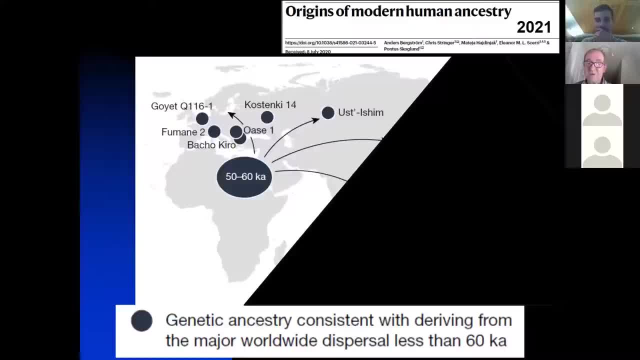 back to a dispersal that happened about 60,000 years ago. So this is from a paper I was on from earlier last year And, as we say here, this diagram shows in black here a number of fossils that have complete or partial or complete genomes, which suggests that genetic ancestry is consistent with. 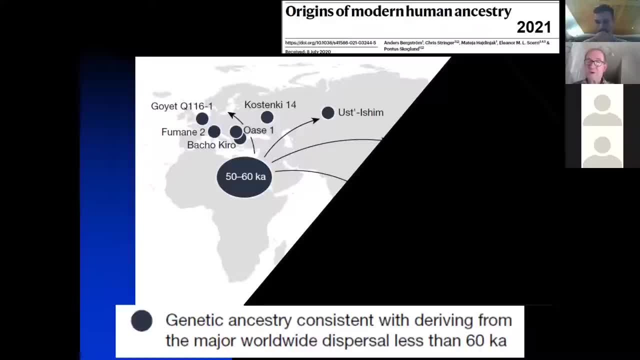 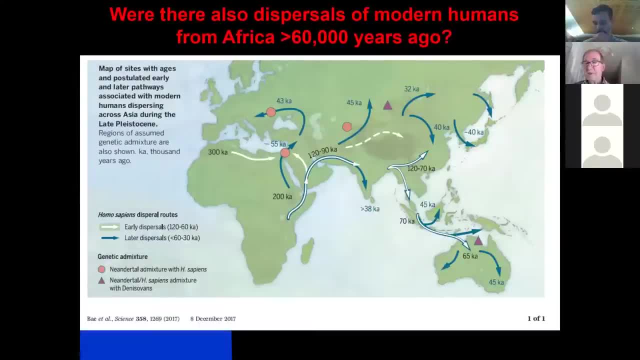 deriving from a major worldwide dispersal less than 60,000 years ago. So that dispersal, of course, was going to bring these humans into the territories of the Neanderthals And it's a bit more complicated than that. So this dispersal at 60,000, it looks like it wasn't. 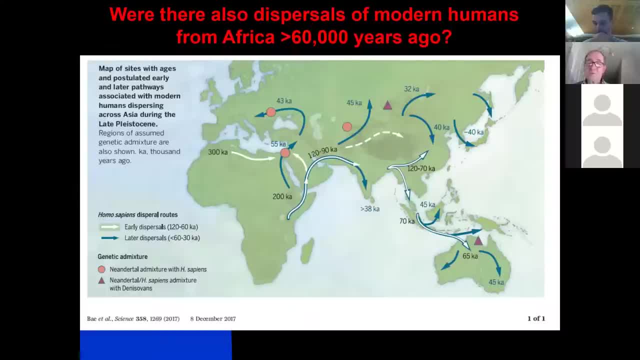 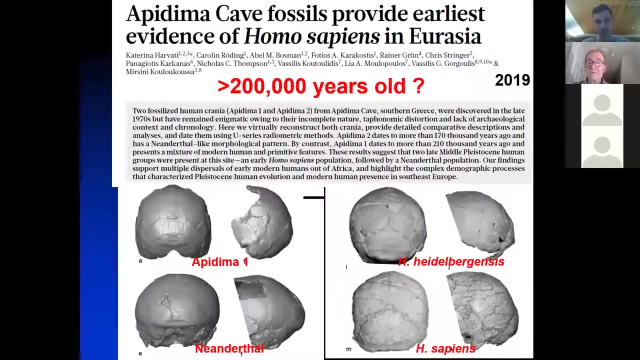 the only one that Homo sapiens, the only excursion that Homo sapiens made out of Africa. This diagram, this map, shows some possible earlier ones, including to China and Australia, And we've got this incomplete fossil from Greece, from Epidema Cave. 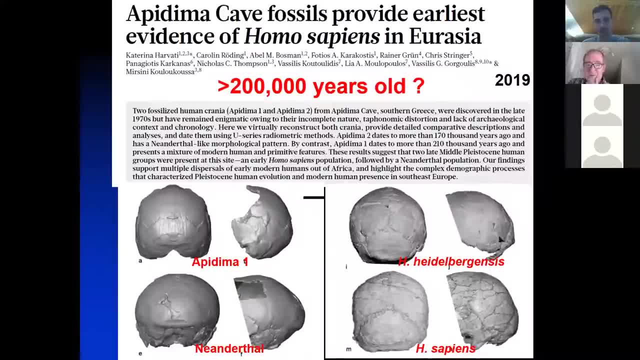 in the Peloponnese And Epidema 1,. as shown there at the bottom, it's only the back of a skull, But it looks like a Homo sapiens fossil. The back of the skull is high and rounded And it looks. 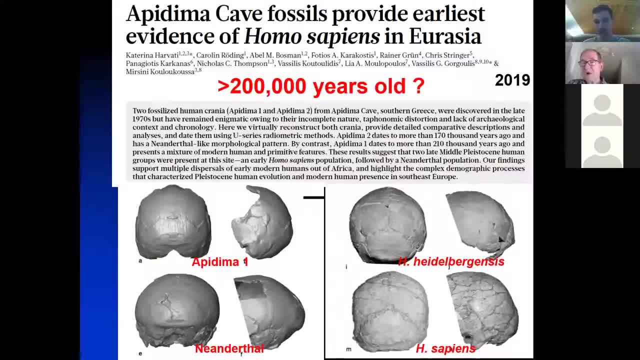 most like a fossil, like Shkul 5, which is on the bottom right there. That fossil of Shkul 5 is similar in the preserved parts, to Epidema 1.. So this morphology of Epidema 1 is very different from the Neanderthals, very different from Heidelbergensis, And yet this fossil is dated. 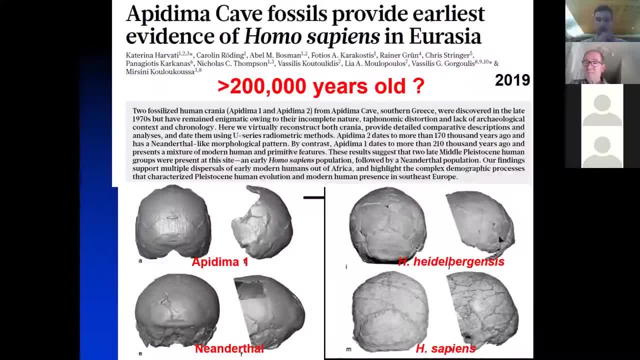 by uranium series to over 200,000 years old. And what's interesting is that Epidema Cave- it looks like the Neanderthals occupied the cave after this date. So we've got a situation where we seem to have maybe a brief dispersal of Homo sapiens into Europe And then that population disappears. 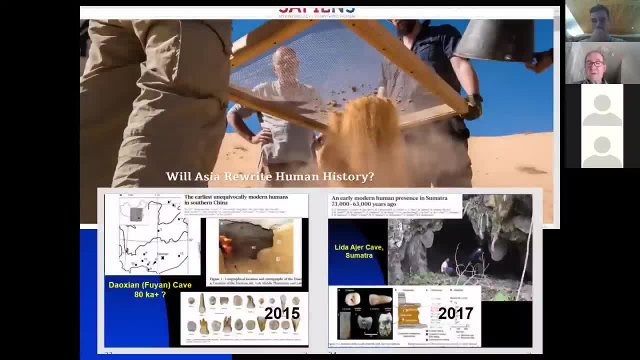 and is replaced by Neanderthals, And there's further complications from the Far East. So we've got sites in China which seem to show Homo sapiens fossils at more than 80,000 years old. We've got a couple of teeth from Sumatra. 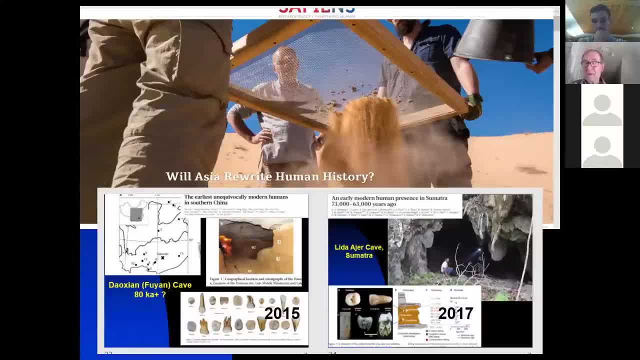 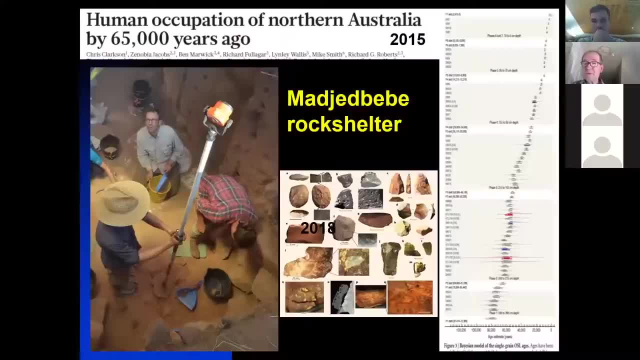 which seem to be more than 65,000 years old And equally challenging the archaeological data from Northern Australia. So, Majabebe 2,, this rock shelter has a long sequence with a series of luminescent states And at about 65,000 years ago. there's a very rich layer, rich in complex. 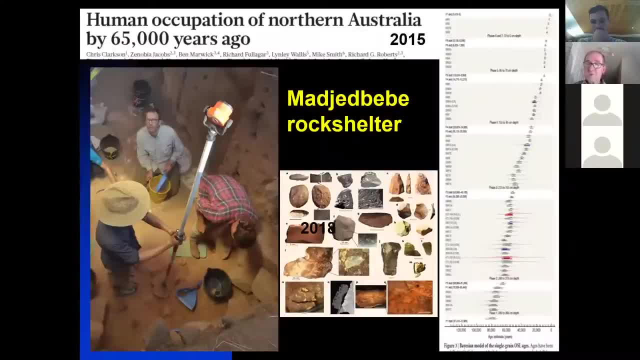 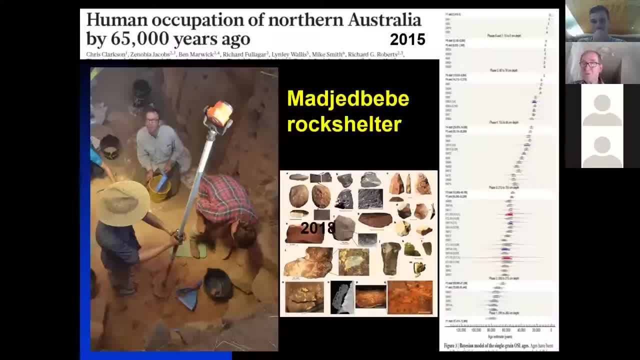 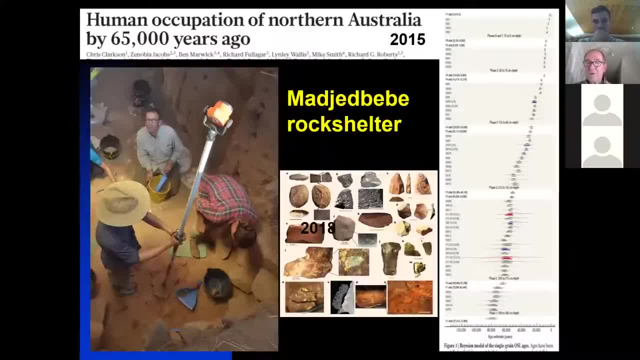 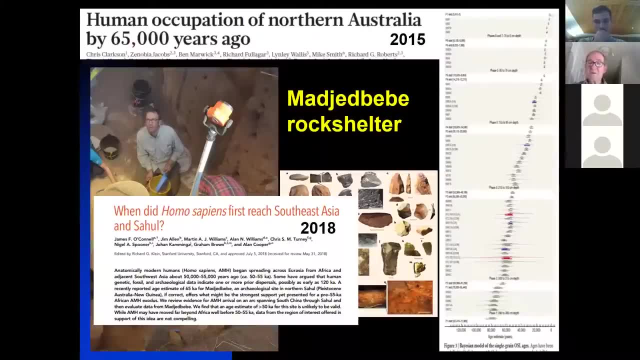 diversity outside of Africa. Now, of course, not everyone accepts the dating there. So here's a paper that critiques that dating and argues that the material in Majabebe is more likely about 45,000 years old. So I think this is an open question. Obviously, more dating will help resolve this. 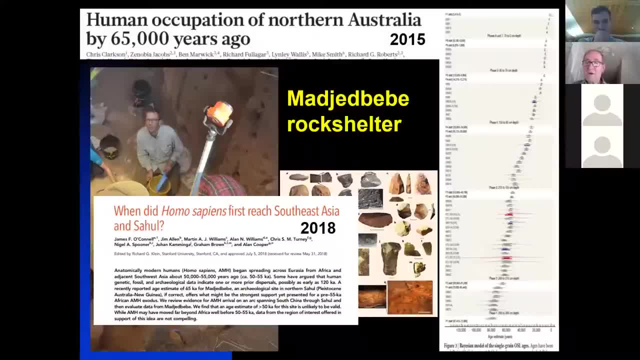 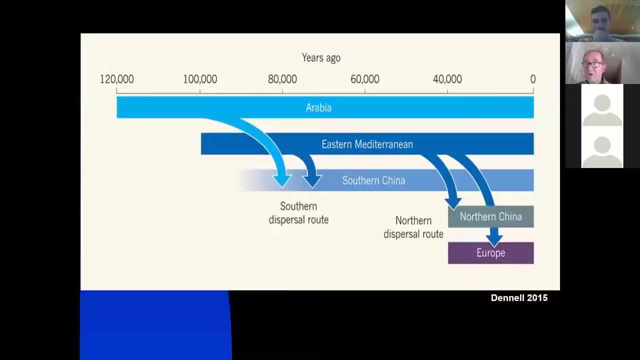 more sites will help to resolve this, whether we can't just be the only site in Northern Australia of this age, that there will be others to be to be found and dated, if that story is correct. But because it does lead to issues in explaining the data, in matching the archaeological data, the anthropological data and the genetic data. 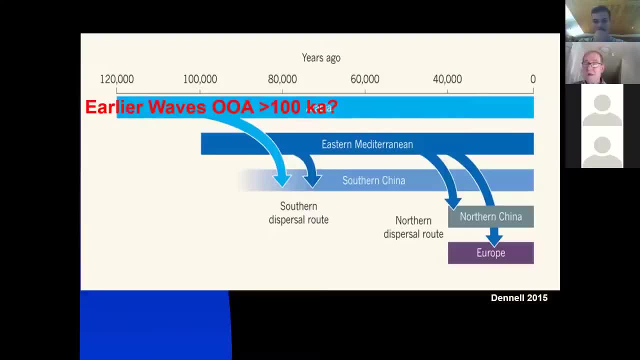 So, yes, it looks like there could well have been earlier waves out of Africa more than 100,000 years ago, including epidemia, including that material, in Southeast Asia and Australia. And then we have the main wave which geneticists map from present day diversity outside of Africa. 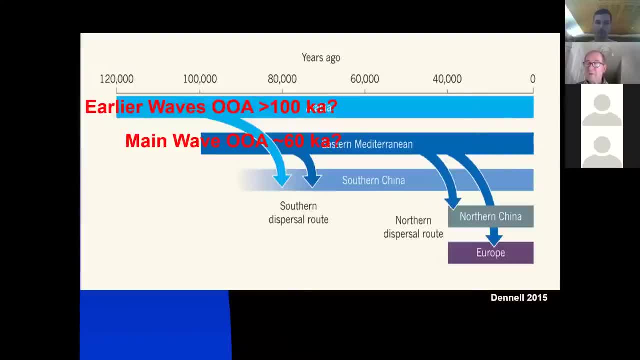 which occurred around 60,000 years ago, And we have to argue that that main wave overprinted any surviving trace of those earlier dispersals of Homo sapiens out of Africa. So whether those early dispersals were unsuccessful and disappeared completely, or this wave at 60,000 was so strong, 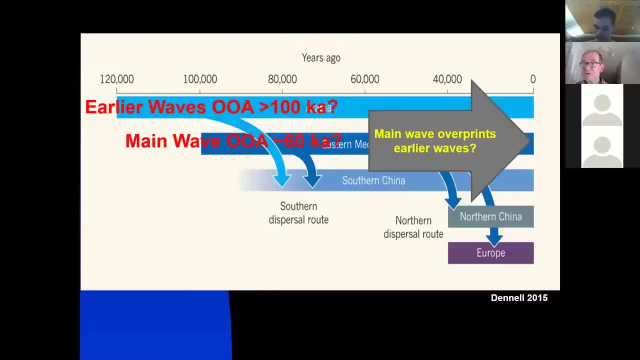 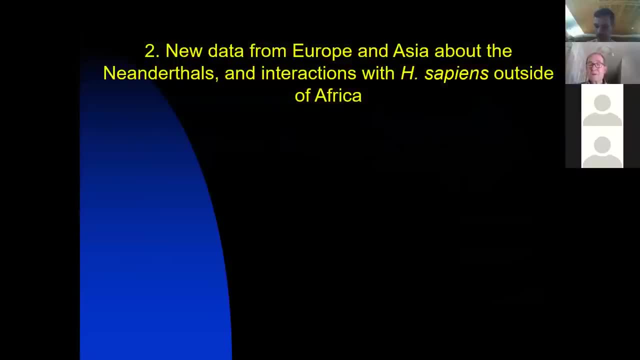 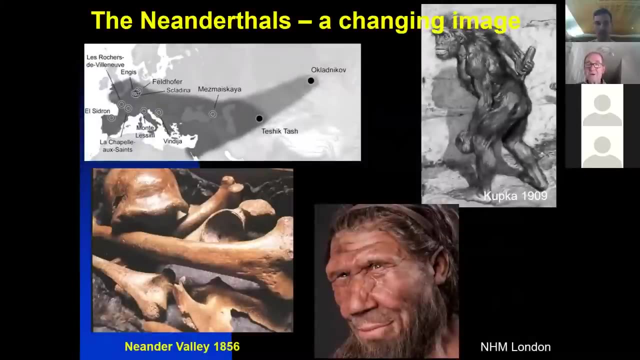 it swamped them, if you like, genetically, and removed any trace of those earlier waves in the in terms of the genes of people outside of Africa today. So now let's look at the situation in Europe and Asia and the interactions with the last Neanderthals. 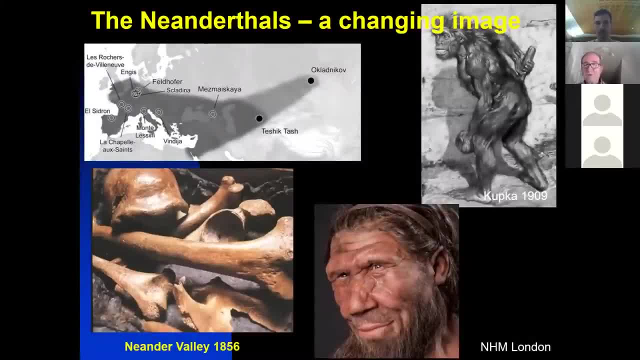 And of course it's worth. I don't need to tell you people, I'm sure that the Neanderthal image has greatly changed in the last, particularly the last 20 years, I think So. the original Neanderthal finds, of course, dating back to 1856 in the Neander Valley. We now know the Neanderthals covered a wide 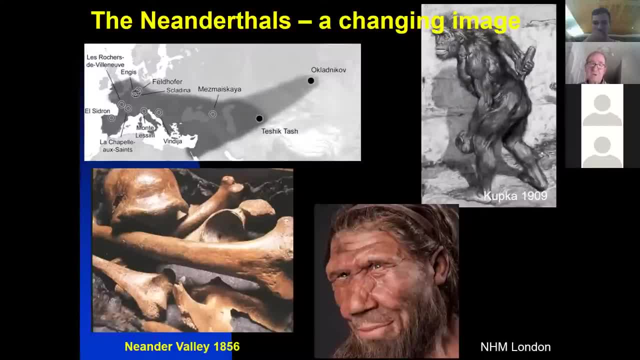 range of cultures and they were not just geographically, they weren't just European. they were in Western Asia, they were in Uzbekistan and they were over in Siberia at times. I think they were probably in China at times And their image as it shows on the right hand side. 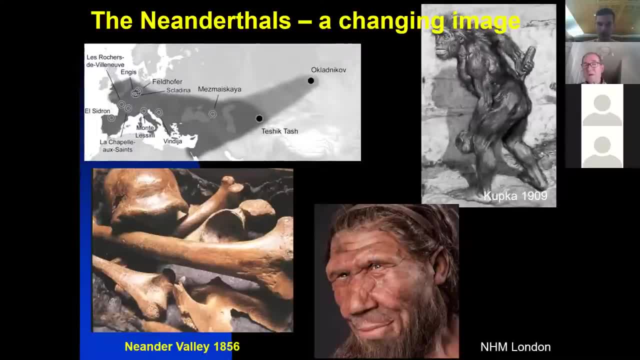 on the top right. there we've got an image of the Neanderthals from the early 1900s, where at that time there were no really primitive African morphologies. We didn't have fossils of australopithecines, for example, back in the early 1900s. 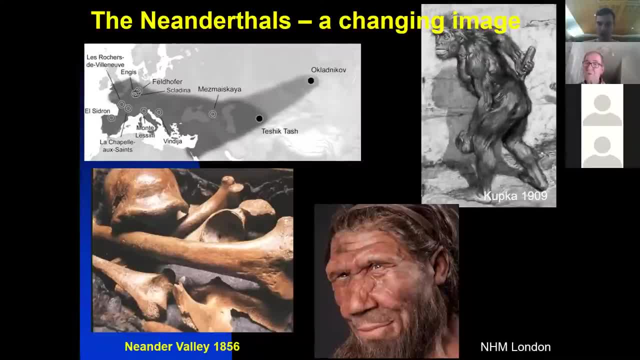 So the Neanderthals believed in human evolution kind of pushed the Neanderthals into this position of a sort of missing link. That Neanderthal there depicted as very bestial, bent knees, hairy, grasping big toes, head hung forward and so on, And then at the bottom right there we've got a. 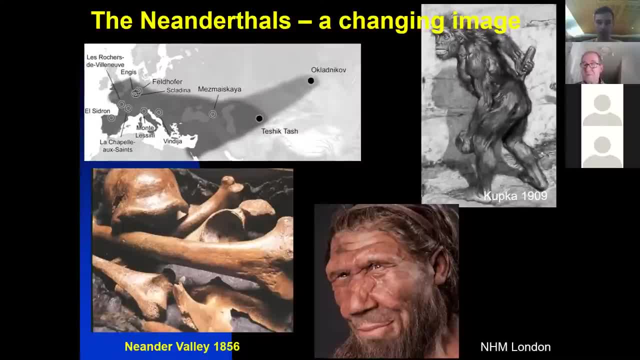 contrasting image from our exhibition in London by the Kennes brothers showing this much more human representation of the Neanderthals. In fact, the Kennes brothers told me that they had based this reconstruction, the expression of it, on a photograph they'd seen of Sean Connery. 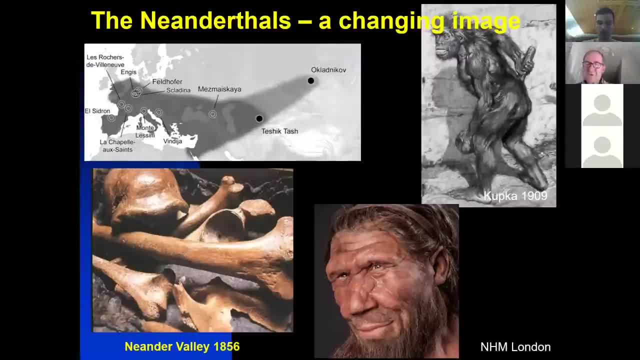 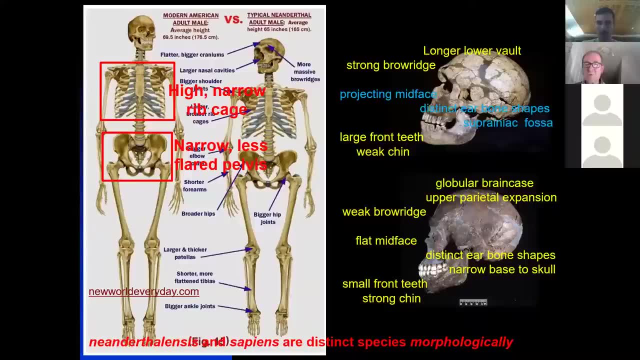 So here we are: a very human representation of the Neanderthals, But they were distinct from us. I think they were fully human, but a different kind of human. So we've got a Neanderthal skeleton now, compared with the modern human one. So Neanderthals have 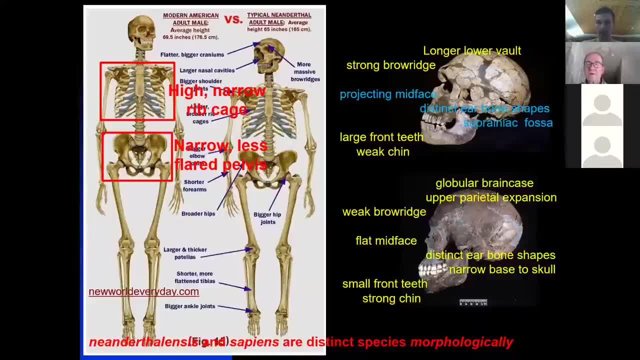 got a much bigger rib cage, more voluminous, wider, deeper. Probably the lung capacity was 20% bigger than that in Homo sapiens, A much wider and more flared pelvis. Probably the internal organs of the Neanderthals were somewhat larger than our own. 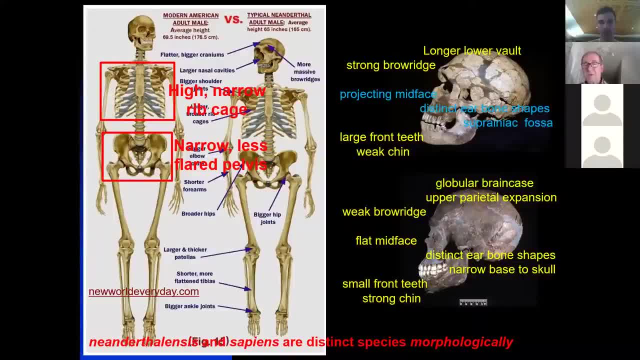 The joint surface is much larger. on the bones The muscle markings are much deeper, And the differences are there when we come to the skull as well. So at the top there we've got a Neanderthal from our Pharisee, Some primitive features there. So the brain case is long and low. 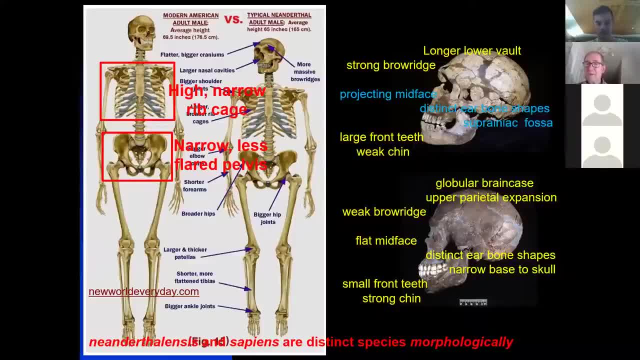 as it is in earlier humans, with a strong brow ridge at the front, Not much sign of a chin on the lower jaw, Large front teeth And then some really distinctive features in the Neanderthal skull, such as that projecting mid face, an enormous nose on the middle of the face, and the face is 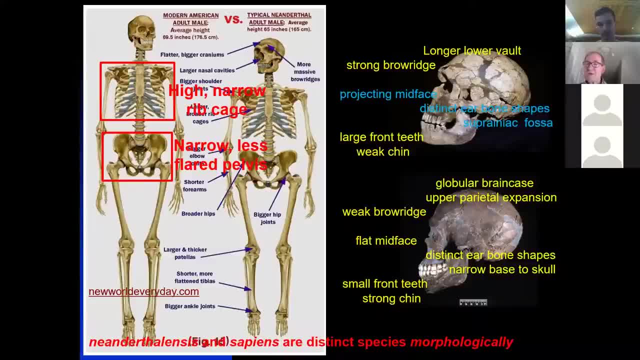 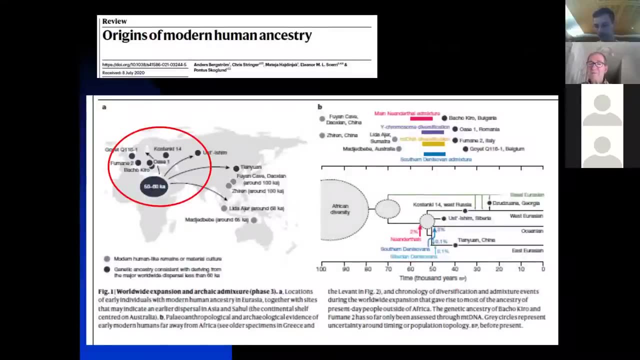 pulled forwards, Distinct ear bone shapes and a little depression at the back of the skull called the supineac fossa. So Neanderthals can be recognised very well from their fossil record And, as we've said, modern humans, having evolved in Africa, start to emerge from there particularly. 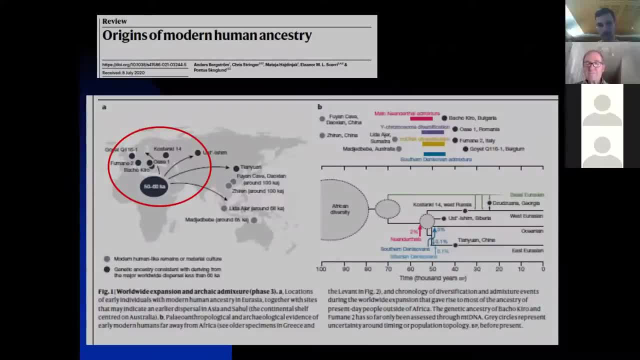 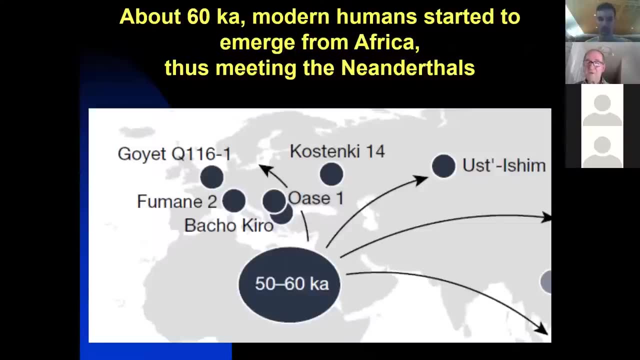 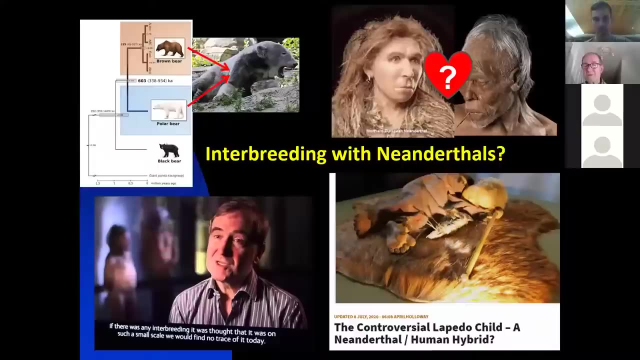 in the last 60,000 years, And so these are some of the genomes that we can map that dispersal of Homo sapiens into the territories of the Neanderthals, And so that brings up that always tricky and controversial question of interbreeding with the Neanderthals. It's something we've argued. 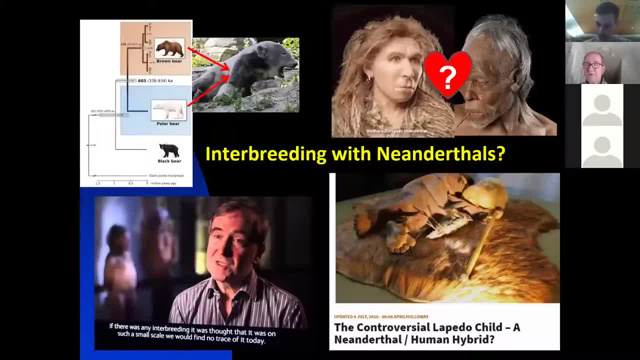 about for many years. So on the bottom right there we've got a fossil from Portugal, the Lepido child from La Gavella, And that's been argued to be a hybrid of a modern human and a Neanderthal. We now know that fossil is only about 26,000 years old. Unfortunately, there's no DNA from it. 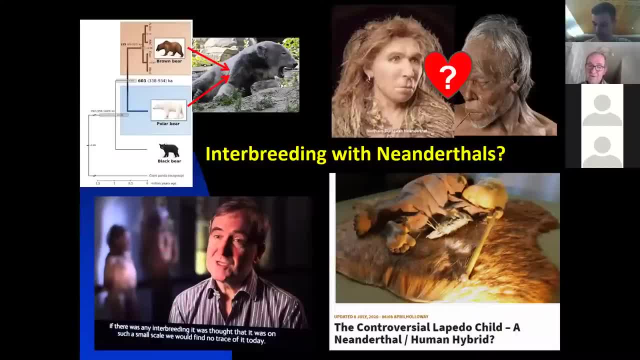 but it seems very unlikely that it's any kind of hybrid. It seems to be just a Homo sapiens child from the Gravetian, And at the top left there we can see evidence from modern species of mammals that they can hybridise successfully. So there's an example of the brown bear and polar. 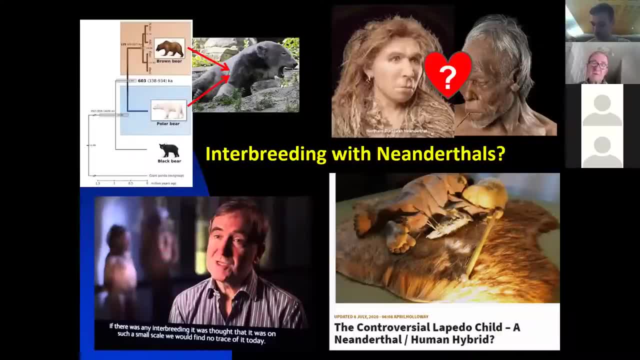 bear hybridising successfully in zoos, And the offspring are fertile. they're interfertile And the divergence time of the polar bear and brown bear is about comparable with the divergence time of us and Neanderthals. So I was certainly aware that closely related mammal species could. 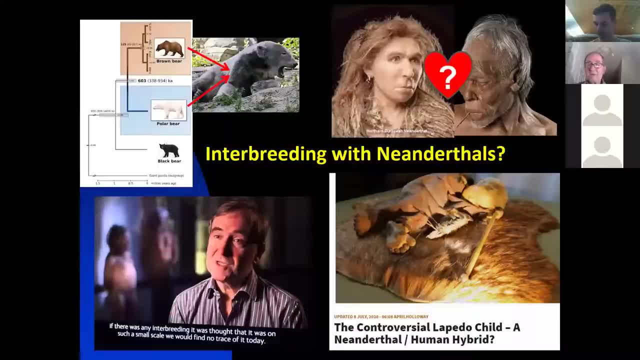 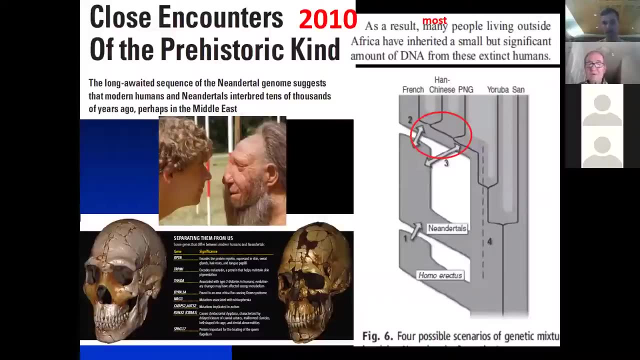 often hybridise. We know jackals and wolves can, many species of baboon can, But my view until recently was: well, that happened a long time ago. it was probably rare and we're not going to find any evidence of it today. But I'm a bit wrong and that was shown clearly. 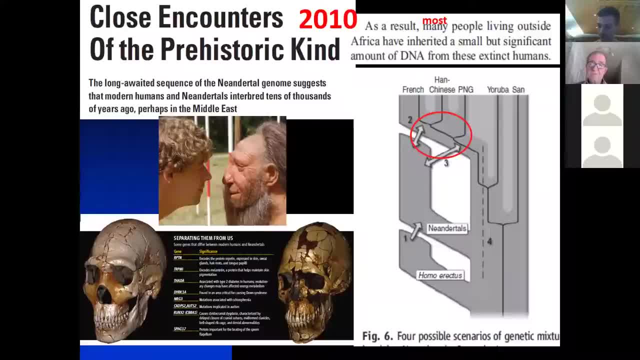 from 2010 onwards, when the first really good quality Neanderthal genomes were reconstructed And, as it says here, close encounters of prehistoric kind. The long awaited sequence of the Neanderthal genome suggests that modern humans and Neanderthals interbred. 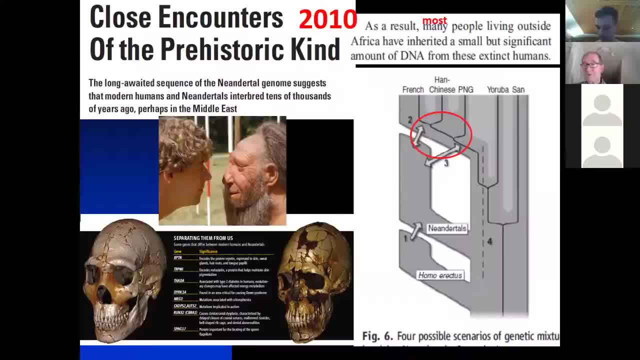 tens of thousands of years ago, perhaps in the Middle East, in fact, we now say, in a number of different regions of Europe and Asia. As a result, pretty well everyone living outside of Africa has inherited a small but significant amount of DNA from these experiments. 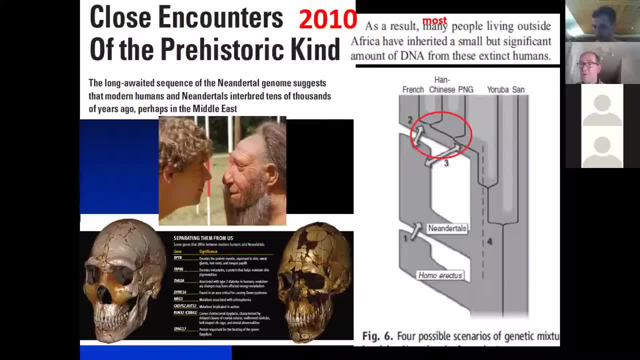 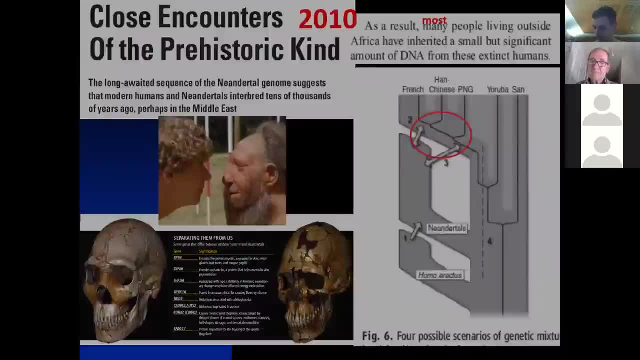 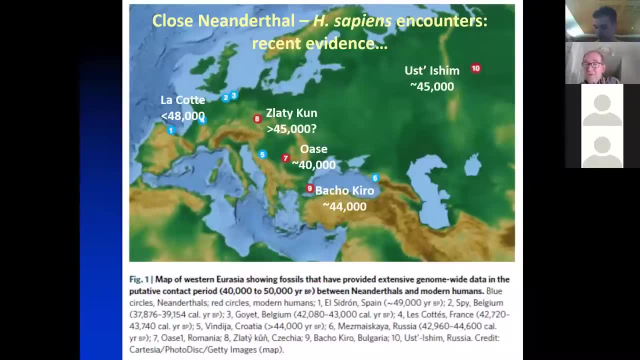 And we can map the interactions of the last Neanderthals and these Homo sapiens dispersing from Africa. Here are some of the sites which show the evidence. A number of these have been published recently And here's just one example from Oasi in Romania. 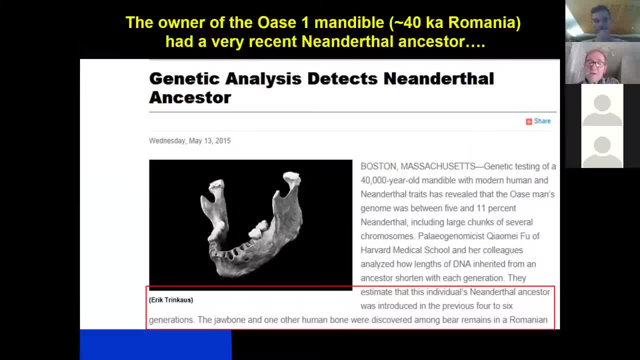 So this jawbone found many years ago now has a strong chin on the front and therefore looks like a Homo sapiens, but the teeth are large and have some unusual features, And so it was hypothesized that it might be some kind of hybrid. And sure enough, when the genome 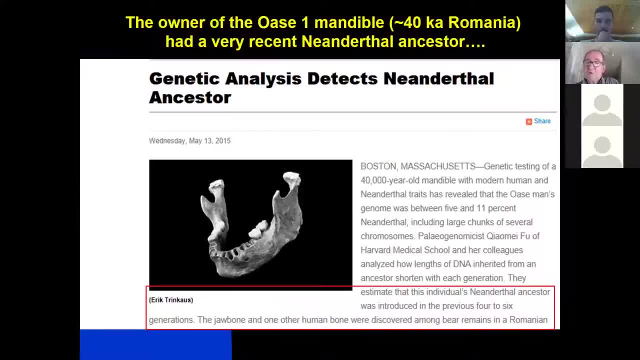 was analyzed. from this fossil, which is about 40,000 years old on a direct radiocarbon date, it was found to have about 9% Neanderthal DNA in the genome, so much more than we find today And as it says here, 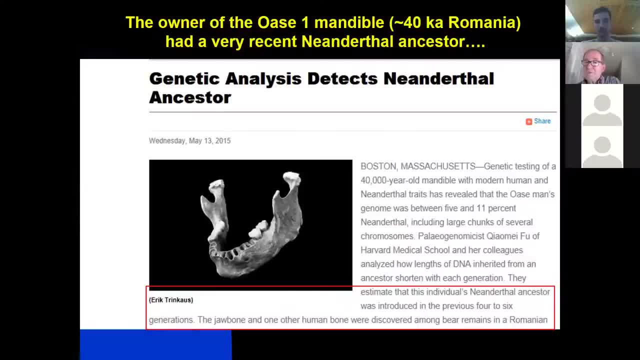 it's estimated that this individual's Neanderthal ancestor was introduced in the previous four to six generations, So this is data from a time when, as far as we know, the Neanderthals were heading for extinction- physical extinction- at least around 40,000 years ago, And yet there was still. 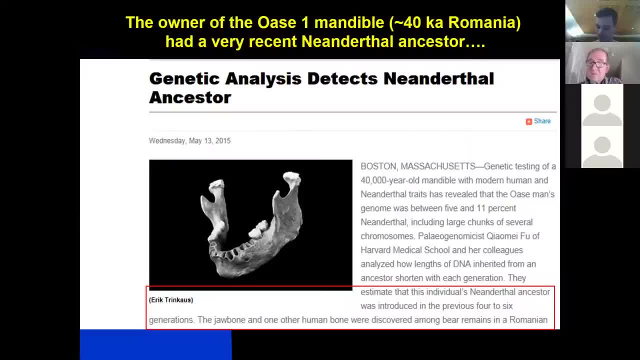 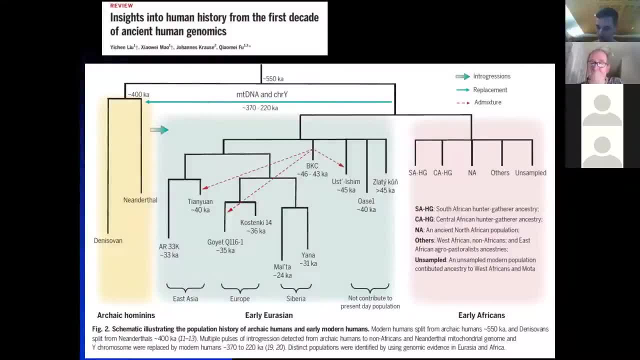 interbreeding going on between Homo sapiens and some of these late Neanderthals, And here's a paper that's worth a look if you want to really get an update on the genetic data, And this is rather a very interesting paper, And it's a very interesting paper And it's a very interesting. 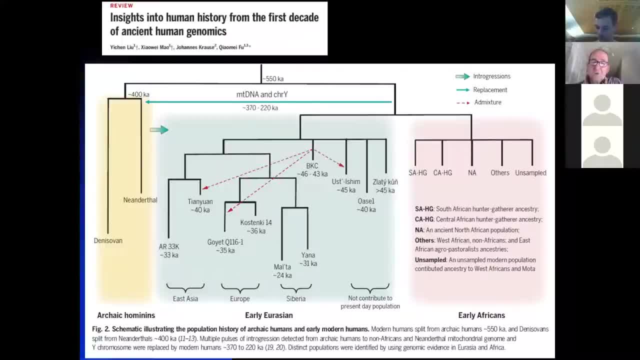 diagram And it's a very interesting diagram. And it's a very interesting diagram And it's a very complex diagram of some of the genetic data. So on the left hand side, there in yellow, we've got the Neanderthal and Dnispan lineages diverging off quite early, maybe 550,000 years. 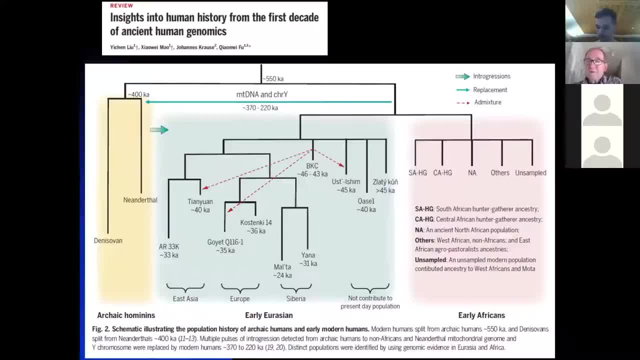 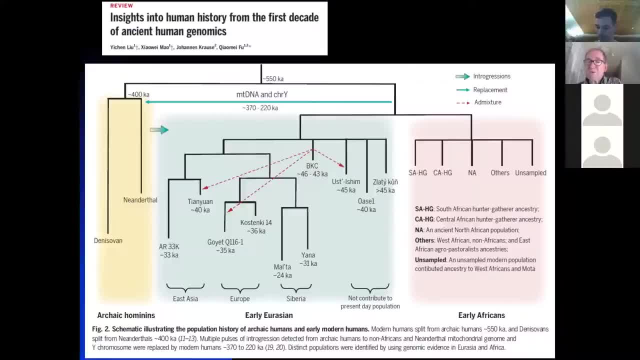 Some of these early lineages don't seem to have any modern descendants in the African, in the European genomes, So some of these lineages seem to have actually died out, But others, as shown here, contributed DNA which we find today in Europe and East Asia and Siberia. 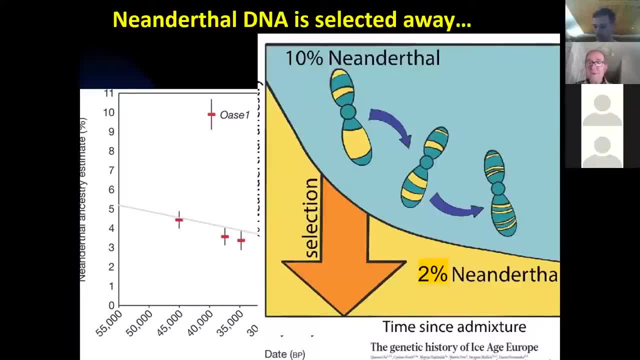 And that Neanderthal DNA and estimated that it could have been as high as 10% in some of these early populations that were mixing with the Neanderthals. but it soon selected away. So there's Awase on the left-hand side there close to 10% Neanderthal DNA But other early modern genomes. 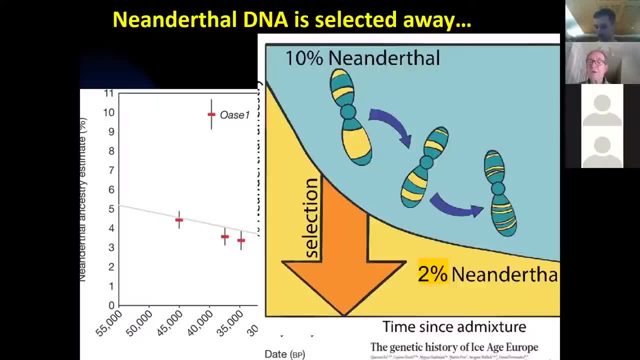 are shown there at the bottom And these show a declining amount of Neanderthal DNA through time. So selection is removing that Neanderthal DNA pretty quickly And it soon gets down to the level of around 2% that we find outside of Africa today. 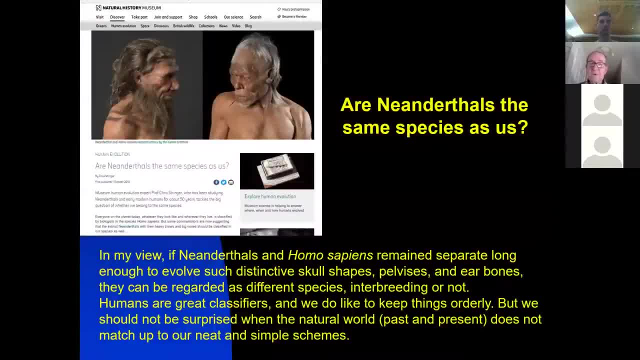 So this talk of interbreeding and Neanderthals brings up this always tricky question of species. And are the Neanderthals the same species as us? And I've written a piece which you can find on the Natural History Museum website. 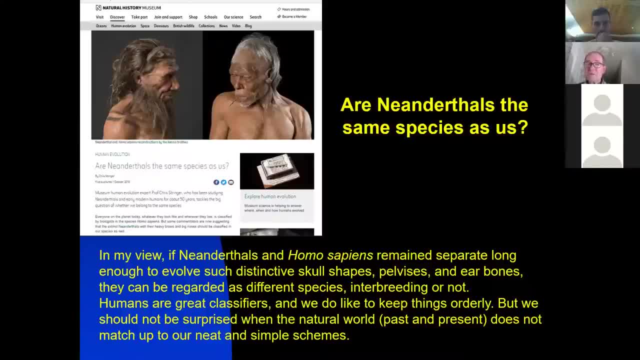 So, as I say here, in my view Neanderthals and Homo sapiens remain separate long enough to evolve such distinctive skull shapes, pelvises and ear bones. they can be regarded as different species, interbreeding or not. Humans are great classifiers and do like to keep things orderly, but we should not be surprised when. 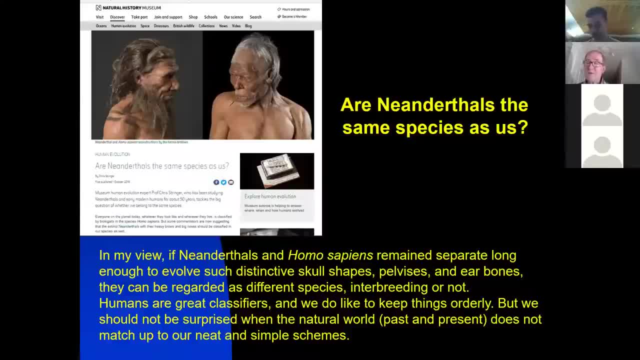 the natural world. past and present does not match up to our neat and simple schemes. So there's the biological species concept, which says that species are defined as being reproductively isolated. But that's only one of about 35 different species concepts that someone 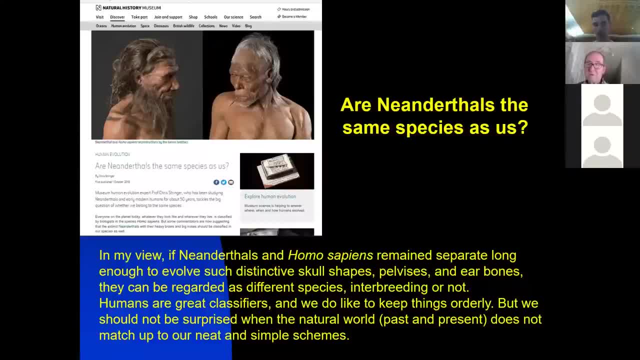 mapped recently And we know that the biological species concept doesn't work for species of bears, species of cats, species of dog, many species of birds. It's estimated that 20% of closely related bird species do a bit of hybridization. So I think us and the Neanderthals- it's not an exception. 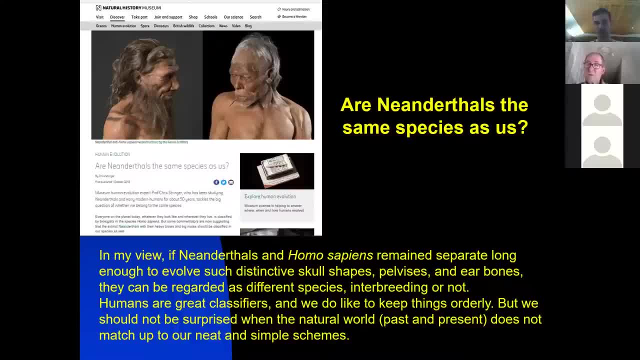 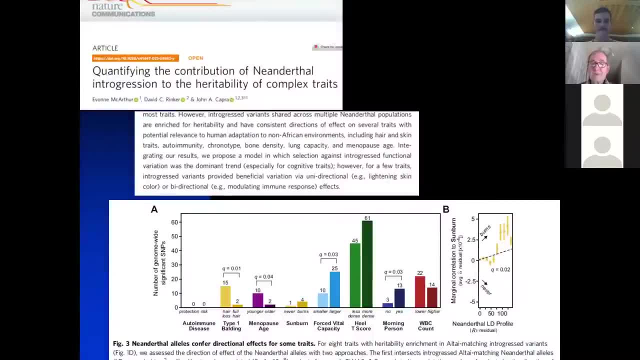 We separated 600,000 years ago. That was not long enough in our case to evolve complete reproductive isolation from the Neanderthals And of course some of that DNA is active in us today. And here's one nice one of many papers really that have been written about this activity of. 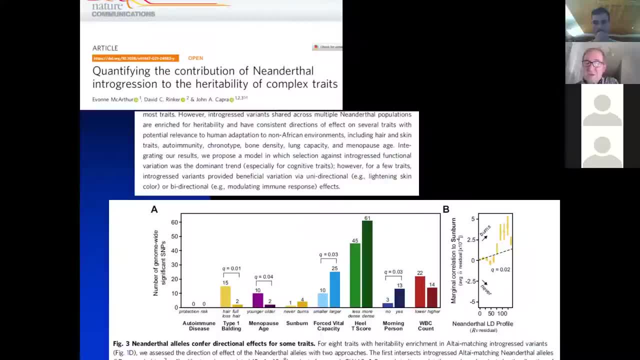 some of these bits of Neanderthal DNA in the genomes today. So, as you can see here, type one: balding, menopause, age, sunburn, susceptibility, force, vital, vital capacity, so lung power and so on. bone density. whether you're a morning, 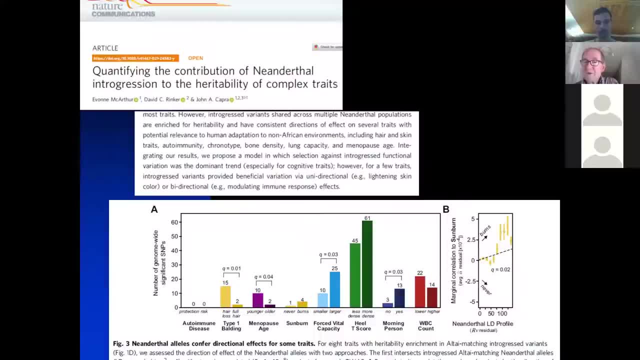 or an evening nighttime person, your white blood cell count. all of these seem to be influenced by the presence of particular bits of Neanderthal DNA. So some of this is certainly active today and our immune systems seem to show activity linked with Neanderthal DNA. 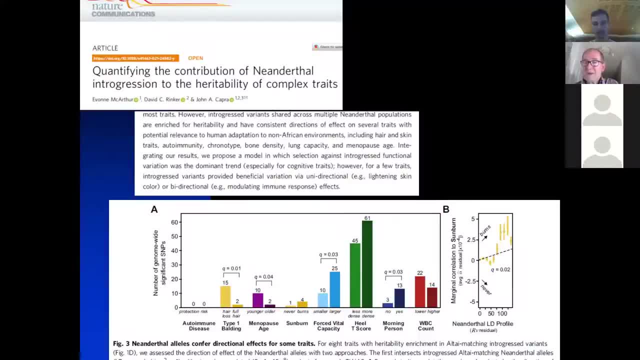 And that's not surprising, probably because, of course, coming out of Africa, we had no natural immunities to the diseases outside of Africa, whereas the Neanderthals had evolved natural immunities over hundreds of 1000s of years. So by interbreeding with them, we got a quick fix to our 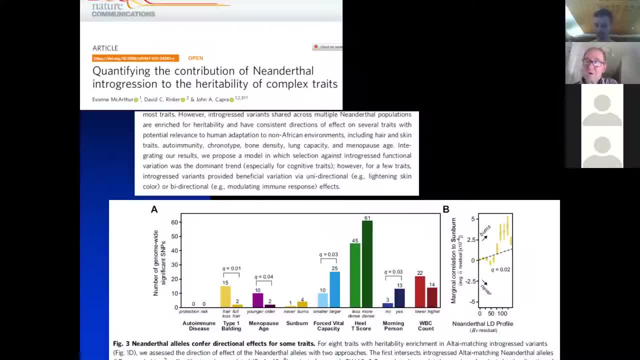 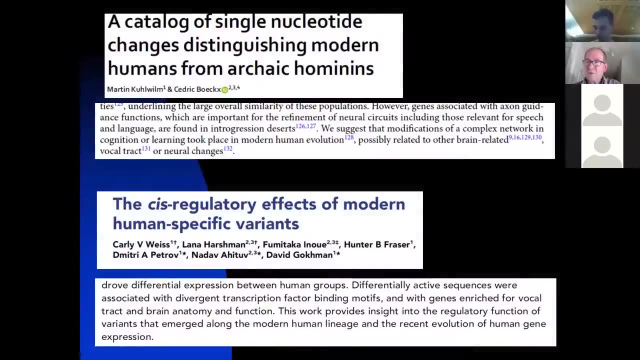 immune systems, And that was good news 40 or 50,000 years ago. Not such good news today, when there are some autoimmune conditions which again seem to be linked to the presence of Neanderthal DNA. What's also interesting is the bits of DNA that did not change, that we did not acquire from. 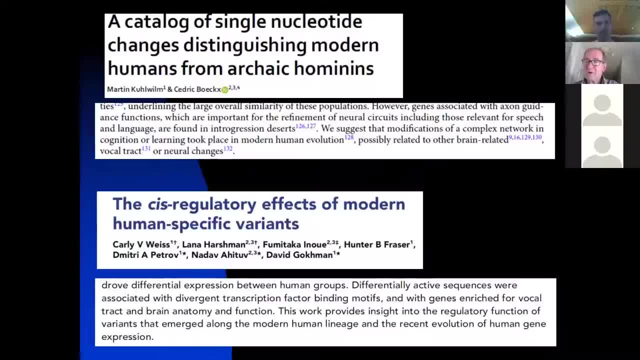 Neanderthals. So there are these so called deserts in our genomes today where you don't find any Neanderthal DNA. And so experts are looking, geneticists are looking at those deserts and looking at the genes in those deserts And, as it says here, genes which are important for the 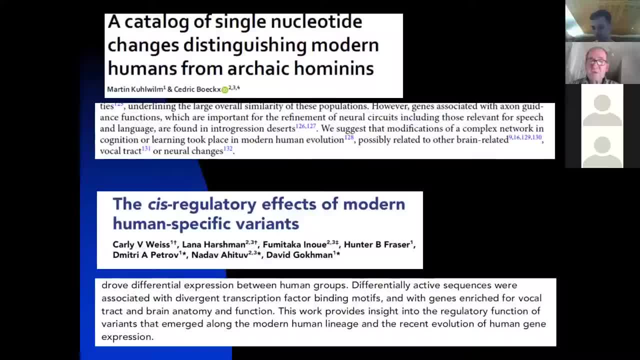 refinement of neural circuits, including those relevant for speech and language, are found in integration deserts. We suggest that modification of the neural circuits, including those relevant for speech and language, are found in integration deserts. We suggest that modification of the neural circuits, including those relevant for speech and language, are found in integration deserts. We suggest that modification. 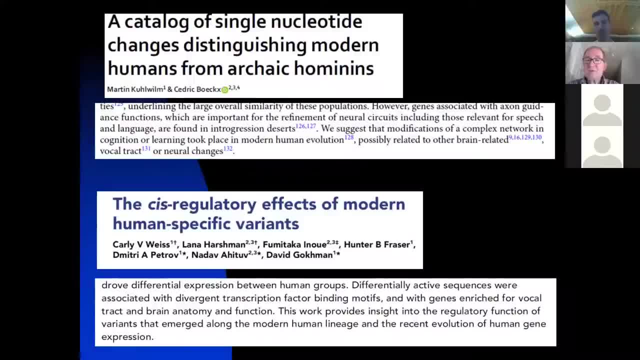 of a complex network in cognition or learning took place in modern human evolution, possibly related to other brain related, vocal tract or neural changes, And at the bottom there, experimental mapping of what some of these genes, which seem to be largely or totally unique to modern humans, are doing, So differentially active sequences are associated. 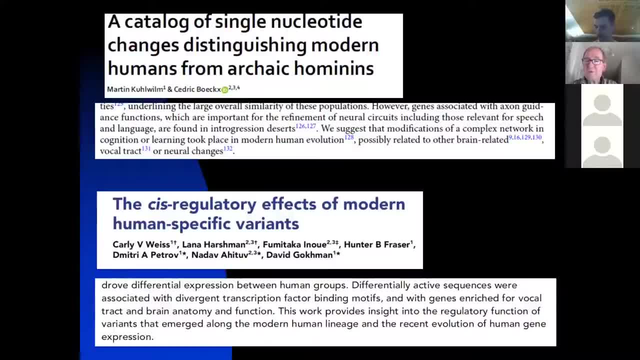 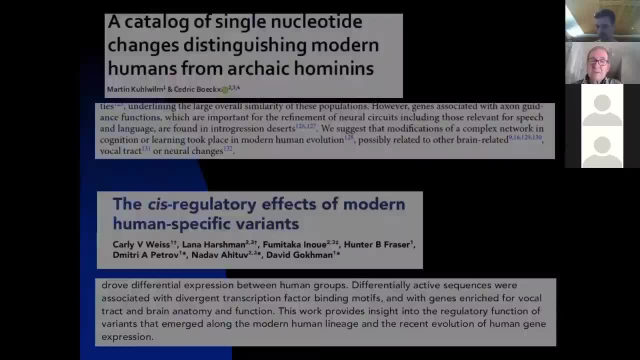 with divergent transcription factor, binding motives with genes enriched for vocal tract and brain anatomy and function. This work provides insight into the regulatory function of variants that emerged along the modern human lineage and the recent evolution of human gene expression. Okay, let's move on now to look briefly at the Denisovans who were in East Asia. So, of course, Denisova cave in southern Siberia, in the Altai region. Russian archaeologists have been digging this cave for more than 50 years and they had found some fragmentary human fossils, And although the teeth were very large, even Homo erectus size, it was very difficult to tell. 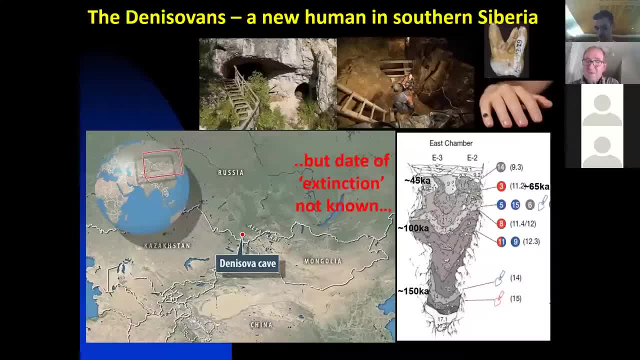 what kind of human they were. But of course, in the last 10 years or so those fossils have given up DNA And we now know that there was another kind of human living in this cave over a period of probably 150,000 or 200,000 years, that we could now call the Denisovans And the fragments that 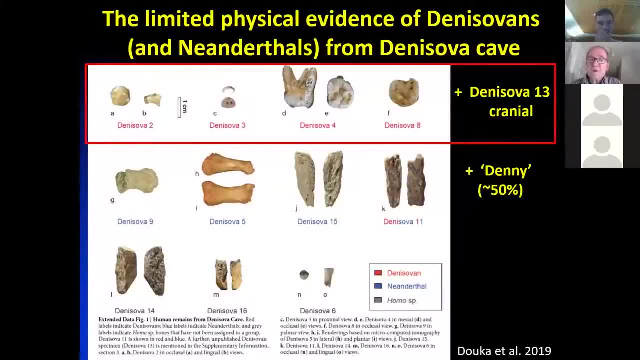 have given rise to this DNA are shown in the top of this diagram, Very fragmentary as you can see. there is one big tooth there, Denisova IV, And there's also some cronial remains not published yet, And these some of them have really high quality genomes. as good as you can get from. 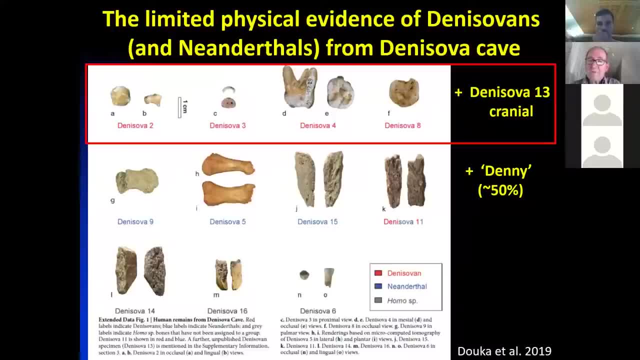 bones today. So remarkable preservation. And what's also interesting is that the cave also has Neanderthals in it. So these fragmentary remains in the lower part of this diagram are actually Neanderthal fragments and they produce Neanderthal DNA. 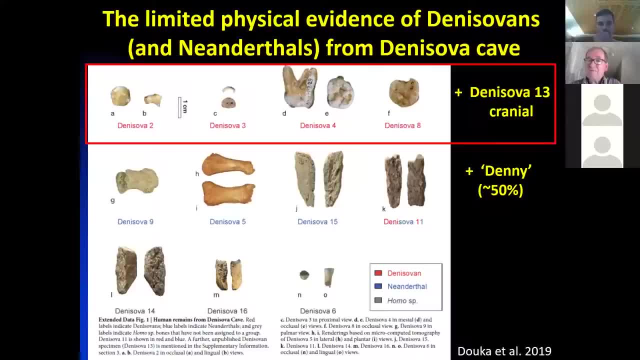 And, remarkably, Denisovan 11. there is actually, seemingly, a first generation hybrid of a Denisovan and a Neanderthal, So this is a girl who seems to have had a Neanderthal mother and a Denisovan father. She's been called Denny, So remarkable evidence. 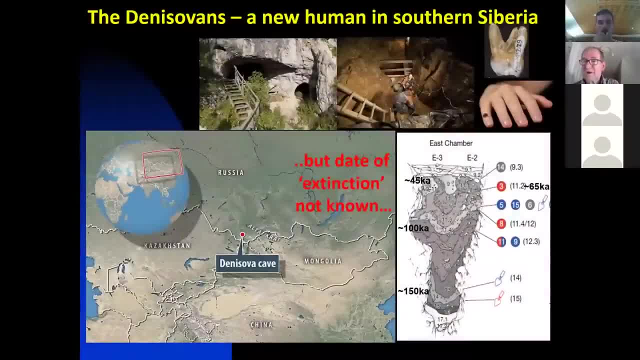 And if we go back to that previous diagram, you can see on the bottom right there the Denisovan fossils are mapped, I think, in grey and the Neanderthal fossils are mapped in red. So both these populations are there, alternating in occupation and even at times probably coexisting in this cave over tens or hundreds of thousands of years. 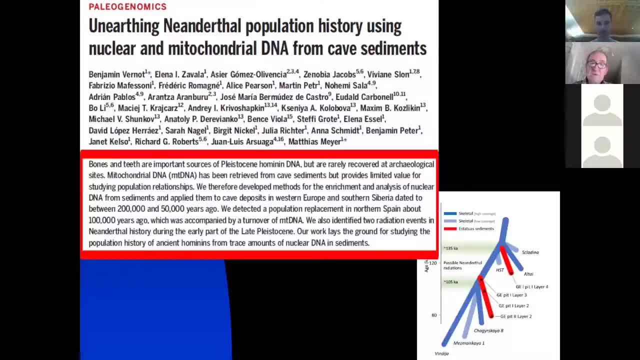 And we don't just need fossils now to get this ancient DNA. So here's a paper which looks at obtaining nuclear and mitochondrial DNA from cave sediments in Siberia and Spain, And so we now have the capability of getting both mitochondrial DNA and nuclear DNA. 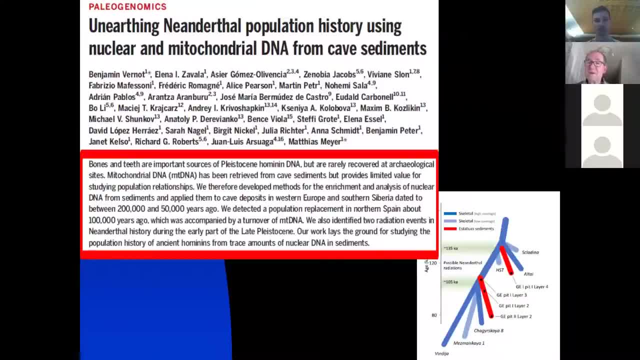 from the cave sediments. So if an ancient human has been in a cave and relieved themselves, if a woman has given birth in a cave, if an individual has died and pretty well all their physical remains has disappeared but genetic material persists, then DNA may be recoverable from the sediments. 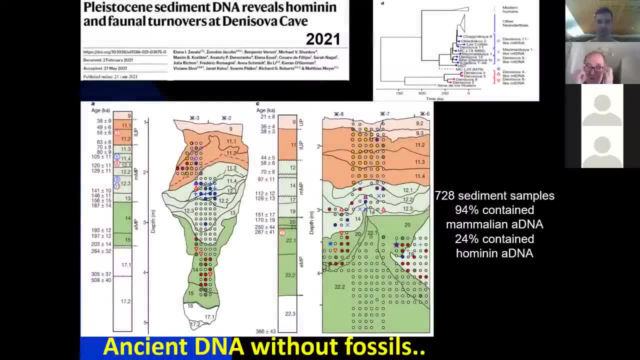 And that's what's happened at Denisovan Cave And again, this remarkable preservation of the site, due presumably to the cold conditions. So, as it says here, so these, these dots are, all you know, ancient DNA samples taken from the cave sediments at Denisovan Cave. 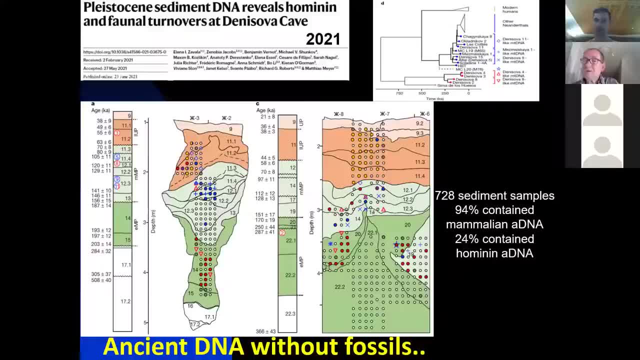 So, as it says here, 728 sediment samples, 94% of them contain mammalian ancient DNA, And that includes things like woolly rhinoceros and hyena and so on 24,. so nearly a quarter of them actually contain traces of hominin DNA. 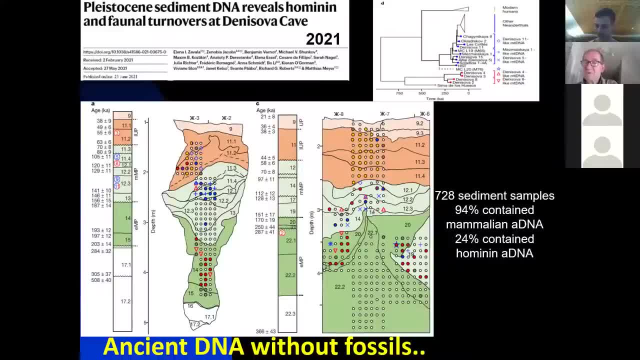 So from the cave sediments now we have even more Neanderthals, even more Denisovans And in the top of the sequence from about 45,000 years onwards, we have early Homo sapiens. So incredible data, And this is, of course, extremely important for future work, because it means that many cave sites 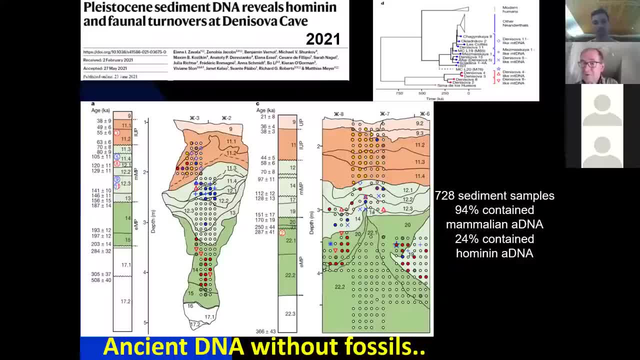 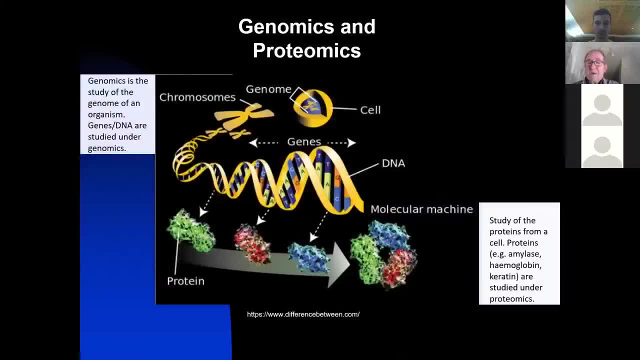 even without fossils, but with some archaeology showing ancient humans were there may have DNA in the cave sediments, And it's not just DNA that we can look for. So there's another area of work which is now developing and taking off, called proteomics. 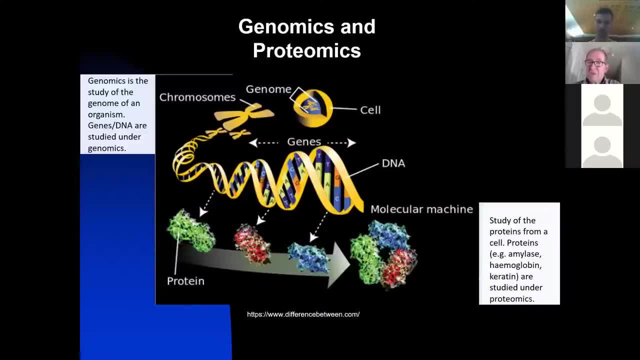 So, of course, as well as the DNA, which comes from the nucleus of the cell and from the mitochondria of the cell, we actually have fossil proteins, And these may have a longer preservation time than DNA. So there's a good possibility that we'll be able to recover fossil proteins from fossils, even though DNA has not been recovered. 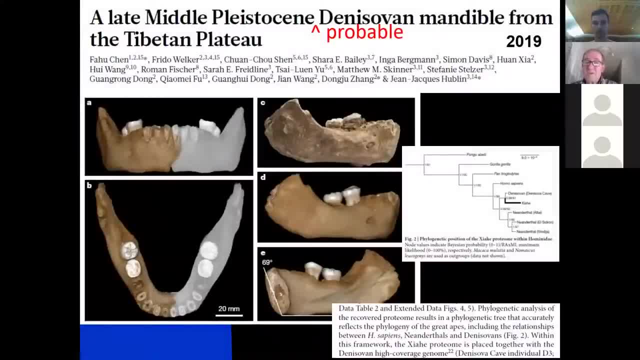 And that was the situation for this jawbone from the Tibetan Plateau of China, from Baixia Cave, or thought to be from Baixia Cave. this jawbone very robust, very big teeth which have been likened to the Denisovans, no chin on the lower jaw, dated over 150,000 years old by uranium series dating. 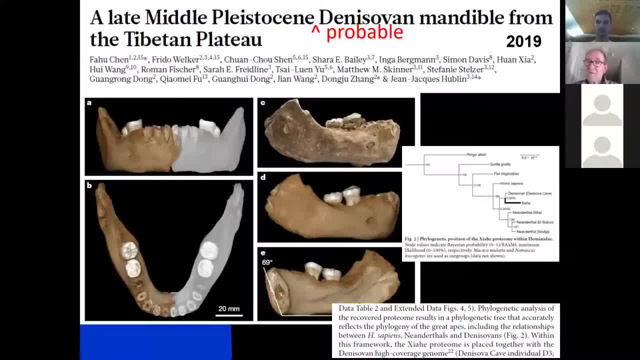 So DNA recovery was not possible, but they managed to recover a bit of fossil protein from it And that fossil protein mapped onto the Denisovans closer than it mapped to the Neanderthals and Homo sapiens. So this is a probable Denisovan fossil, over 150,000 years old, from the Tibetan Plateau of China. 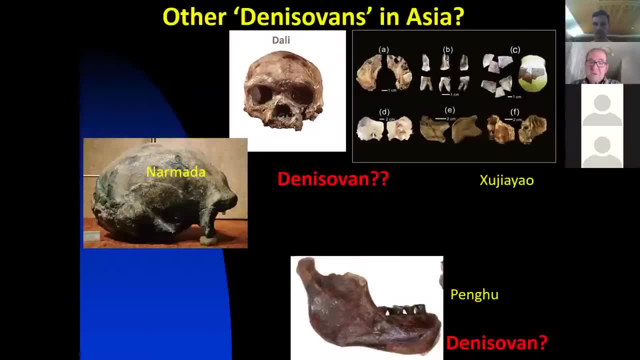 And there are a number of other fossils in the Far East and in India which could be Denisovans. This includes the Namada fossil from India, this jawbone from Penghu off the coast of Taiwan, fossils like Dali and Zujiaoyao. None of them have had their DNA sequenced yet. 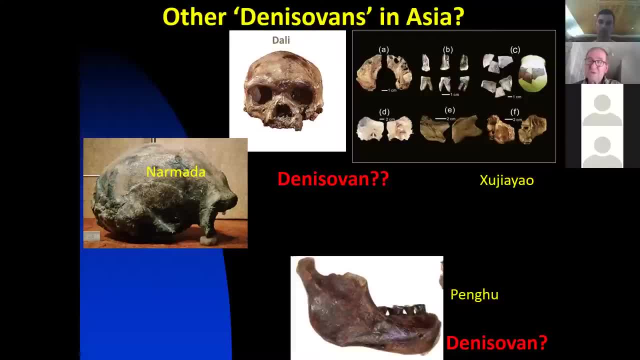 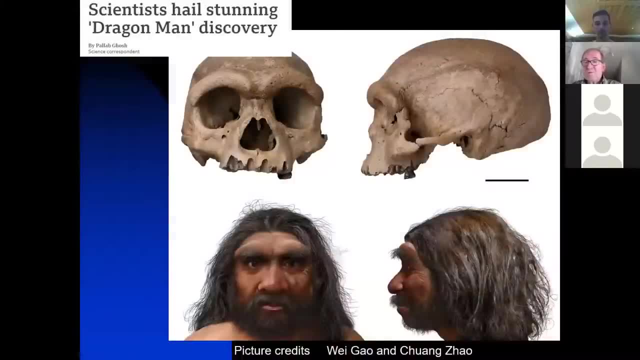 So we don't know whether they are Denisovans, but this is certainly something to be looked at And, equally, their proteins, their fossil proteins, could be investigated, And this is true for this beautiful fossil which I was involved in studying and publishing last year. 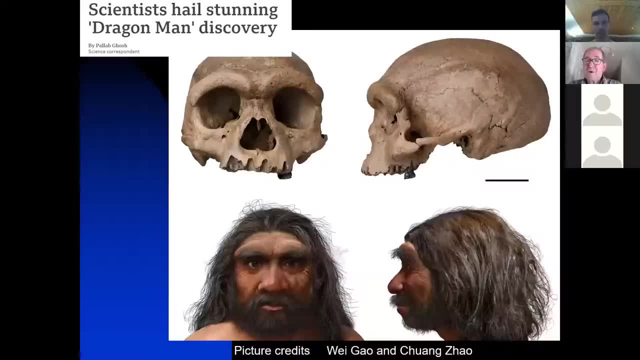 The so-called Dragon Man find from Harbin in northeastern China. So this fossil, very large, brained, archaic, features in the cranial vault long and low with a great big brow ridge, But the face looks much more like a Homo sapiens face. 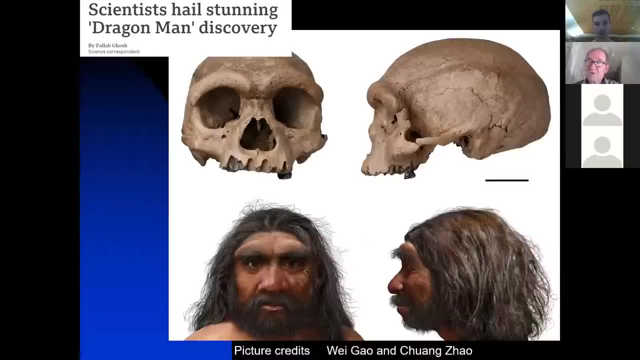 And there's only one tooth preserved in the upper jaw, one tooth left, But it's a massive molar, very like the ones from Denisovan cave. So again, this could be a Denisovan, more than 150,000 years old as well, in this case. 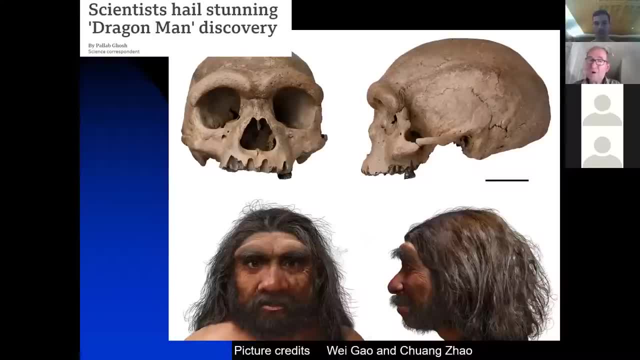 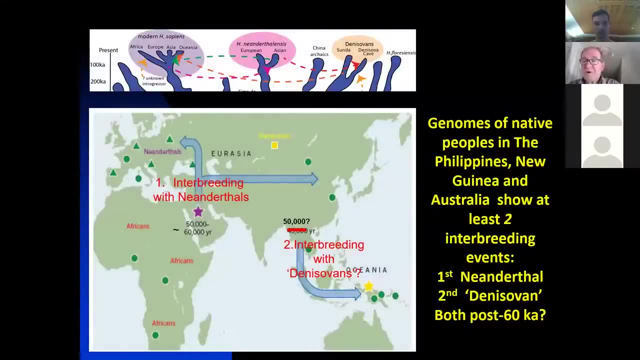 But until we have its DNA, we don't know. Until we have its DNA or its proteins, we can't be sure. And what's interesting, of course, is that Denisovan DNA isn't just found in Siberia or the Tibetan Plateau of China. 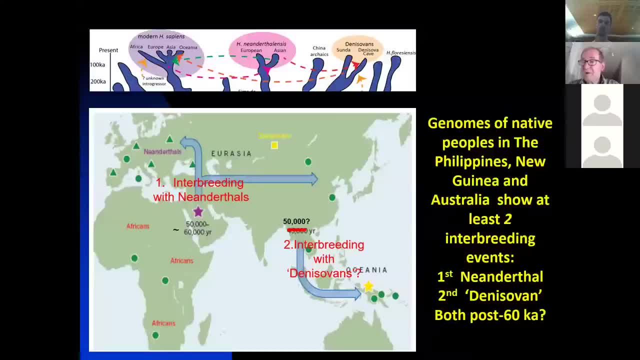 Because we find signs of interbreeding with Denisovans down in the islands of Southeast Asia particularly, and places like Australia, New Guinea and the Philippines. Now, the ancestors of modern Australian Aborigines, for example, have been Filipina people not thought to have gone anywhere near Siberia. 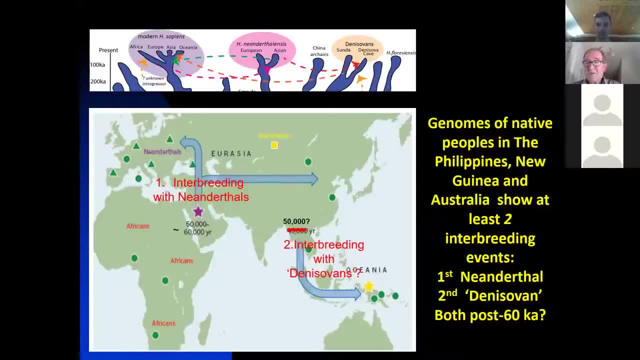 So the hypothesis is that this dispersal- maybe 60,000 years ago- of modern humans from Africa went through Western Asia And there was mixing with Neanderthals there. Then the populations moved from Southern Asia and down into Southeast Asia. 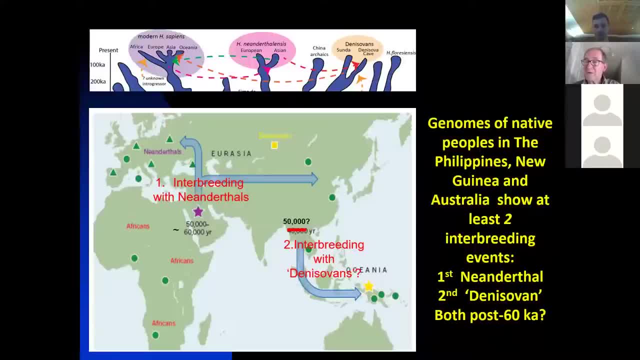 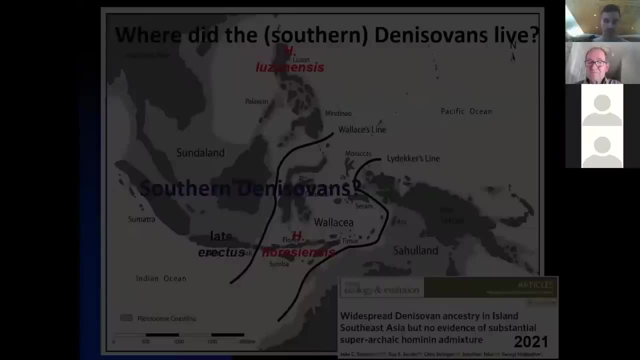 And it was down there that they interbred with a Denisovan-like population, which is why some of these individuals in Australia, New Guinea and the Philippines have up to 4% Denisovan DNA, As well as about 2% of Neanderthal DNA. 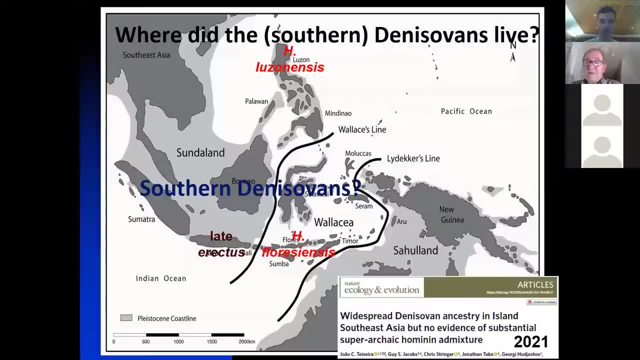 And where did those Southern Denisovans live that appear to have interbred with the ancestors of populations in New Guinea and Australia and the Philippines? Well, we think that Homo lucidensis was in the Philippines, Homo floresiensis was in Flores. 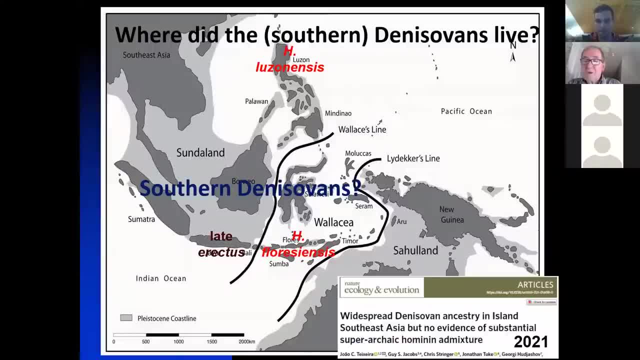 Homo erectus may still have been in Java. So my best bet, And that of some of the rest of us, is that these Southern Denisovans were living in places like Sumatra, Borneo and Sulawesi, And indeed there are artifacts on Sulawesi that are thought to be more than 150,000 years old. 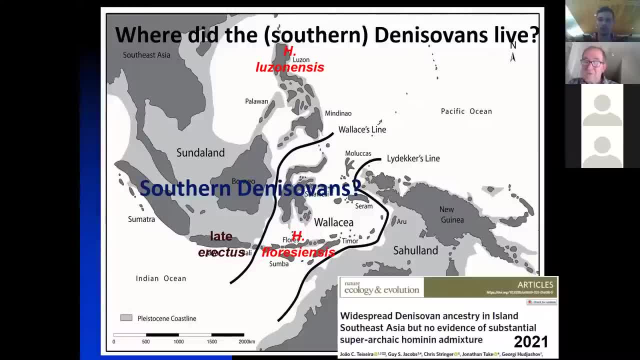 May well have been made by Denisovans, But until we have fossils, of course, down there which we can match with the ones from Denisovan Cave, it's going to be very difficult to map the presence of these Southern Denisovans down there. 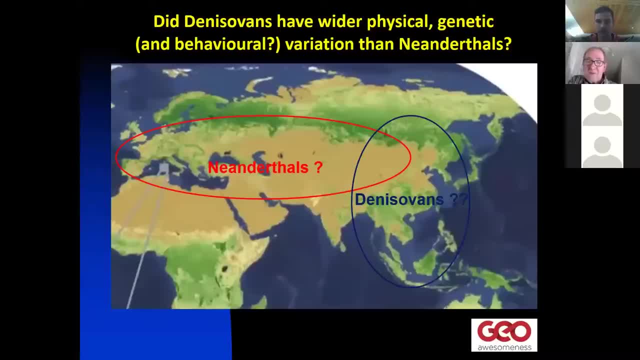 And possibly then this maps the range, Or both Neanderthals and Denisovans. So Neanderthals had an east-west range largely, Whereas Denisovans may well have had much more of a north-south range, ranging from the colder areas of Eastern Asia, Siberia and China down into the tropical and subtropical regions of Southeast Asia. 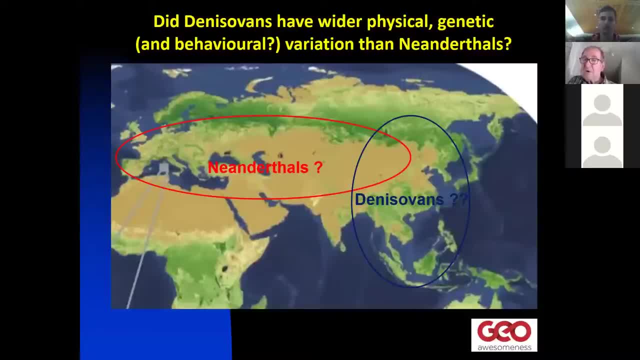 And on genetic data, it appears that the Denisovans are somewhat more varied genetically than the Neanderthals were. So a lot more to learn about these Denisovans, including, of course, their extinction date, Because the physical extinction of the Neanderthals we think we can map to around 40,000 years ago. 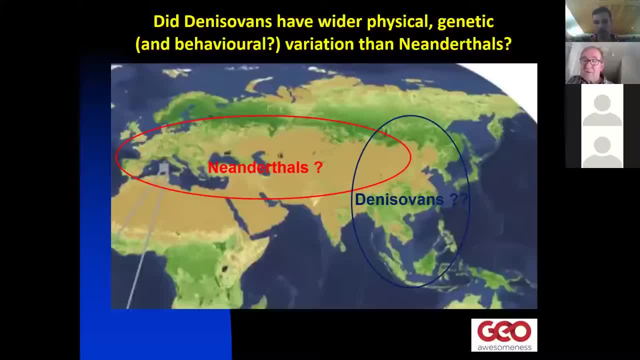 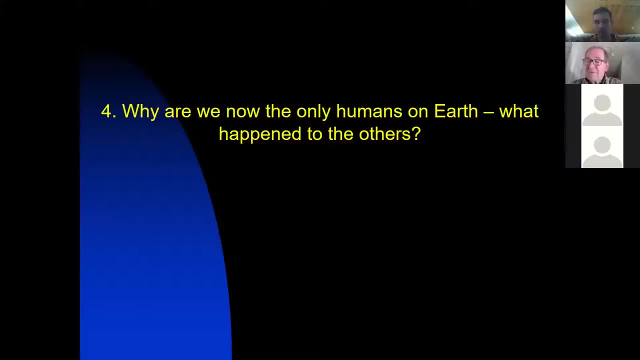 For the Denisovans. we have no idea how long they survived And some geneticists think that they could still have been around in Island, Southeast Asia, 30,000 years ago. So that last big question: why are we now the only humans on Earth, and what happened to the others? 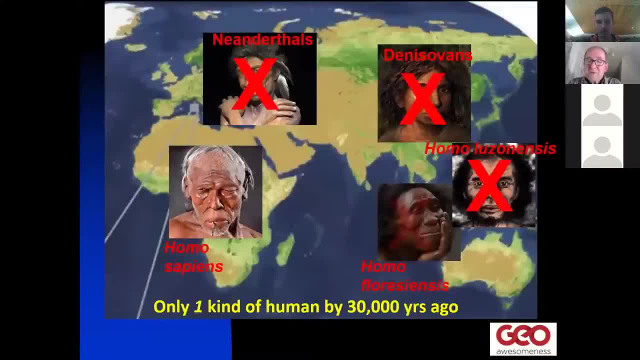 So these different kind of humans are all around at 70,000.. But by 30,000, we're not By 30,000. years ago, as far as we know, those other species had physically disappeared. Of course, genetically the Neanderthals and Denisovans did not disappear. 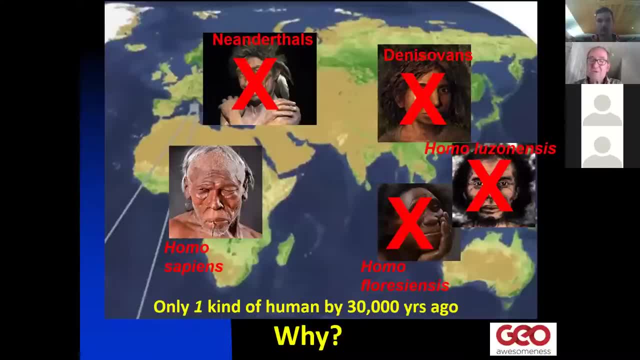 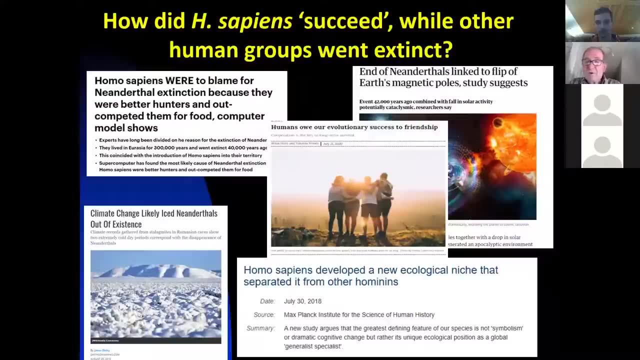 They live on. Some of their DNA lives on in us today. So why Well? I grabbed these from the popular literature and I'm sure you've got your own contributions to make to this debate. So top left there. Homo sapiens were to blame for Neanderthal extinction because they were better hunters and out-competed them for food. 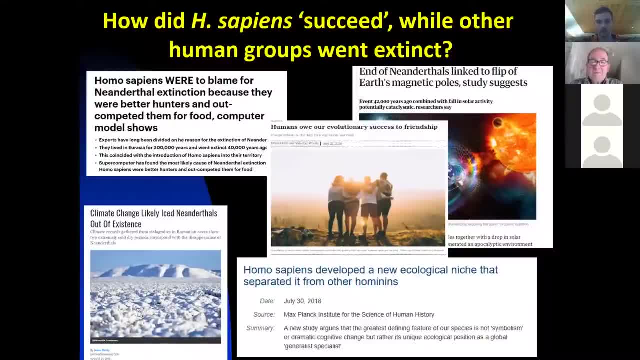 A computer model shows Bottom left there, climate change likely iced the Neanderthals out of existence. Two extremely cold dry periods correspond to the disappearance of the Neanderthals. Because the problem there is: if it was extremely cold for the Neanderthals, it would also have been extremely cold for early Homo sapiens. 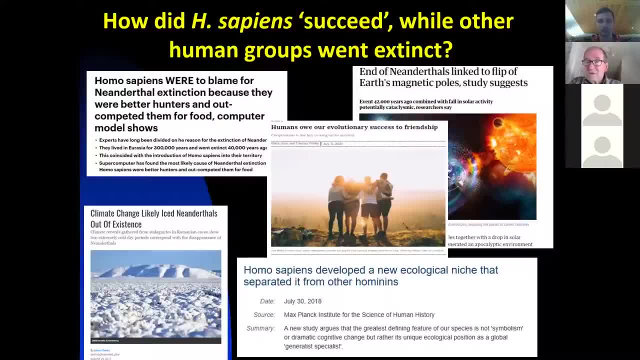 Top right there. one of the most recent ideas- the end of the Neanderthals- linked to a flip of the Earth's magnetic poles. a study suggests An event 42,000 years ago, Combined with the fall in solar activity, was potentially cataclysmic. researchers say. 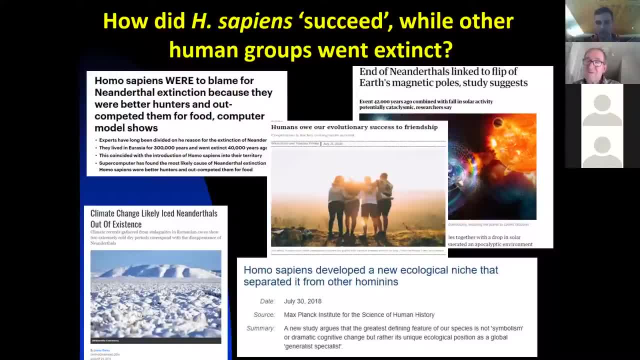 Well, again, the problem there is. you know, this does seem to have been a significant event, But of course it would have been significant for everything on the surface of the Earth and not just the Neanderthals. So I think this idea is overreached. 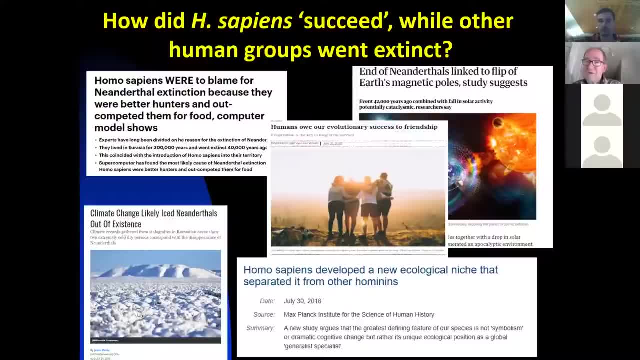 And we've written and published a reply to this paper critiquing some of the conclusions and the just over interpretation of the data. Bottom right there, Homo sapiens developed a new ecological niche that separated it from other hominins. A new study argues that the greatest defining feature of our species is not symbolism or dramatic cognitive change, but rather a unique ecological position. as a global generalist specialist, And in the center there, and quite a nice idea. humans are evolution's success to friendship. Cooperation was the key to our long term survival. So we may have had a lower level of evolution. We may have had a lower level of aggression within our groups, greater cooperation, greater networking between different populations, compared with these other humans. 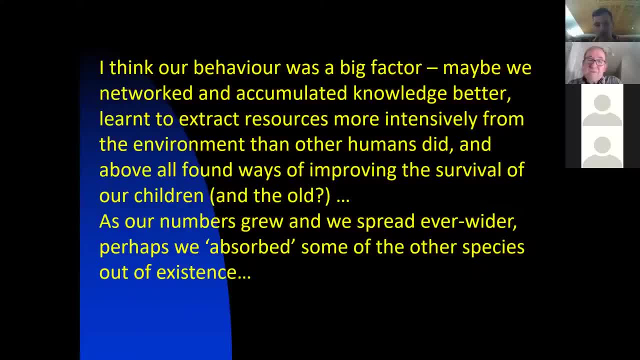 And my summary, my feeling at the moment. I think our behavior was a big factor, probably the biggest factor in our success. Maybe we networked and accumulated knowledge better, learned to extract resources more intensively from the environment than those other humans did. 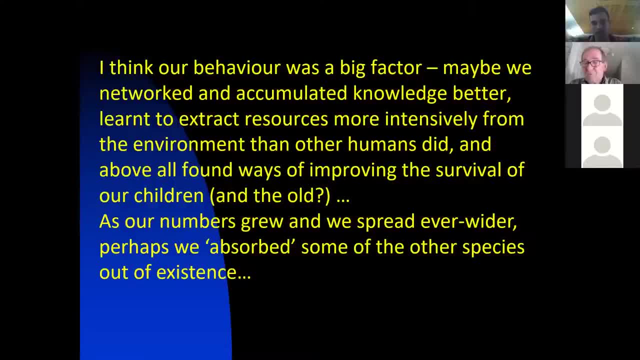 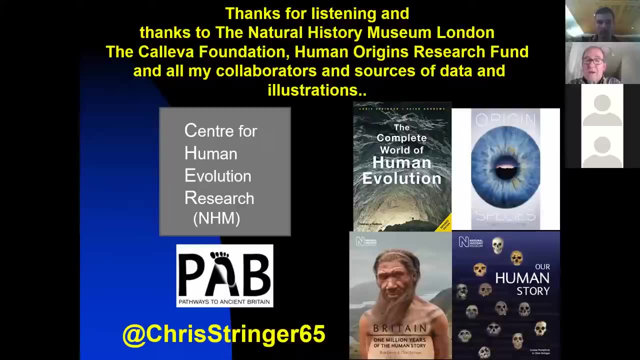 And, above all, found ways of improving the survival of our children and probably older people as well. As our numbers grew and we spread ever wider, perhaps we simply absorbed some of those other species out of existence. So thank you for listening, And I'd like to thank all the people who supported my research, all my collaborators and all my sources of data and illustrations. 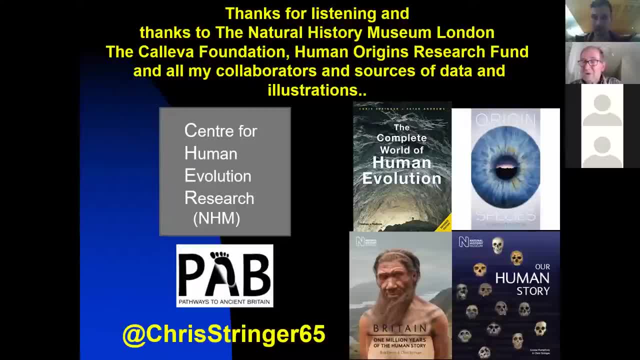 And there's some books you can read and there's a bit mentioned already, And if anyone's on Twitter, you can find me on Twitter with that handle. So, yeah, I'll stop there. Thanks very much. Many thanks for this talk, Chris. 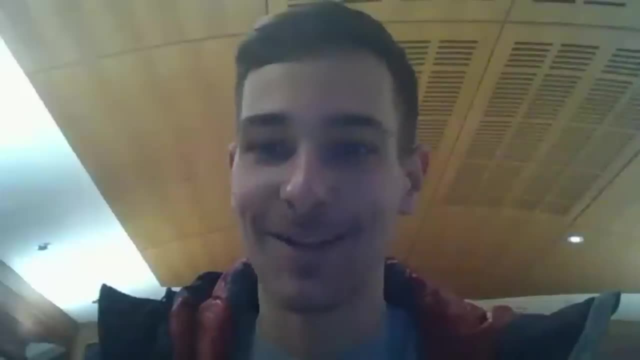 It was a really exciting one, As always. if anyone who is joining us with any questions, you can write them down in the chat and I will read them out loud, Or you can just raise your hand and ask your question directly. But yeah, before that, I will give you some time to think about your questions and start with my own ones. 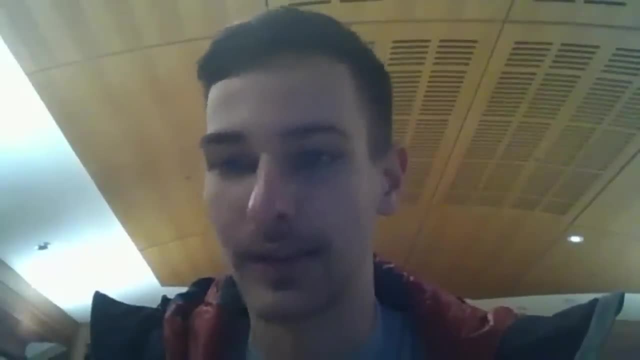 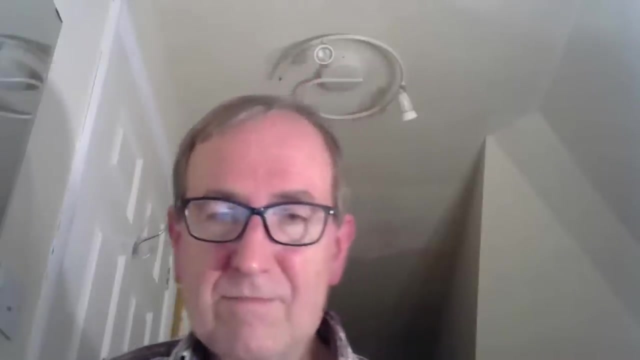 So, Chris, going back to the start of your talk, how widely, would you say, is now accepted that pan-African origin theory or hypothesis you were talking about? Well, I think, genetically, there's no doubt that we have a primary African origin. 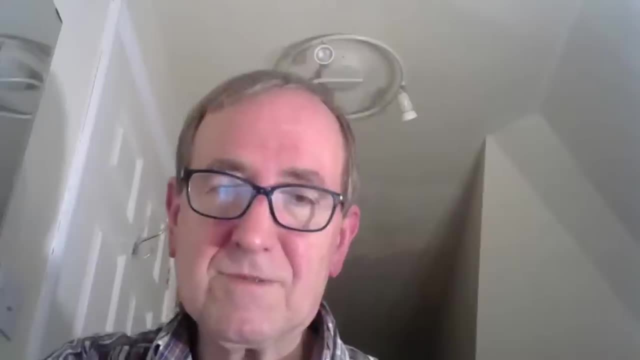 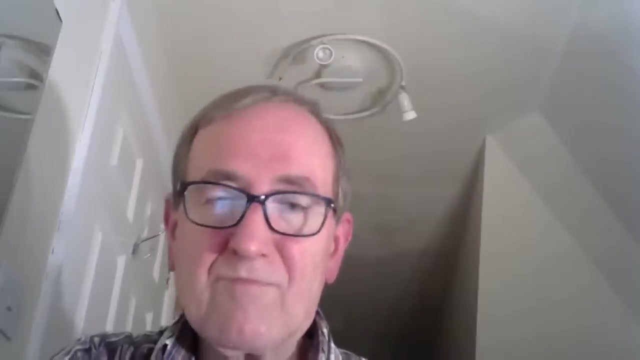 And I think what's happened is that it's no longer 100% recent African origin, And if I was giving this talk 15, 20 years ago, it would be 100%. 15, 20 years ago I would have said, yeah, we're pretty well, 100% recent African origin. 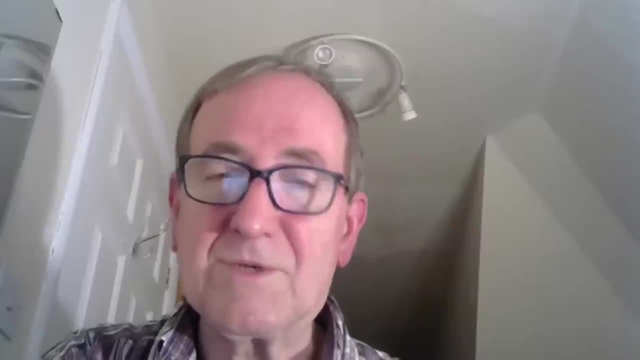 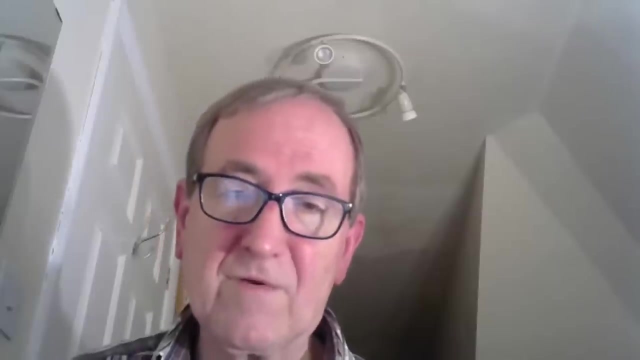 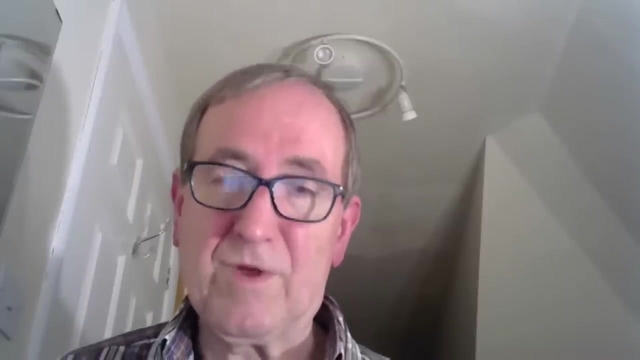 Now you'd have to say it's more than a 90% recent African origin, So it's not a complete recent African origin And this has led to a revival of this other idea of multiregional evolution. But I think what we've got is really modern humans coming out and mixing with those other species. 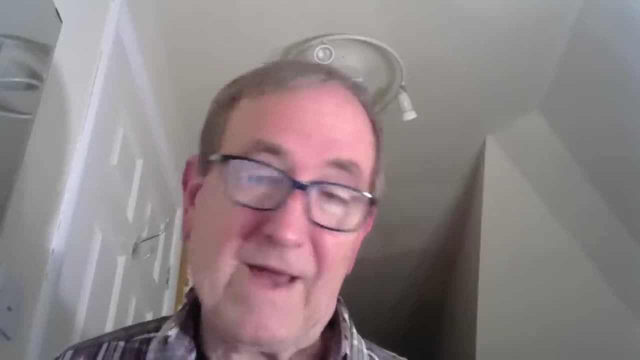 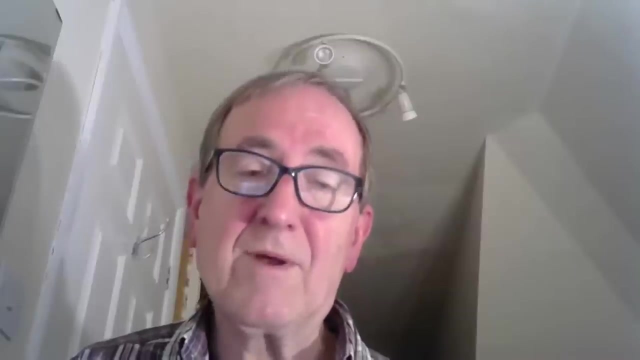 So I would call it out of Africa and hybridization mostly out of Africa. That's Fante Parbo's term for it. Now, mostly out of Africa. I think that's a good term. So we largely map our genetic and physical evolution back to African ancestors. 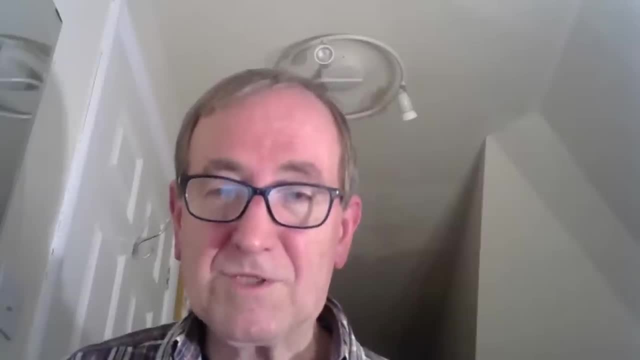 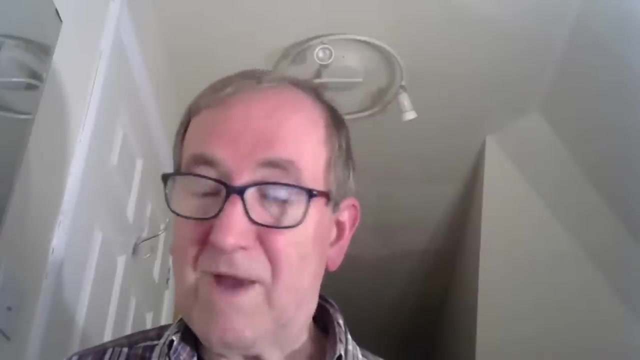 Behaviorally. that's obviously something for you archaeologists to think about. For me, I think it's less clear, But I would still say that most of our behavior probably maps back to Africa as well and its origins, And it remains to be seen how much we acquired behavior from these other species that we remember. 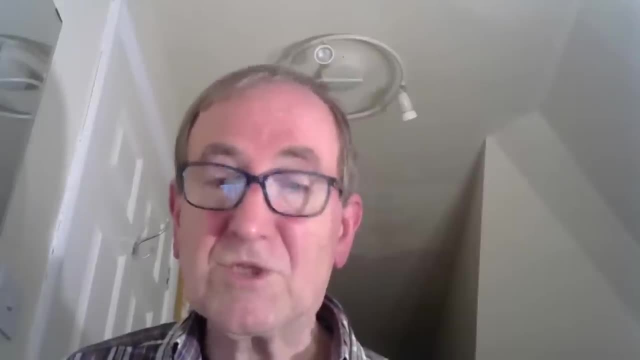 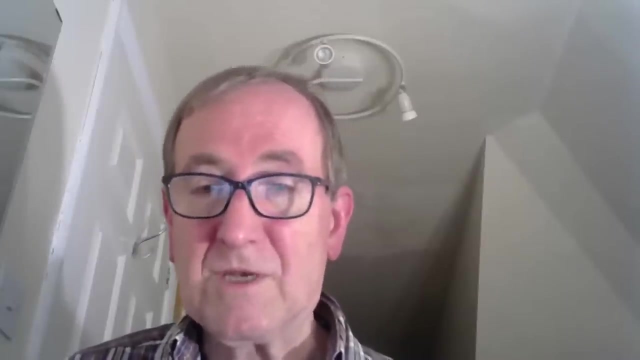 This is, of course, one of the most interesting things for the Neanderthal-modern human coexistence. There were certainly genetic exchanges going on. Neanderthals were joining modern human groups, So how much cultural exchange was going on in both directions. 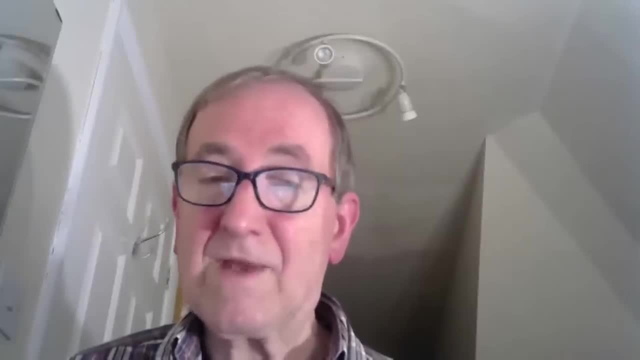 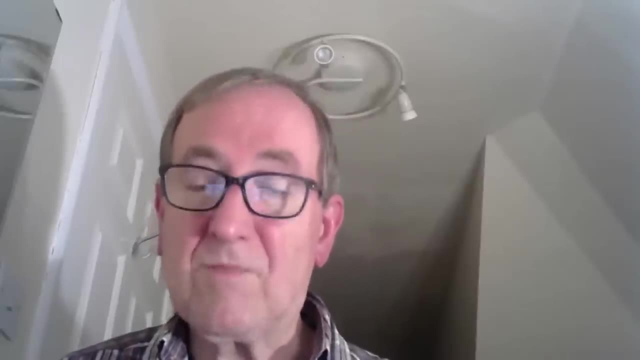 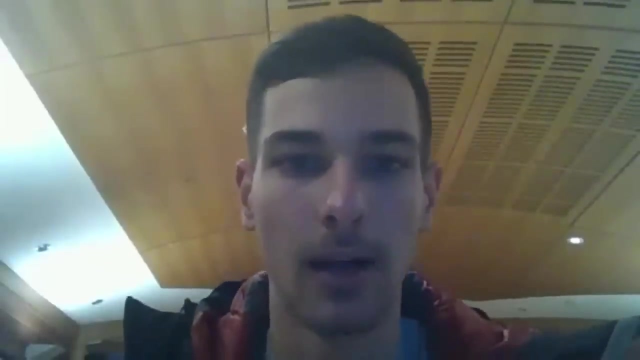 And for the Denisovans. we know obviously far less about that, But how much of that intermixture with the Denisovans was accompanied not only by gene flow but also by exchanges of cultural information, behavior. All right, Thank you. 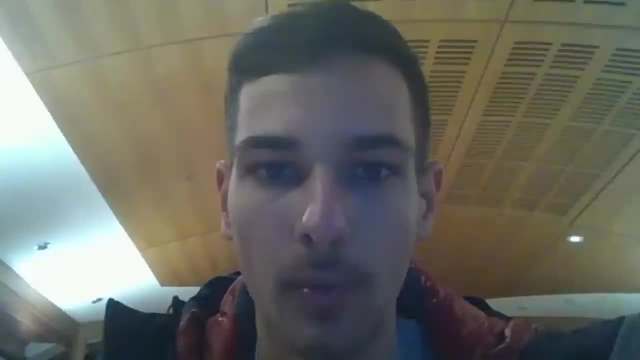 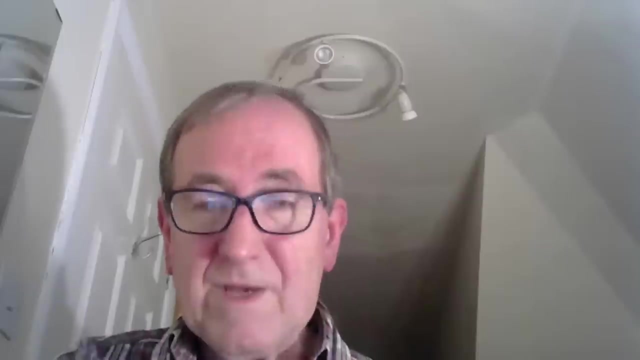 Gary is asking whether there are enough hominin fossils to make conclusions about early evolution. Yeah well, I would say in some areas there certainly aren't enough. So for Africa, I didn't get a chance to really pick up on one of those diagrams. 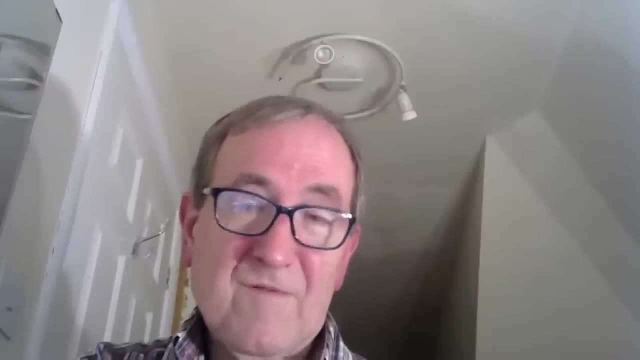 But our African fossil record, I would say, comes from less than 10% of the African population. So there are huge empty areas where we have no fossil evidence for ancient humans, even though we know they were there from stone tools. The Indian subcontinent, that vast area. 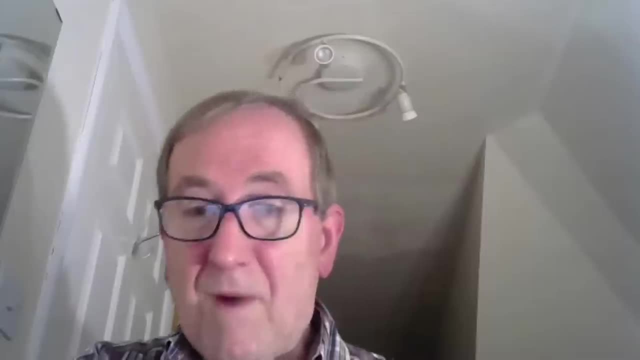 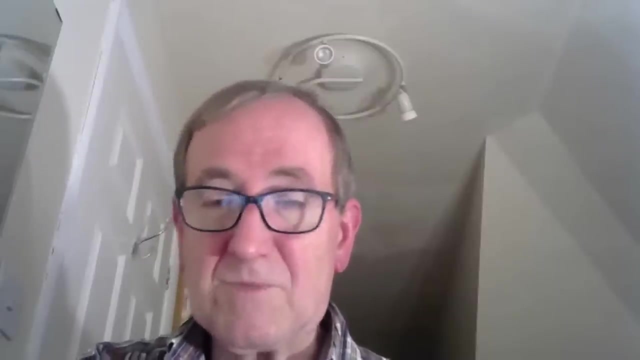 has only one significant ancient human fossil than a Marder fossil. So for some areas we still lack a lot of data. For Europe the situation is much better, But even there we can have surprises, as we've seen from the epidermal fossil. 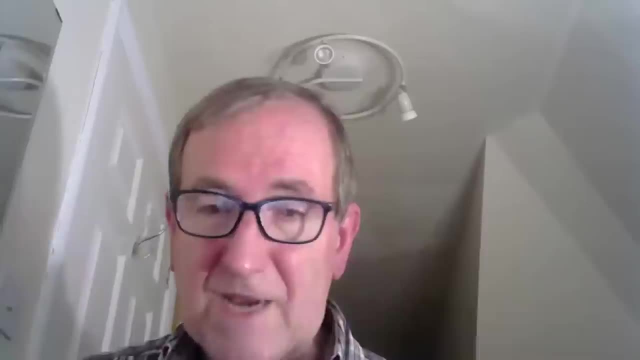 So I think in places, our data are pretty good. The genetic data, of course, are building up all the time, And the increase in genetic data is much faster than the growth of significant fossil data. So yeah, we build the scenarios we can. 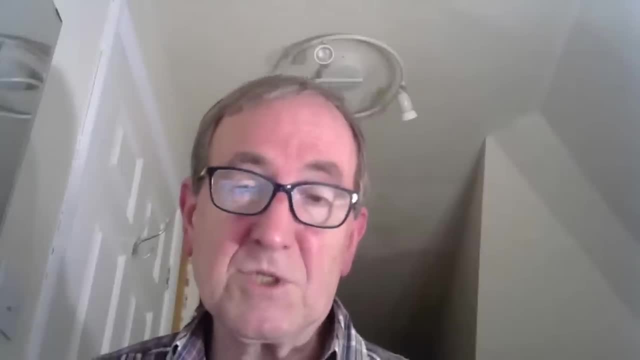 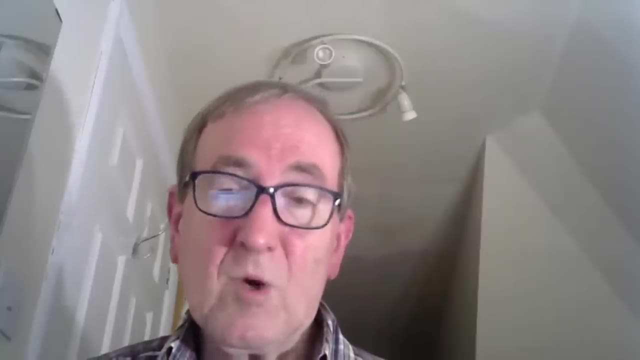 I've changed my views about things such as the position of Homo heidelbergensis as a common ancestor for us and the Neanderthals, And I would say I'm no longer sure who our common ancestor was. It might be there in the fossil record already, but not identified. 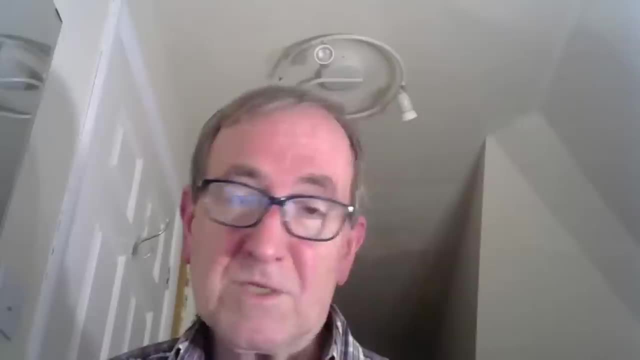 So, yeah, we have to work with what we've got. Something like Homo naledi comes along and provides us with a great surprise. Homo floresiensis was a huge surprise back in 2004.. So I think you know we build our model with greater confidence. 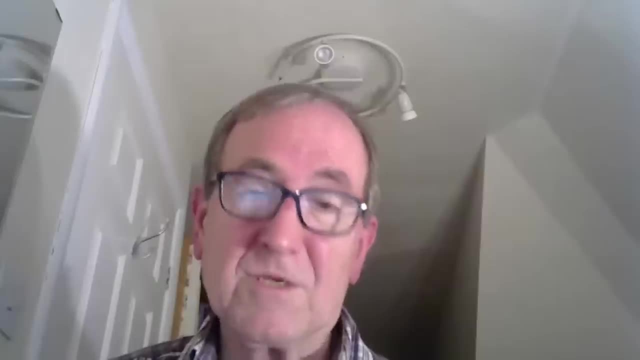 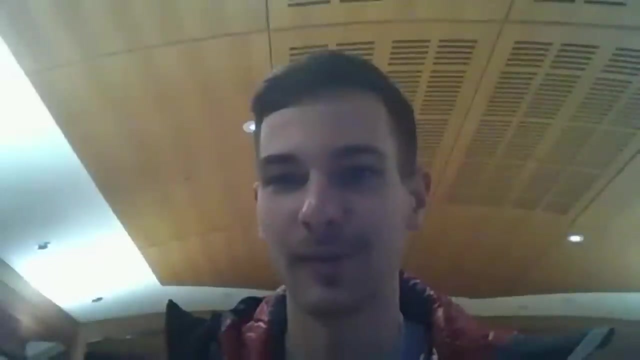 but with continuing caution, because, yes, we have to be aware there's still a lot we don't know about human evolution. I will give a bit of a follow up question on what you've just mentioned, And it's like recently there has been a study. 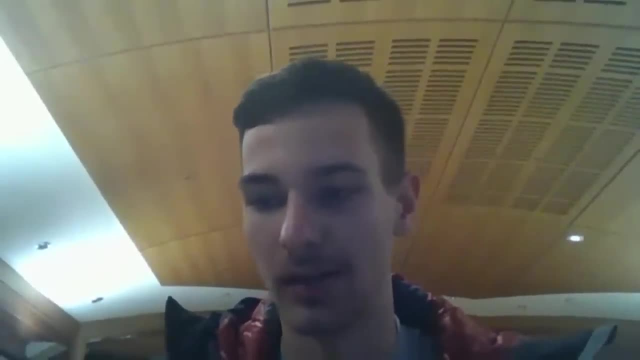 there have been, like many new human species being named or introduced based on- sometimes only on very partial evidence- I would say I don't know- mandible or part of skull. Can this be a problem for, or can it cause a problem in the future? 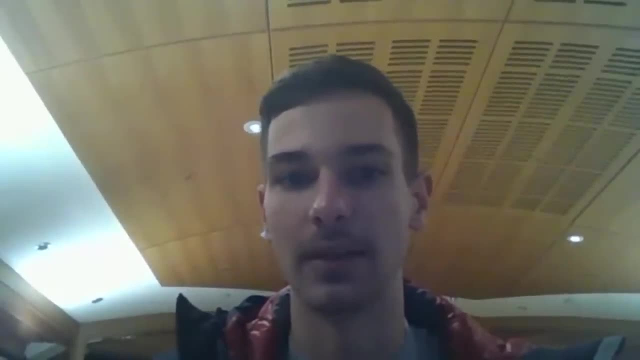 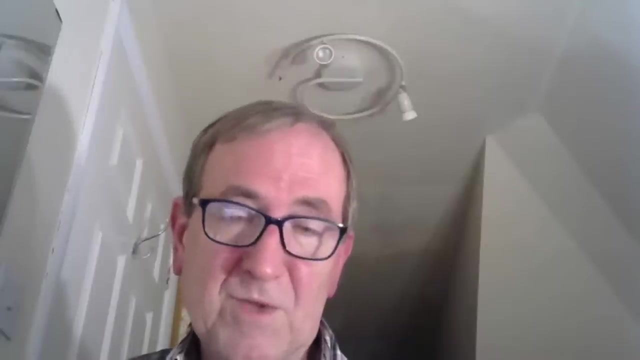 for archaeology and for developments in archaeology. Yes, I mean, certainly it is. It is a problem with the proliferation of species. How many of these are really good species, And when we get more data, will they be shown to be actually similar to other species? 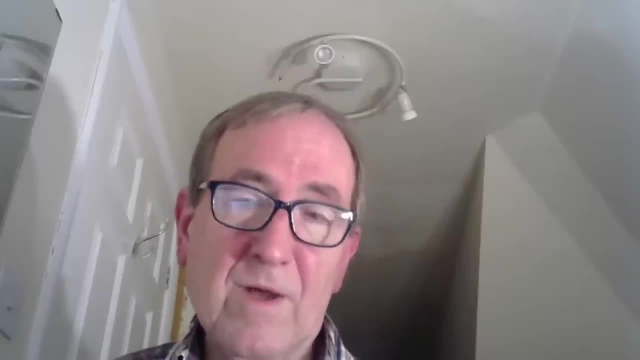 So Homo luzonensis is the case in point, really, where you've got quite fragmentary material and it does seem to be distinct. It's distinct from Homo floresiensis on the bits preserved, But when we have more material it might be that that will seem to be more similar to floresiensis. 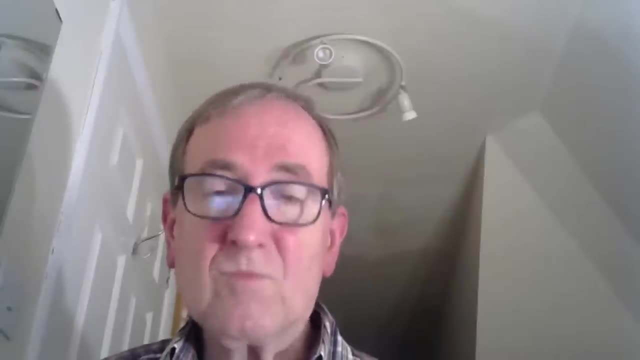 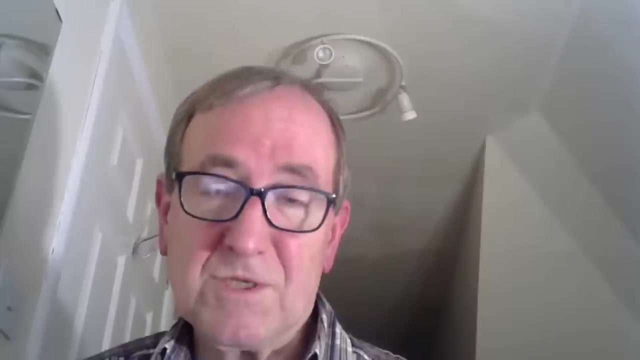 than it seems to be at the moment. For Neanderthals we've got a pretty good fossil record now And the Siemens de los Huesos material. you've got probably 29 individuals in the pit of the bones at Atapueca. 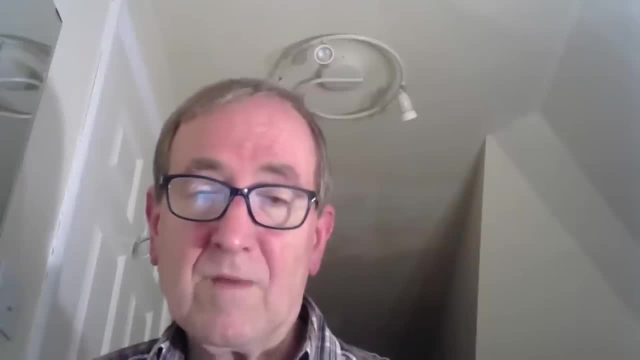 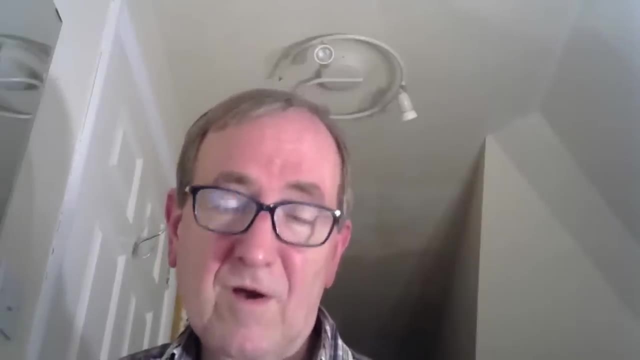 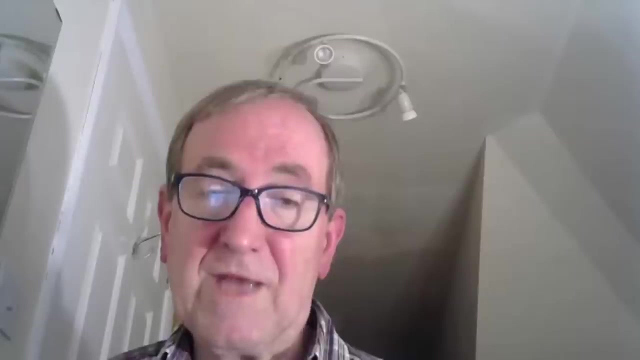 from about 430,000 years ago, Over 6,500 fossils. So it's a really good sample, And so we have a good idea, of that little window in time at least, of the diversity and the anatomy of those people. They seem to be morphologically Neanderthals. 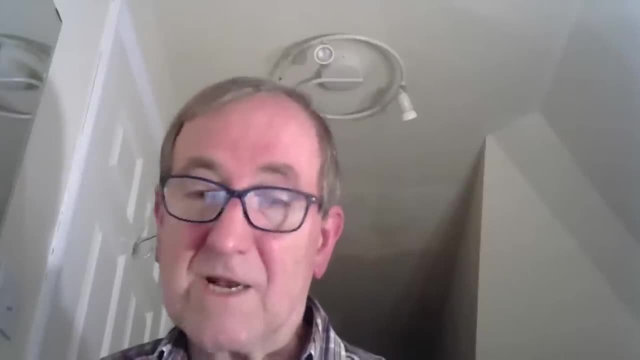 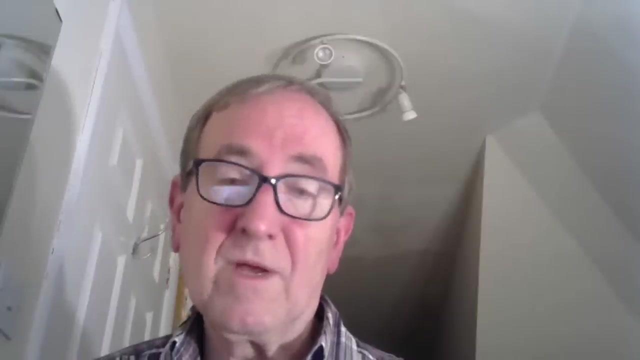 And of course they also seem to be genetically Neanderthals. So there's even DNA from the Siemens de los Huesos placing them on the Neanderthal lineage. So yeah, for some bits of the story I have reasonable confidence we're close to the truth. 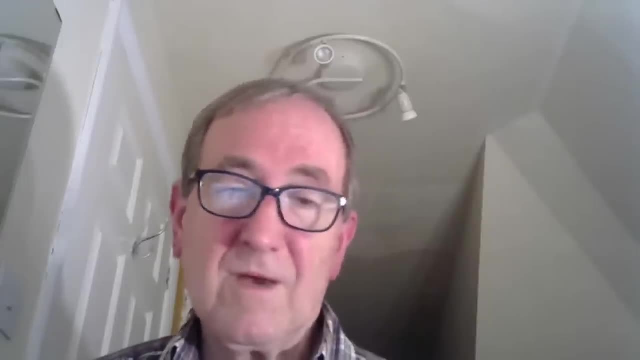 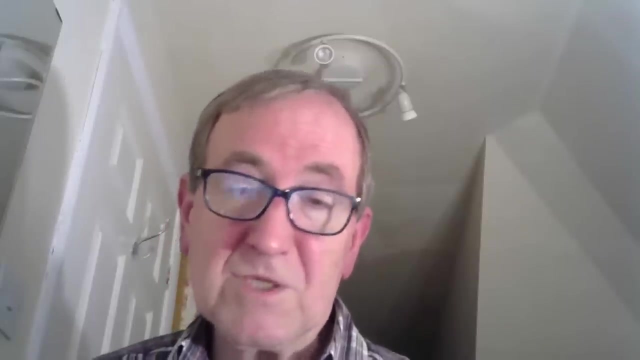 But for other areas, and certainly for the Denisovans- we're really only beginning to learn about them- And that whole area of Island, Southeast Asia. who knows how many other species might still be lurking there waiting to be discovered? Great Thank you. 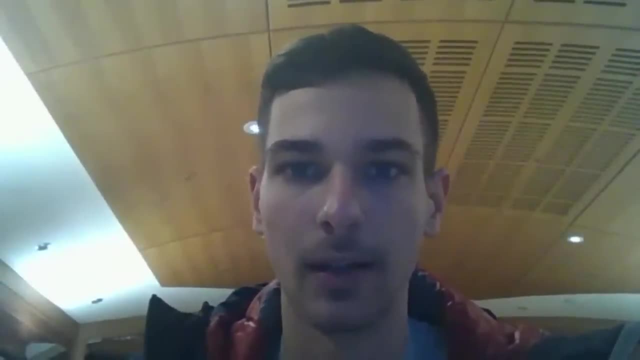 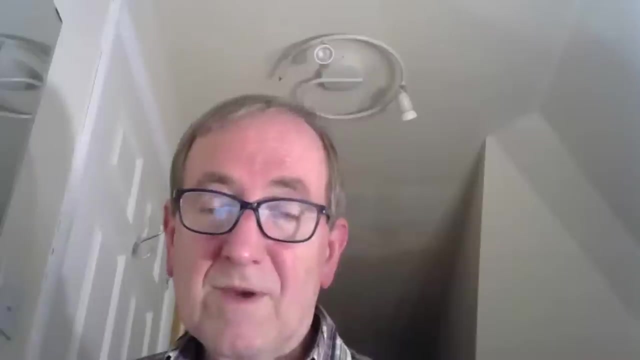 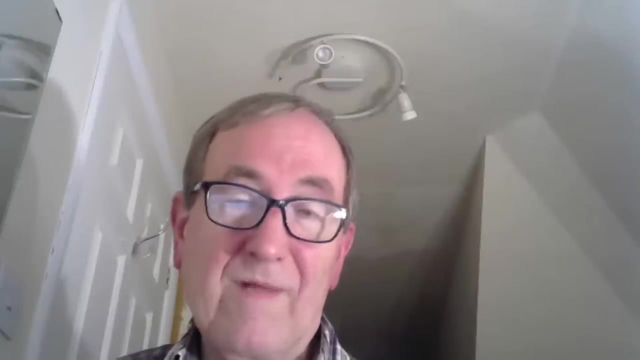 Sharon is asking whether you think that the melting of permafrost is likely to reveal any surprises. Yes, well, there certainly might be a Homo sapiens or two preserved up there in the permafrost. Whether the Neanderthals were ever up there. 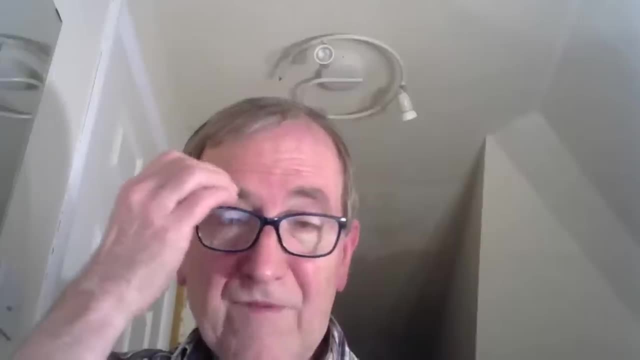 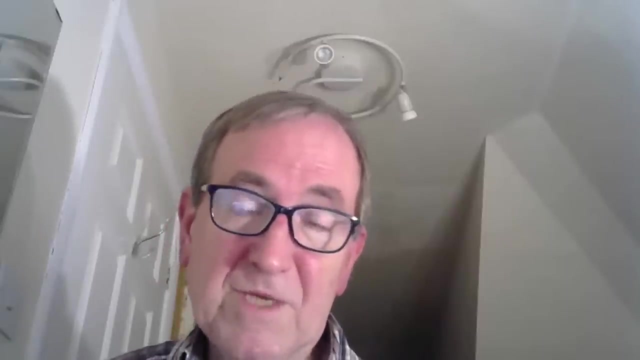 I think that's much less likely. I think probably for Neanderthals there's more hope maybe, of finding a Neanderthal in a peat bog. So, for example, we've got preserved peat deposits from the last interglacial in Europe. 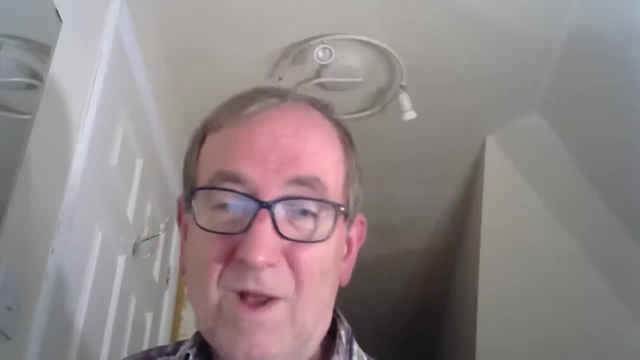 And who knows, Maybe a Neanderthal fell in there once and we might one day find the body. So you know, it's always: you never say never. There have been remarkable finds from permafrost and from, of course, melting glaciers, in the Alps, for example. 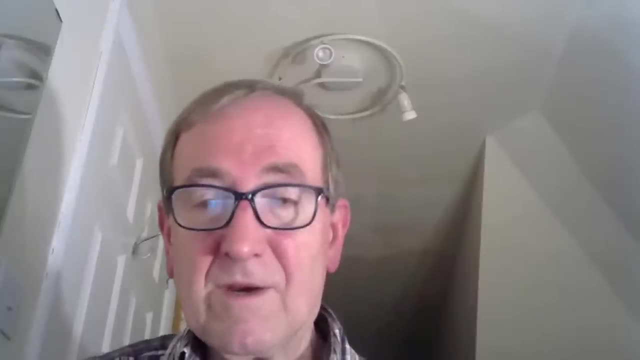 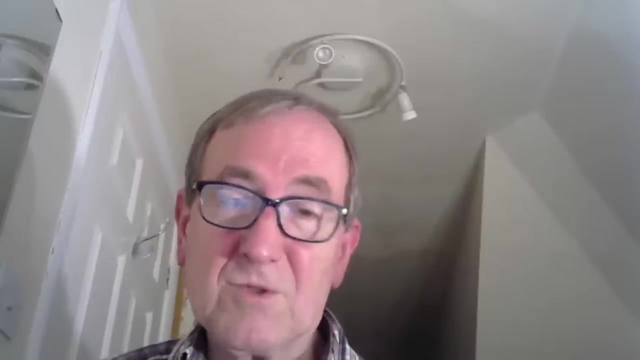 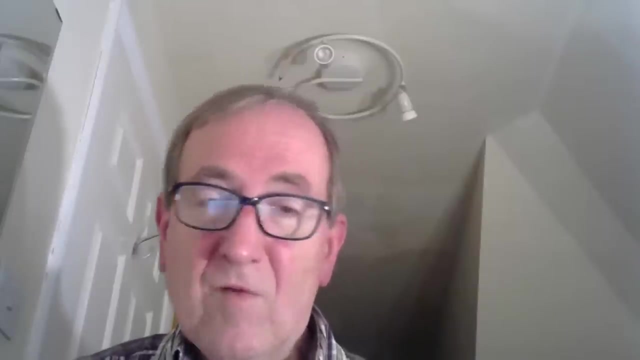 Think of Otzi found in the Alps. So maybe we will have tissue preservation of the Neanderthals or Denisovans one day. It will be wonderful, because if we do, but the DNA itself is obviously very, very helpful And more and more can be drawn out from that DNA data. 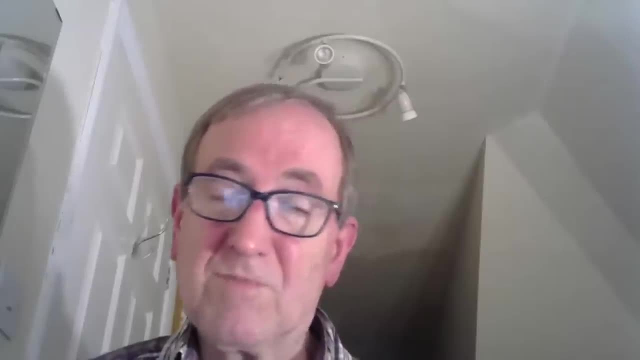 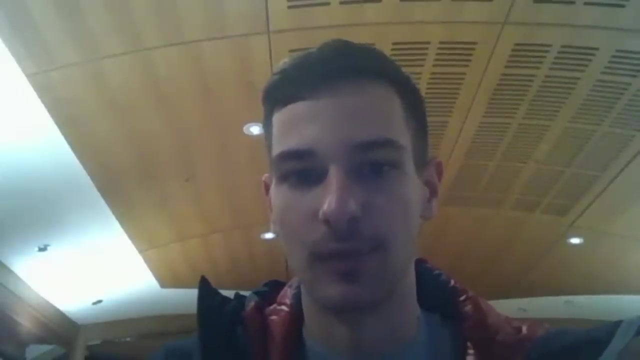 as I was showing from some of those studies of the intergressed bits of DNA and what they were doing, probably in Neanderthals compared with us. So if we would have some of this DNA preserved of other species which we don't have for now. 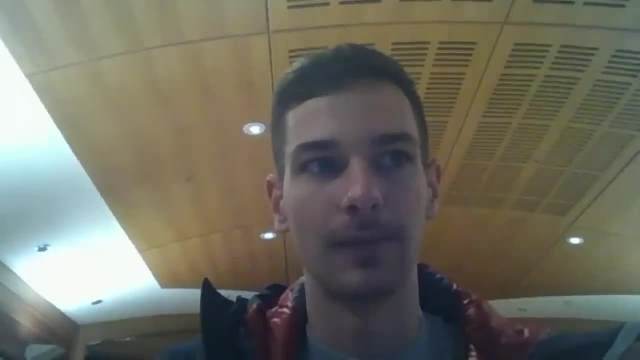 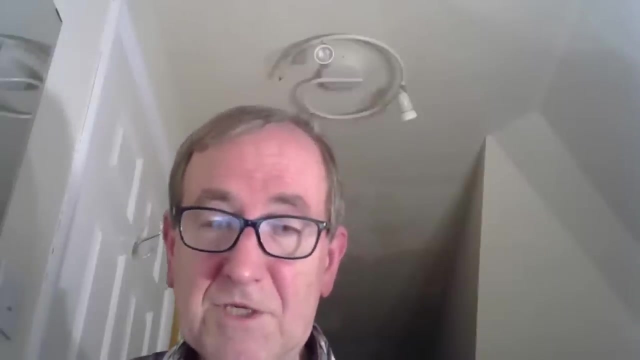 would it be possible to trace whether we have still some parts of the DNA present in ourselves today or, as it is possible, with Neanderthals, or not really? Yes, So I was on a paper which attempted to test in Ireland, Southeast Asia. 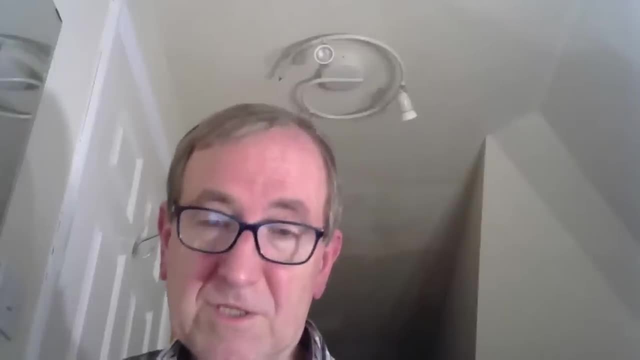 whether there was evidence of these other species in the DNA. So we've got Denisovan DNA represented at the level of about 4% in some of those populations. So we all tested whether there. we tested whether there might be very, very small amounts of distinct archaic. 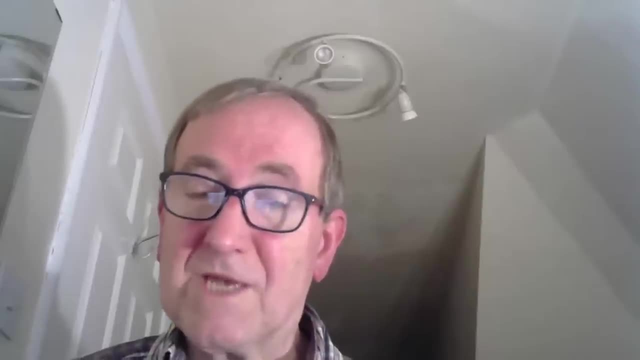 so-called archaic DNA that might be coming from, let's say, Floresiensis or Lusinensis or Homo erectus, And we couldn't find any trace of it in the samples we had. and with the resolution we had, Now, that's not to say there couldn't be a little bit of it there. 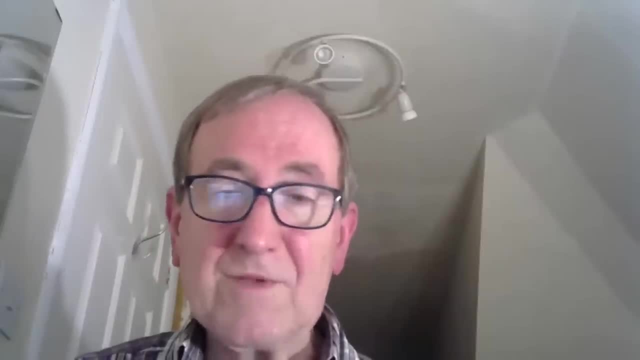 and we weren't able to pick it up. So it's possible there will be others And in Africa there's certainly some data that Africans too have introgression from archaic humans in sub-Saharan Africa. So possibly this is from Hydrobigensis rhodesiensis. 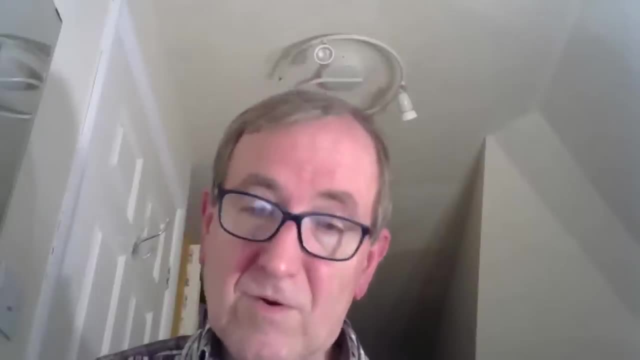 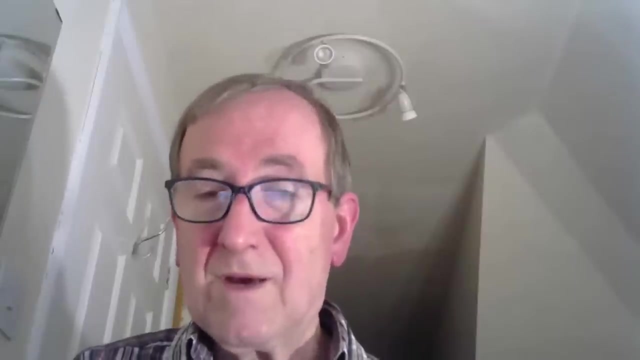 possibly even from Homo naledi, Who knows? So there are traces of archaic DNA there, But because, as I mentioned of the African conditions, we don't have a genome of one of those ancient African humans to compare, to really map where it's coming from. 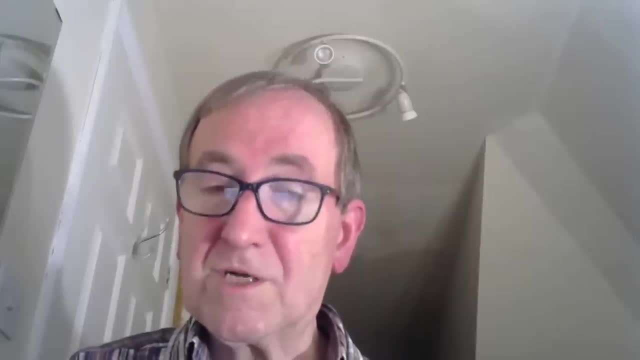 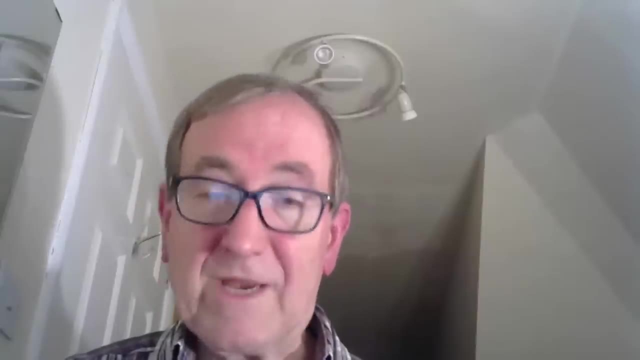 So we don't have the equivalent of a Neanderthal or a Denisovan genome in Africa that can tell us the source. We don't have the equivalent of this putative introgressed DNA, But it looks like it is there, And so African populations, too, may have a similar level. 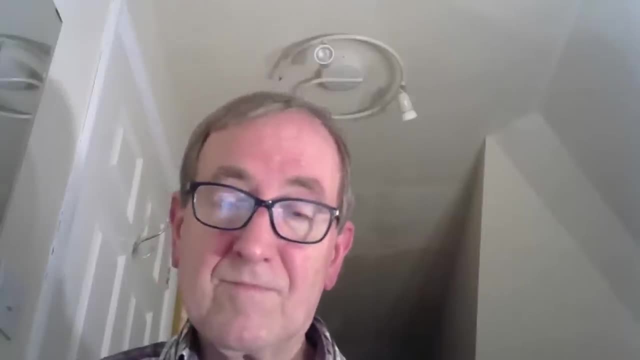 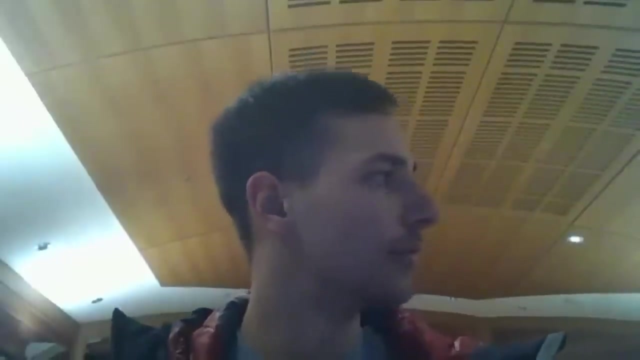 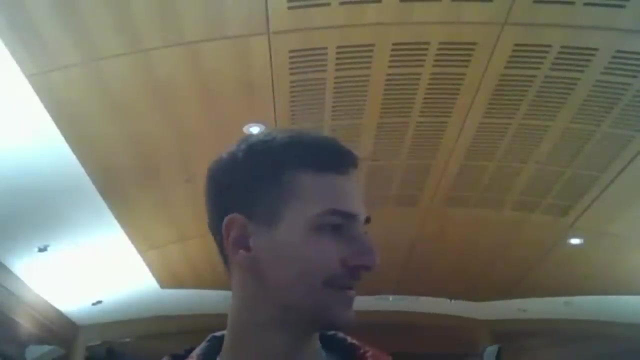 of what can be called archaic DNA, not yet well mapped. All right, Thank you. Are there any other questions? Do you have Just come in here and you can ask it yourself. Thank you so much for the talk. I just wanted to ask you your hypothesis about behavioral reasons. 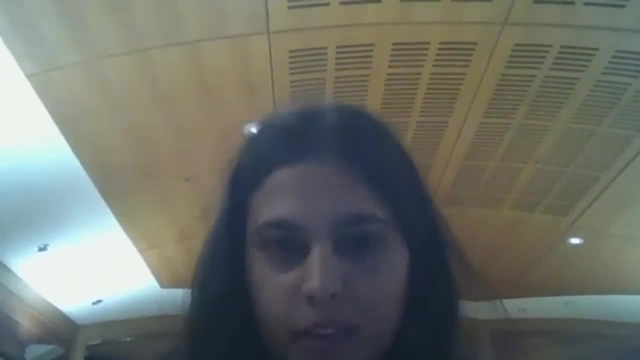 for us being the only species left in present times. Would you suggest any ways to gain more clarity on what exactly this behavior might have been, Maybe something we can observe in the archaeological record, what we can look out for when we are trying to understand? 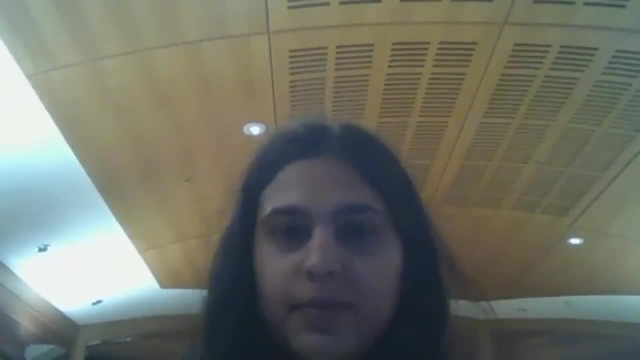 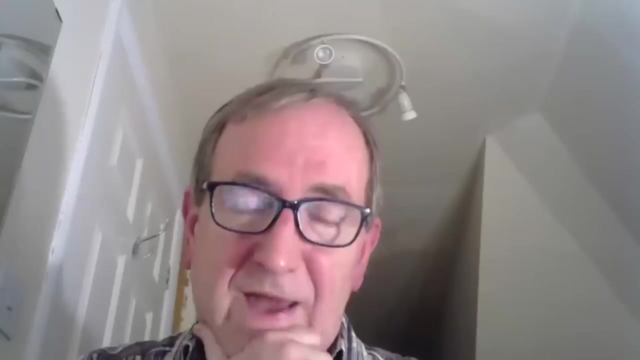 why we were the only ones left. Yeah, I think that's a very good question. I mean, I don't have the answer to why we're the only ones left. I think for the Neanderthals and us we can map the disappearance of Neanderthals pretty well. 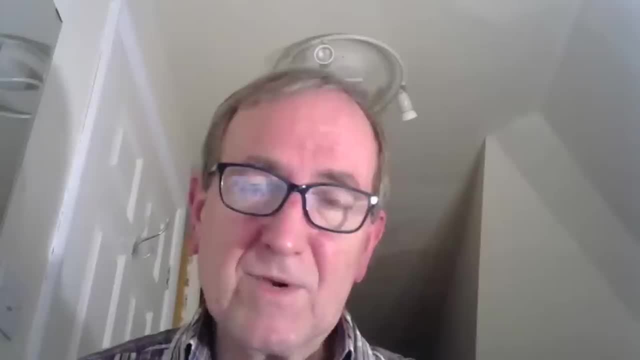 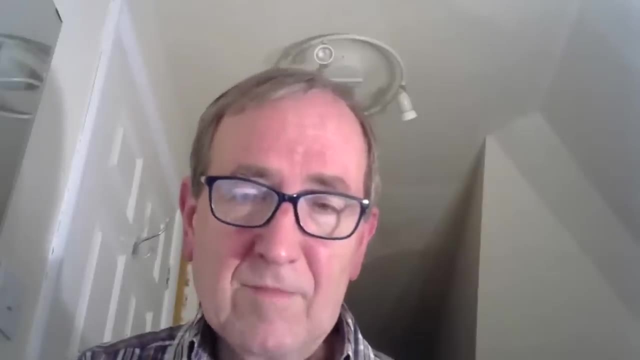 And of course the behavioral gap between us and Neanderthals is narrowed down. So it's very difficult to point to a single thing. I mean representational art representing animals and figures. For me, I don't see evidence for that. I don't see evidence for that in Neanderthals. We know now that early modern humans were apparently producing representational art over in Borneo and Sumatra as early as they were in Europe. So I think probably that kind of art was there. 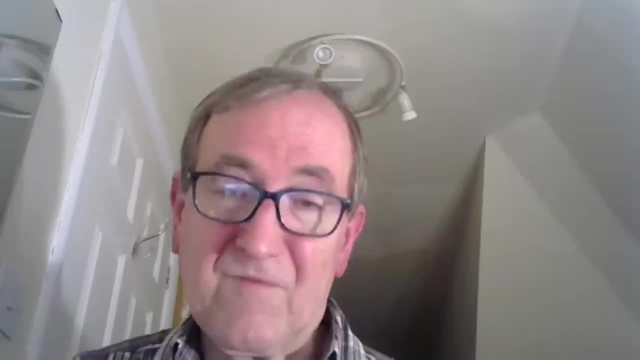 in the common ancestor of those populations. So it probably was in Africa before 60,000 years ago and it came out with modern humans and spread with them. So that may indicate something about the minds of modern humans compared with Neanderthals. 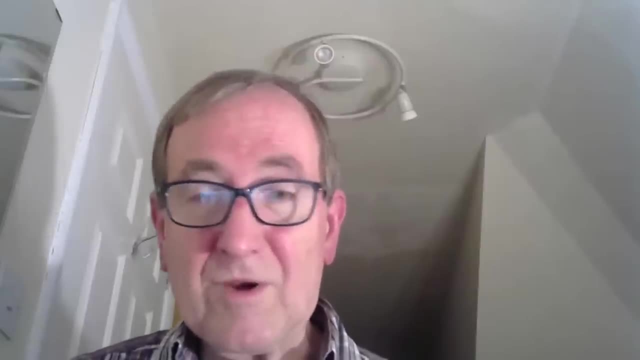 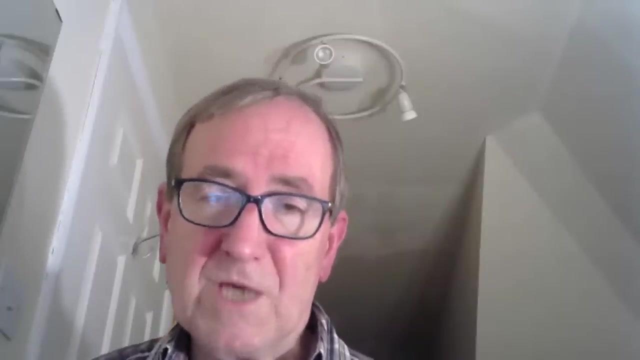 that kind of representational figurative art. But you know I'm not an archaeologist so I'm treading on dangerous territory here. And it may well be that it was an organizational thing for modern humans, And so it may be that, as we are able to map the sites, 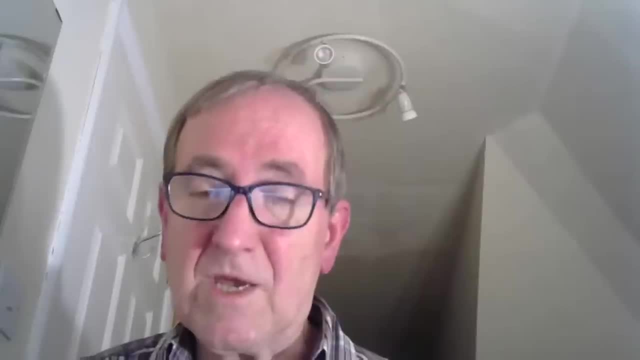 of early modern humans and compare them with Neanderthals and Denisophans in more detail, we may find that it was indeed networking, that larger group sizes allowing the greater storage of information and passing it on from one generation to the next. 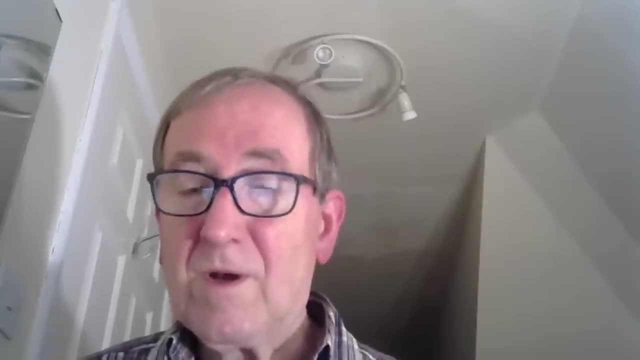 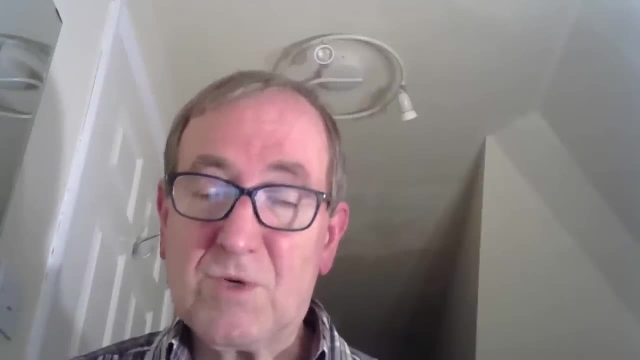 It may well be the survival of older people that are not only going to be grandparenting which will help the survival of infants, but it also means they've got a store of knowledge which covers a longer period of time, And that knowledge store can be important in the bad times. 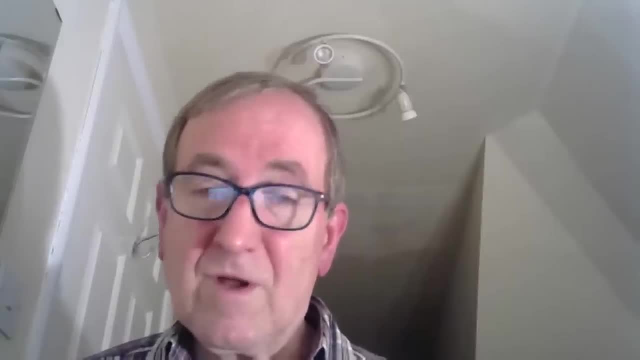 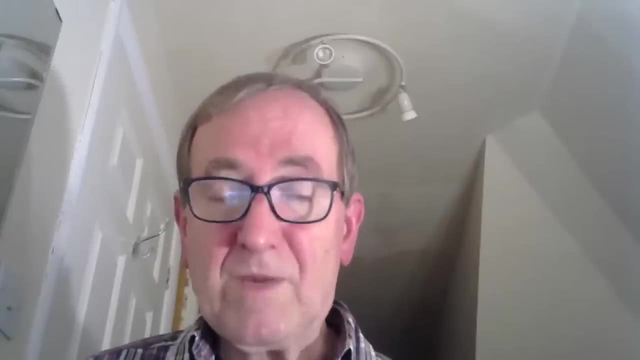 Older people may remember survival strategies that worked in the previous past, And also something that we see for Australian Aborigines, for example, is the older people are the ones who store the kinship knowledge, So those are the kinds of knowledge which they have in their heads. 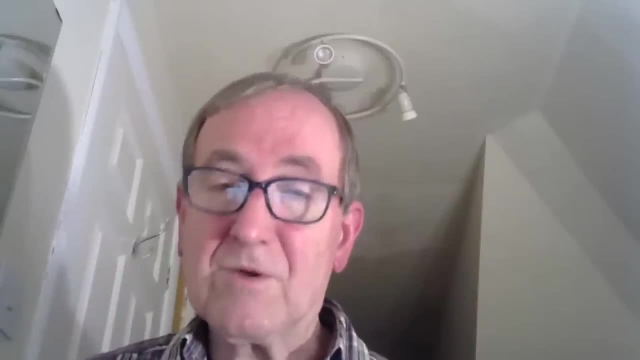 this fantastic map of relationships, of who's married who in the past, And that can be important in building alliances with other groups, in tracing back to a common ancestor. So I think even the survival of older people may have been important in the success of modern humans. 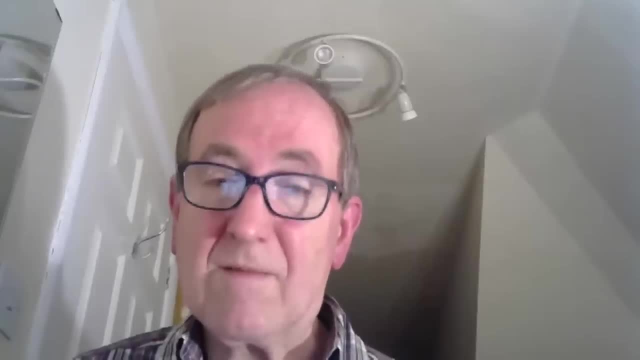 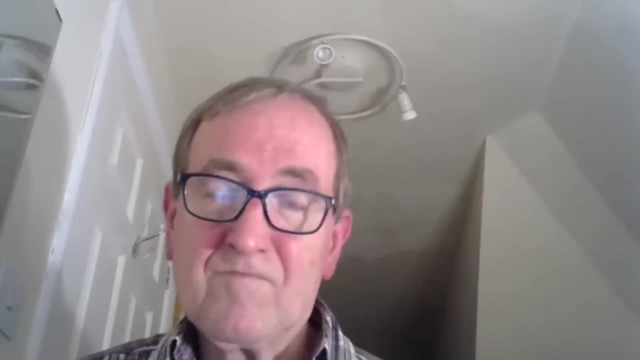 If less were surviving in Neanderthals and Denisophans, that may also have held them back a bit. And of course, you know, there could be some technology. Some people suggest that bows and arrows were key to the success of modern humans. 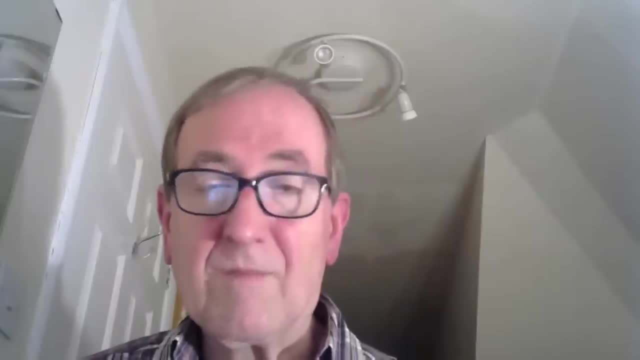 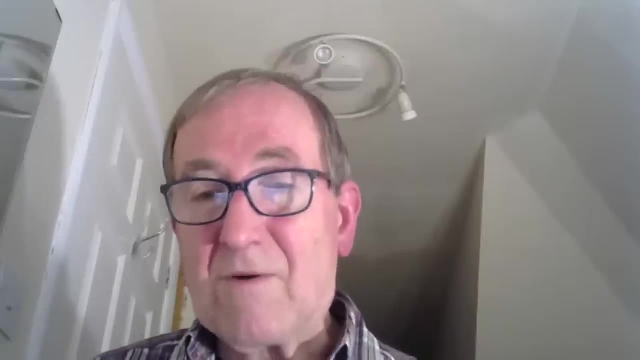 And there's some evidence from Africa that they appeared early. But for me, as you know, looking at the record- and you people would know this better than me- I think the presence of bows and arrows is very difficult to map against the spread. 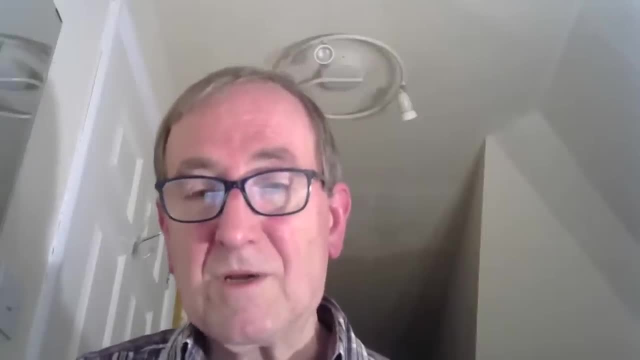 of modern humans across Europe and Asia. So, yeah, I can't point you at anything specific, but I think it's going to be a pattern in the end, built up from really good site data and also really the best dating that's possible in these populations. 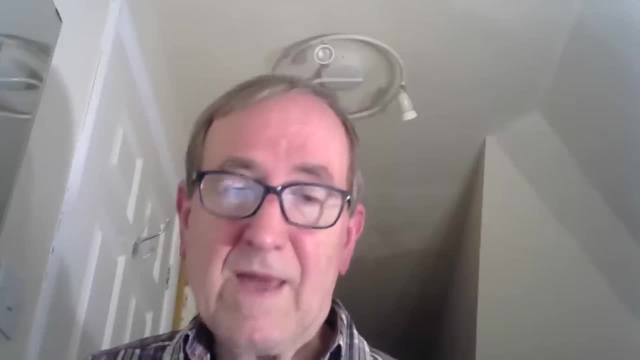 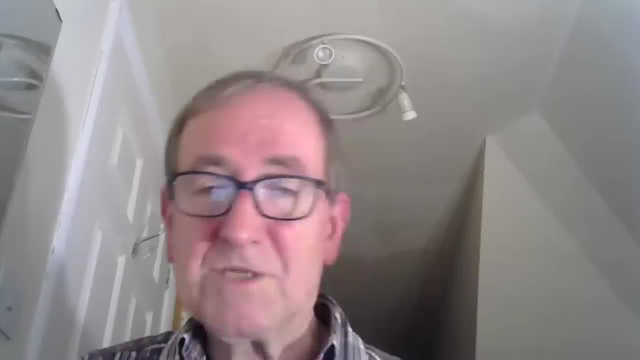 And something also I didn't talk about is how the interbreeding happened. That may also be a factor in the disappearance of these other populations And, of course, what we got evidence of is Neanderthals joining Homo sapiens groups, which is why we have Neanderthal DNA today. 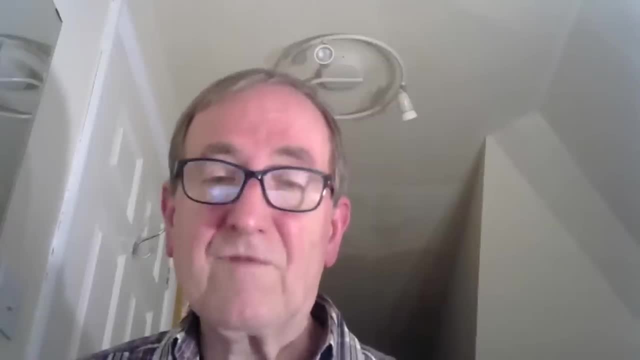 What there isn't much evidence of in the late Neanderthals so far is Homo sapiens DNA going into the Neanderthals. It may have been happening and we just haven't got it yet, But it seems to be. it seems to be much rarer in the late Neanderthals. 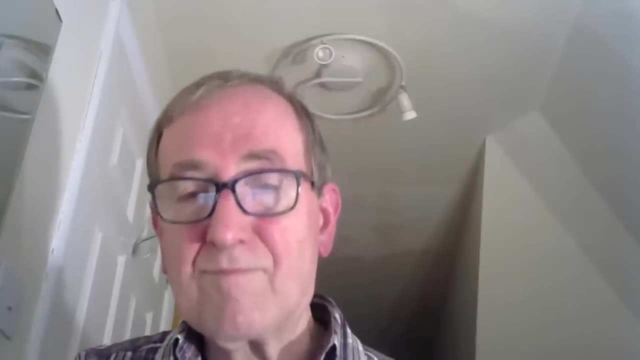 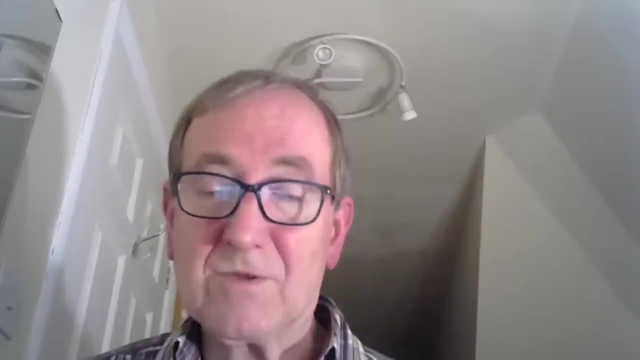 than in the reverse direction. So, of course, if you're taking out prime age, breeding individuals out of the Neanderthal gene pool and incorporating them into the Homo sapiens gene pool, that's going to be bad news for the Neanderthal gene pool. 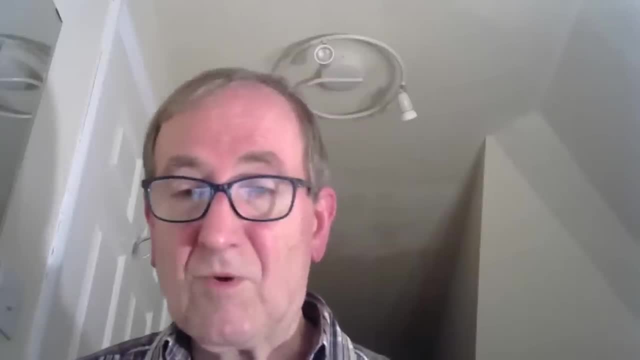 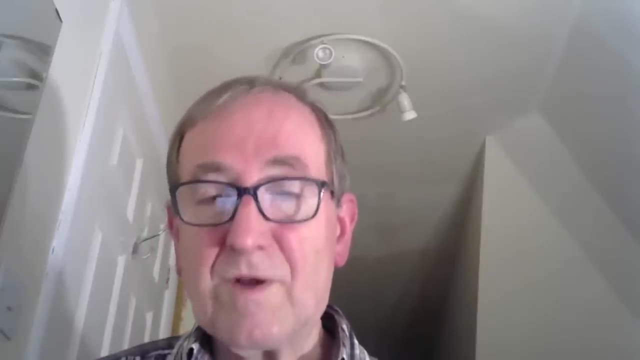 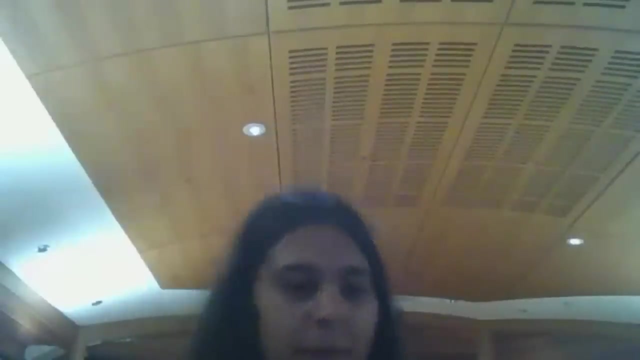 losing prime age individuals to these early modern human groups, So that even even that interbreeding, if it was mainly going one way, could be part of the story of why these other groups eventually faded away. Yeah, thanks so much. We have another question from Steve. 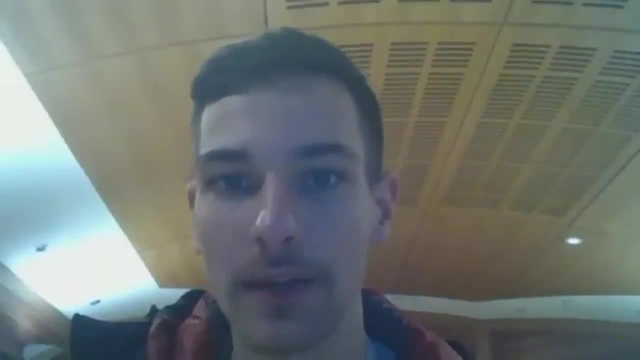 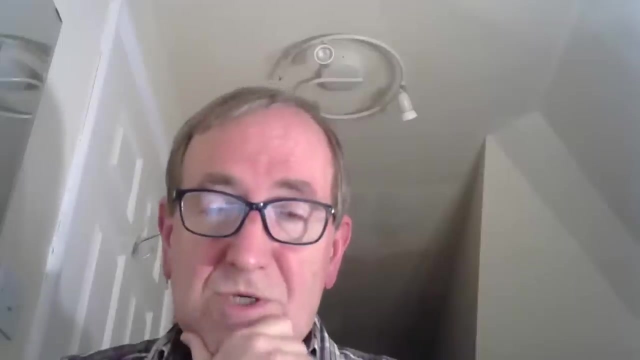 What do you predict to be the most exciting developments with regards to our understanding in human evolution over the next 10 years or so? Yeah, that's a good question. I think that the sediment DNA is going to be really important because you know, there are many parts of Europe and Asia. 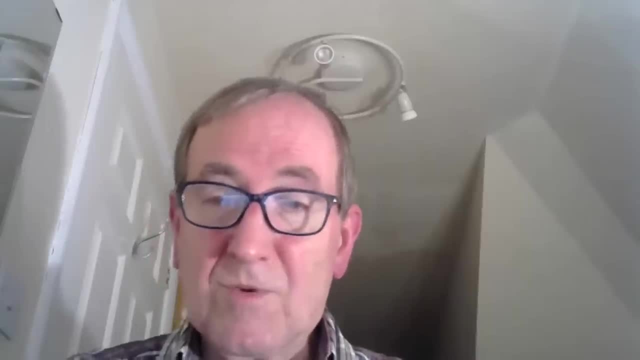 where we don't have a good fossil record, but there are cave sediments with stone tools. So if the preservation conditions are right, we will be able to map now the presence of Neanderthals, Denisovans and Homo sapiens in these sites. 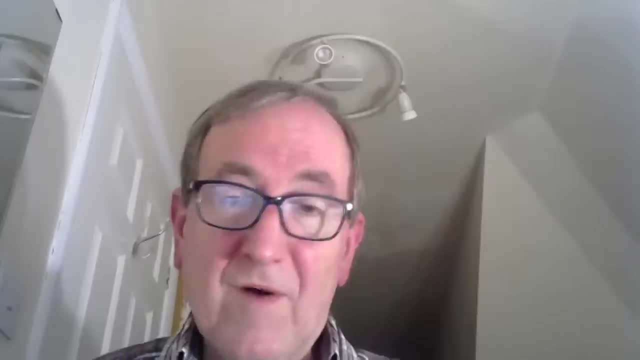 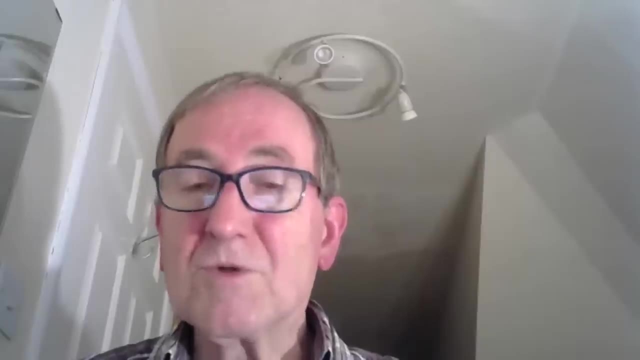 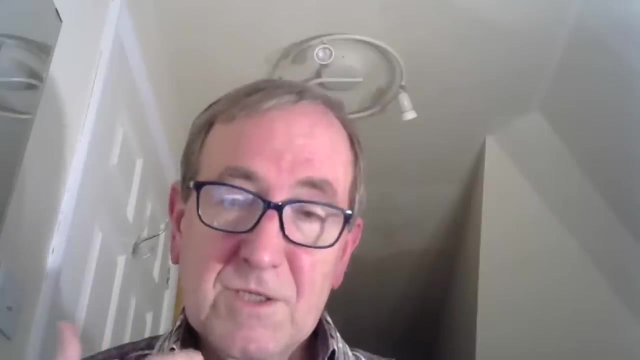 from DNA evidence, And we may even find other humans like the Denisovans that were there too. So I think the sediment DNA is going to revolutionise the way sites are dug archaeologically in this time period. If there's DNA preservation, then collecting for DNA samples. 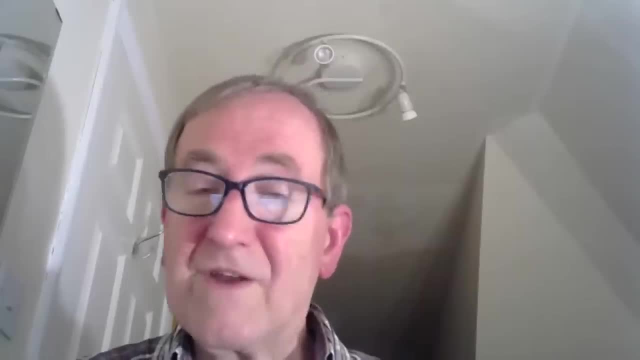 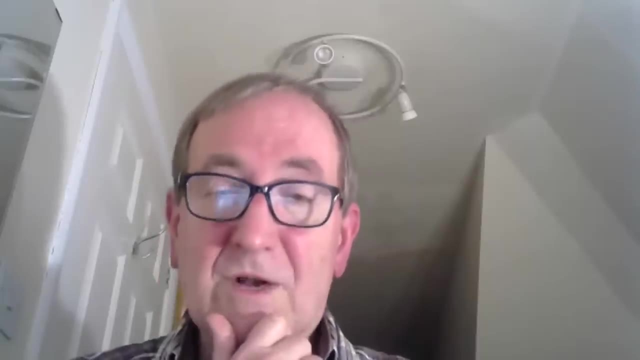 should be part of the excavation strategy from the very beginning now of any new site that is going to be excavated. And the good thing is that even in Africa, in high altitude sites, in deep cave sites, there might even be sediment DNA preservation there. 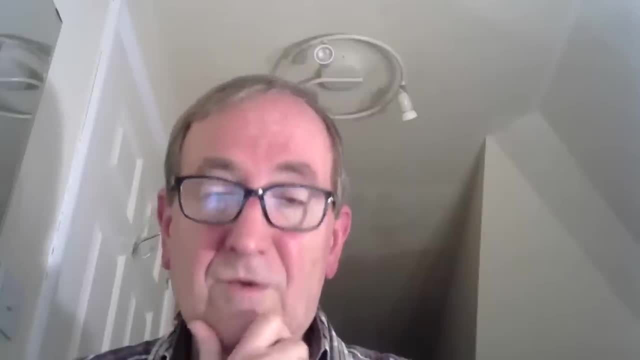 where you haven't got fossils. So I think that's a huge breakthrough and will be very important. On the genetic side, yeah, I think that studies that are going on to see what's the introgressed DNA, what comes across into modern humans. 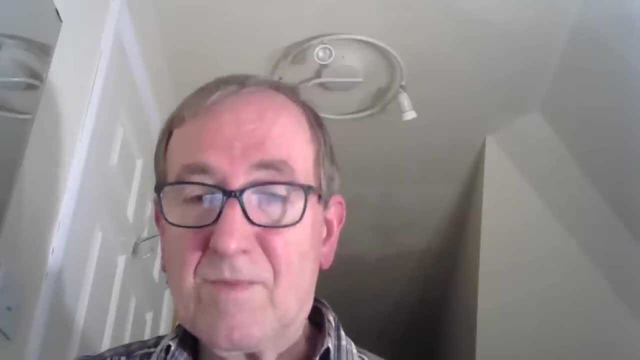 and what doesn't come across into modern humans. that will be important in really pinning down what bits of DNA are unique or largely unique to the Homo sapiens lineage and which are unique to the Neanderthal and Denisovan lineage, and then looking at at least to some extent.